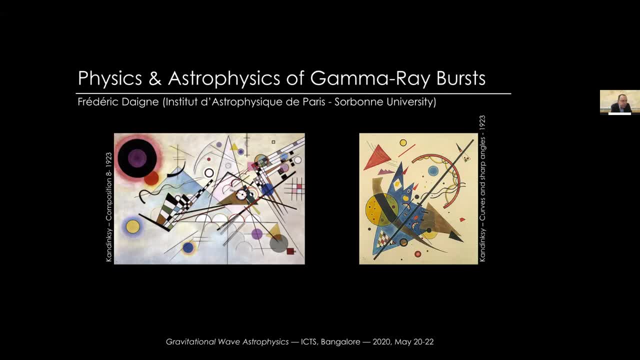 down your questions in the chat box publicly. At the end of the session we will have an interactive interaction session where you can raise hand and ask questions. Okay, over to Frederick. Okay, thank you very much. So let's start our third lecture. So here I have a slide. 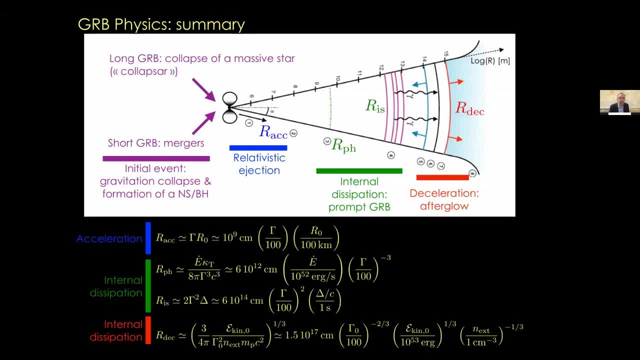 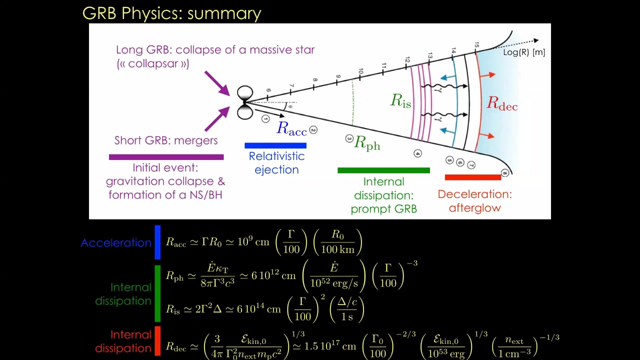 with a summary of the GRB scenario we developed together yesterday with the different steps. Here. this picture is focusing on the different phases in the history of relativistic ejecta. So there is on the left the initial event leading to the formation of relativistic ejecta And yesterday I. 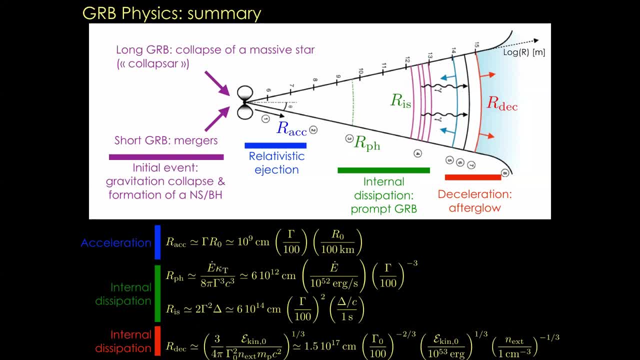 explained that there is an important produce, a photospheric produce, where the ejecta becomes transparent And all the elements are transparent. So the ejecta is transparent And all the elements are transparent. So the ejecta is transparent And all the elements are transparent. 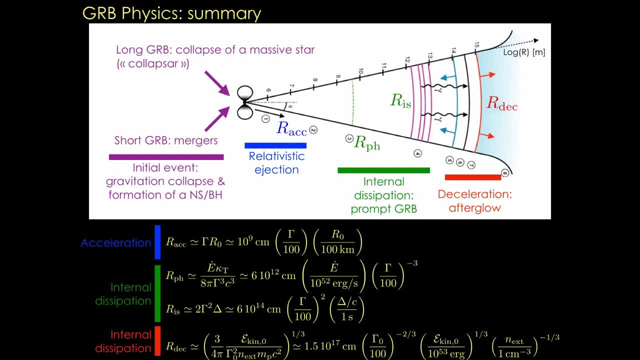 electromagnetic emission we will save is produced above or at this radius, and there are typically two episodes: one of internal dissipation, which is probably the main origin of the prompt emission, and then a deceleration phase, which is responsible for the afterglow. so today i will discuss a few. 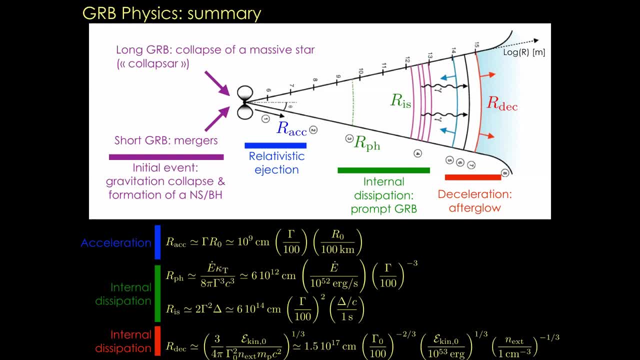 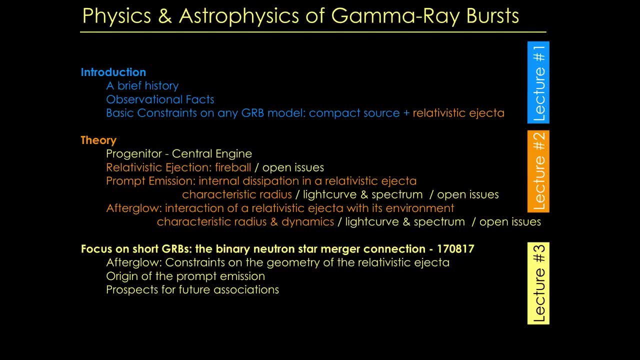 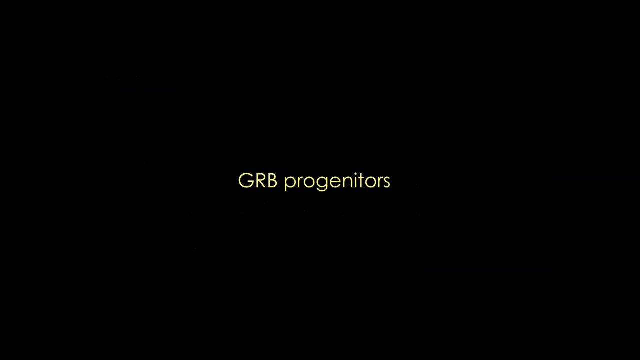 details about some aspects of this scenario. i won't be able to discuss everything, and then i will finish with the discussion of the recent 170817 event and the association of short camera burst with mergers. okay, so i will start with a few words about the question of progenitors. 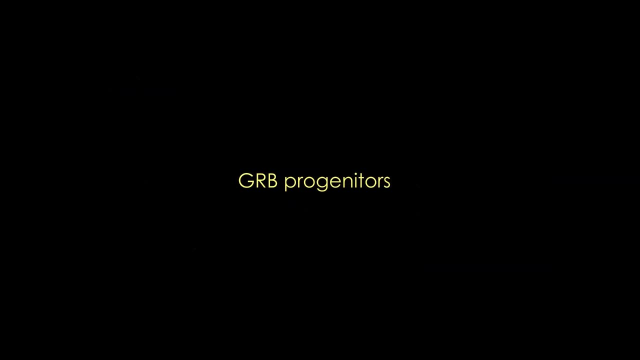 up to now i gave only very general arguments in favor of gravitational collapse and said that there were two channels: core collapse of the massive star or a merger of a binary system of two compact objects, for instance two neutron stars. now i can give a few more details to explain how we know that. 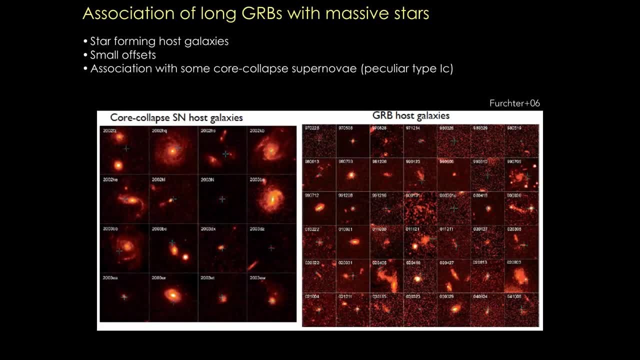 this association is probably correct. so for long gamma ray burst, the association of people of long gamma ray burst with massive stars is now really clear. to understand the arguments you have to know- very important- about stellar physics. probably everyone knows that. i will tell it. i would say: 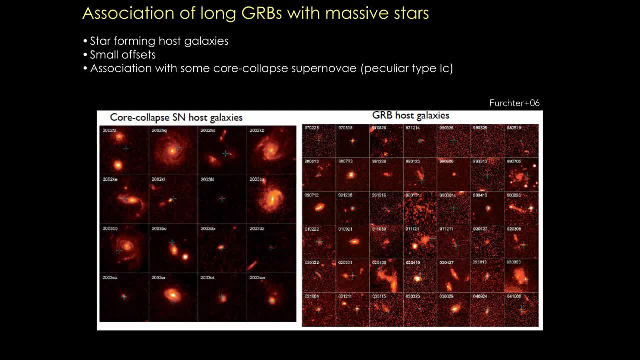 again, the lifetime of stars depends strongly on their mass and decreases rapidly with the mass, so massive stars have very short lifetimes compared to the typical time scale of evolution in a galaxy. that's why you can always consider that a massive star at the scale of a 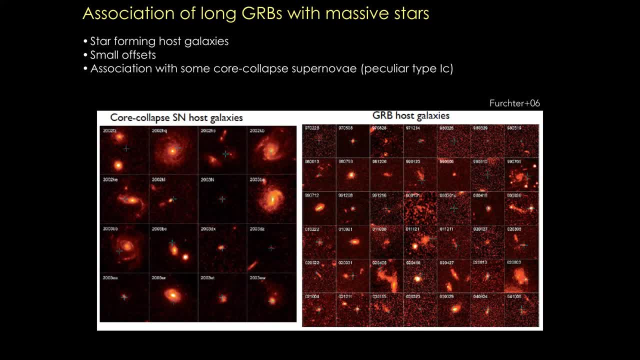 see, they are born somewhere and they immediately explode at the same place. and you, you always expect a massive star explosion to be associated with star formation, whereas for all other kind of progenitors, with longer delay compared to the star formation, you do not expect such a correlation. 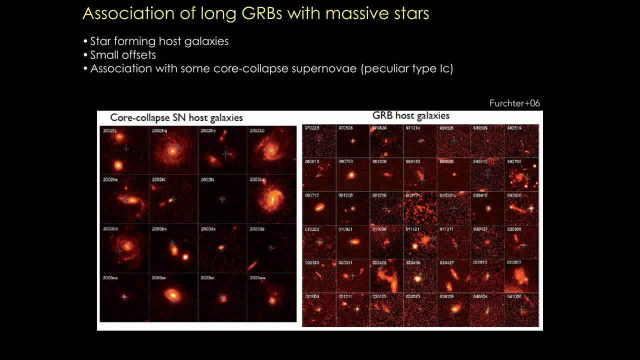 this key argument, for instance, has been used long time ago for the classification of supernovae. you probably know that one a supernovae can be observed in any kind of galaxy, whereas all other types of galaxy, of supernovae, sorry- are observed only in star forming galaxies. this is a clear 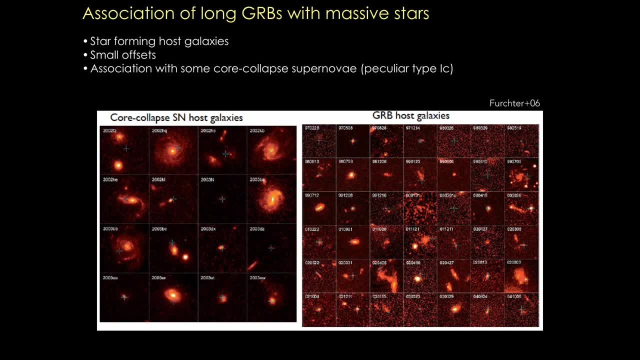 indication that all supernovae are associated to cross collapse, except one, a supernovae, which are associated to thermonuclear explosion of the world. you know that is the case. for example, the star formation is a supernovae that is in the middle of a wide dwarf and, as it takes a lot of time to produce a wide one, and then it takes a 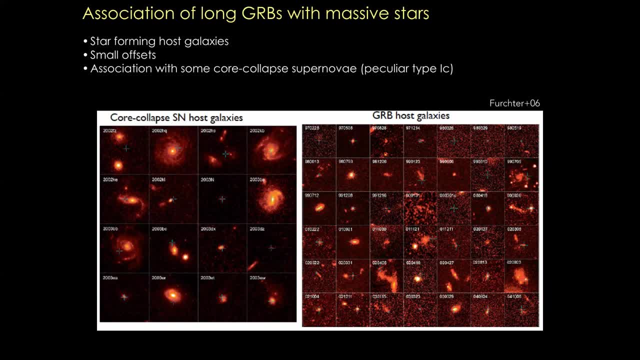 lot of time to reach for a wide wall, the condition for thermonuclear fusion. then you do not expect any correlation with star formation anymore. so here i show a sample of a of all galaxies of cocollapse supernovae and the sample of those galaxies of gamma rebursts. 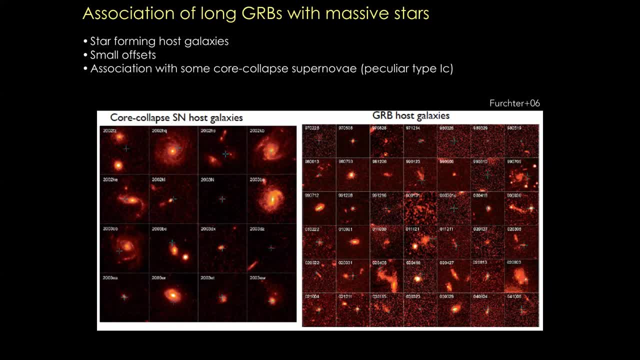 So the image of the galaxy has not the same quality as for a core collapse supernovae. Otherwise, you typically have the same kind of galaxies. You get star-forming galaxies, for instance. You see a few cases of very clear spiral galaxies. 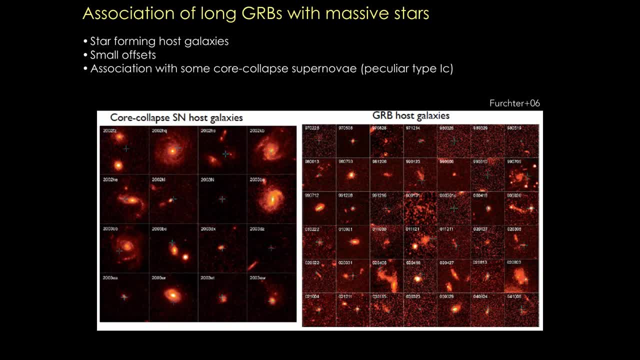 Another important aspect is the fact that the location of the afterglow is indicated with a cross, which usually is in the very central region. The offset of the afterglow compared to the brightest region of the galaxy where star formation occurs is usually very small. 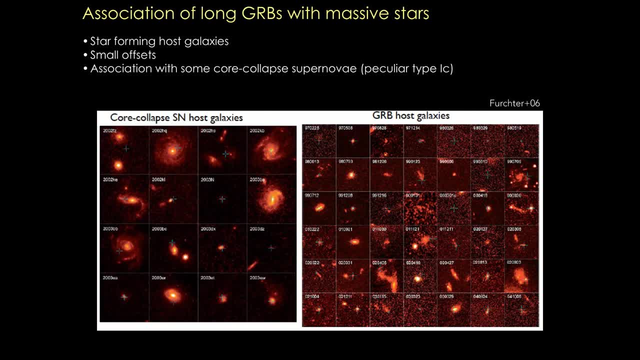 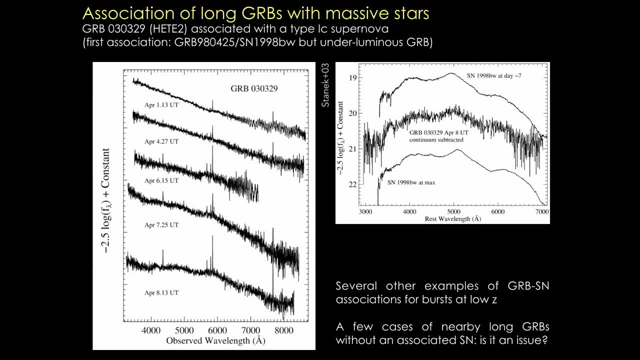 So here there is really a clear association of long gamma ray bursts with massive stars And in addition there are a few cases of gamma ray bursts associated to a supernova, a 1C supernova, a peculiar 1C supernova, I would say. 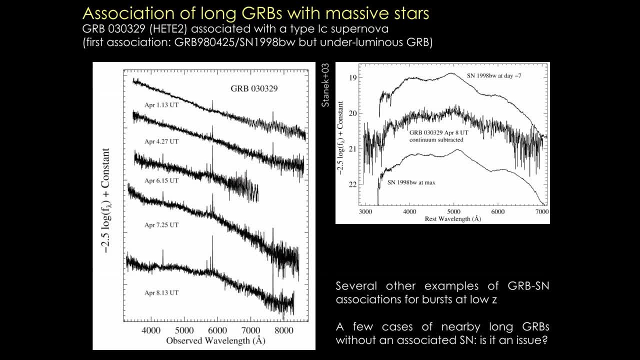 But 1C supernovae are associated to massive stars, It's not 1A supernovae. So here I show a famous example: the association of GRB 0303-29 with a supernova. So on the left you see the evolution of the spectrum. 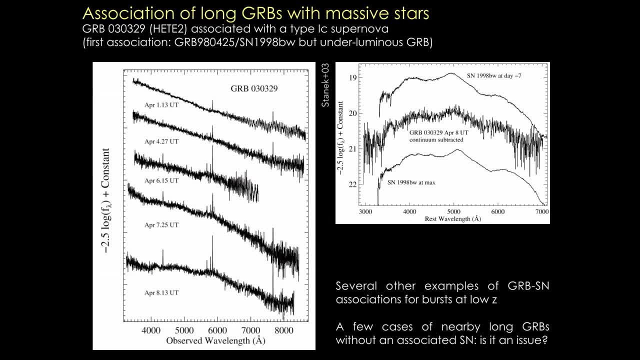 of the afterglow. You see that initially it's a clear power law, as expected for the afterglow, which is a non-sermal synchrotron radiation, And after, I would say maybe April 6 or maybe April 7,. 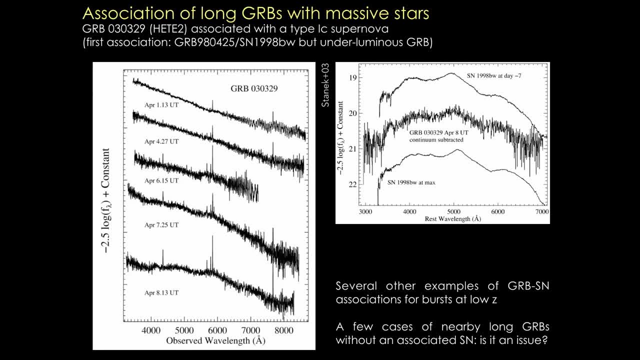 you see an additional component which appears, which has some spectral shape, And when you subtract the continuum, this is done on the right. So to do that, you take the spectrum at April 4, where it's clearly a pure power law. You smooth this power law. 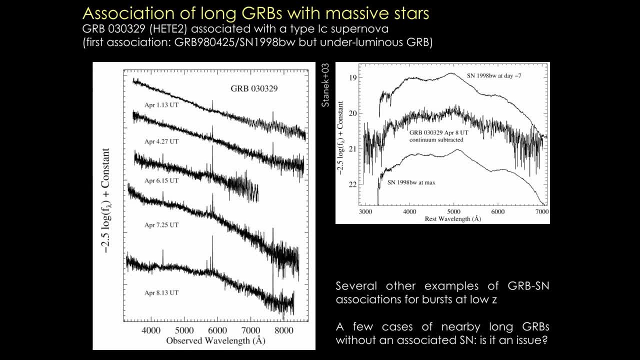 and then you find the right scaling to subtract it from April 8, and you get this spectrum with clear supernova features, especially broad absorption lines, Okay, So it's a good example. There are other ones. The first one was GRB 9804-25,. 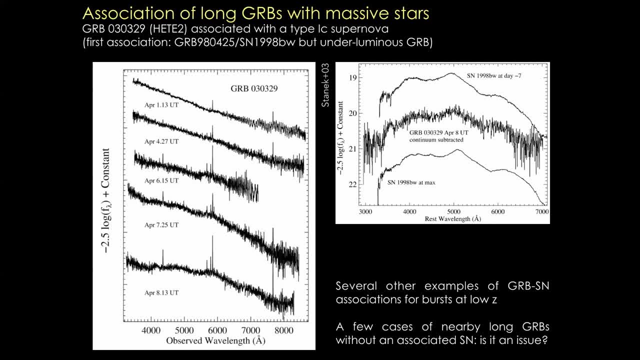 which is really nearby. It's at 40 megaparsec. It's a very interesting case, but it's not a spectrum. It's not a standard case because this GRB is undiluminous by, I think, four orders of magnitude. 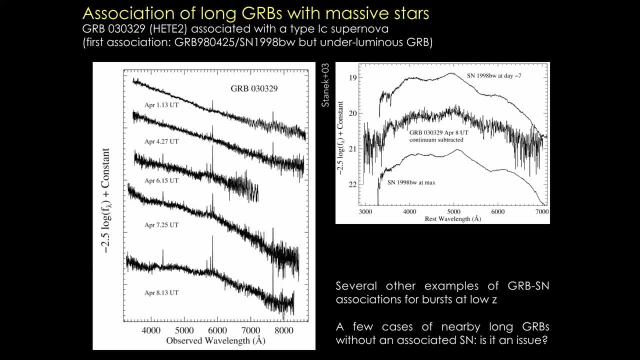 So it's not a standard gamma-ray burst And now there is a larger sample. There are other associations. It's always for nearby gamma-ray bursts, because to detect the supernova you need low distance, And I should mention that there are a few cases. 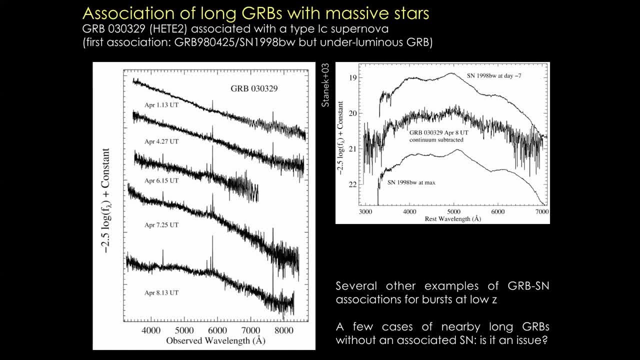 of nearby long gamma-ray bursts without an associated supernova. And then there is a debate to know if it is an issue or not, because, of course, if you do not understand fully the progenitors of gamma-ray bursts and the way the massive star will collapse. 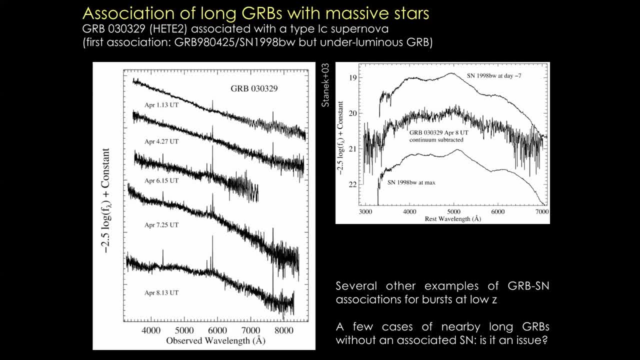 and produce a gamma-ray burst and possibly an associated supernova. it's not very clear to know if you should expect a one-per-one association. I would say that in the very early version of the Collapsar model, which is the model of the core collapse, 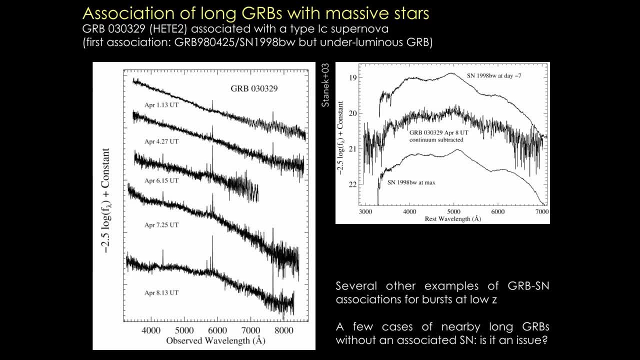 of a massive star to produce a gamma-ray burst. the very early version of this model was a failed supernova model, And it was not so clear that an associated supernova was expected. Okay, So I list here a few questions related to this question. 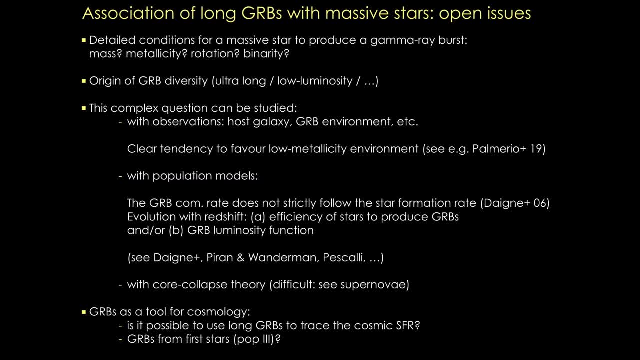 of long gamma-ray burst progenitors. The link with massive stars is clear, but now we have to understand the precise condition to produce a gamma-ray burst. We know that the rate of gamma-ray burst in a galaxy is much lower than the core collapse supernova rate. 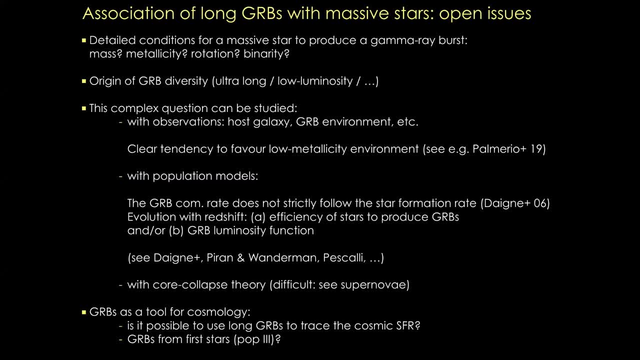 So it's only a small fraction of massive star which will produce gamma-ray burst. And what are the conditions? Is there a condition on the mass, on the metallicity, on the rotation, on the minority? It's not very clear. Another associated question: 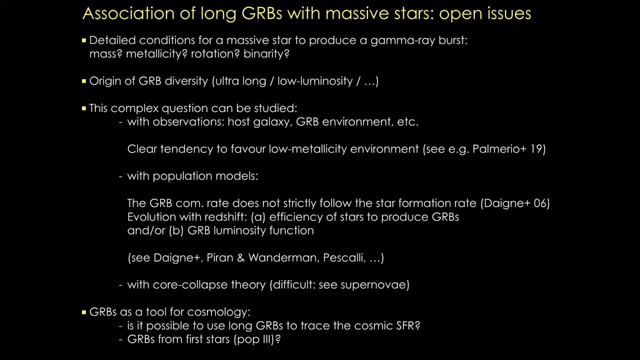 is the origin of the observed diversity of gamma-ray bursts. Why is there such diversity of luminosity, of duration, It's not very clear. It's probably related to the progenitor and the progenitor somehow will determine the energy reservoir to power the gamma-ray burst. 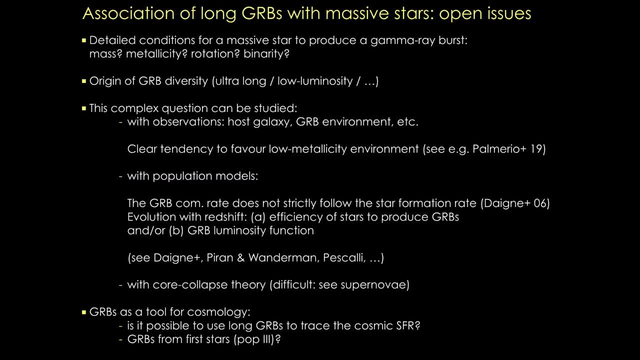 for instance, regarding the luminosity, But it's a very complex question. So to address this question, there are several ways. A lot of observational work, For instance. a lot of work is related to the host galaxy. I see that there is a question about short gamma-ray bursts. 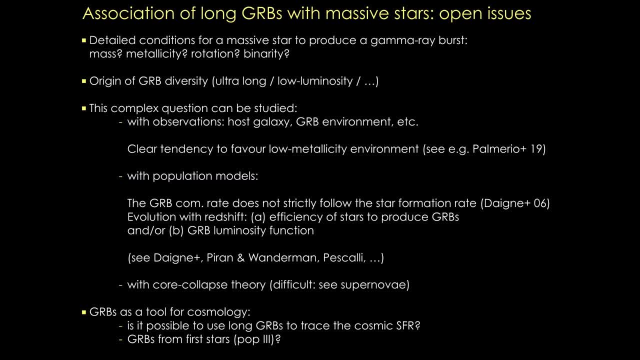 I will comment that in the next slide For the host galaxy, for instance for nearby bursts, you can try to determine the physical condition in this galaxy. If you are close enough, you can even try to probe the environment of the gamma-ray burst. 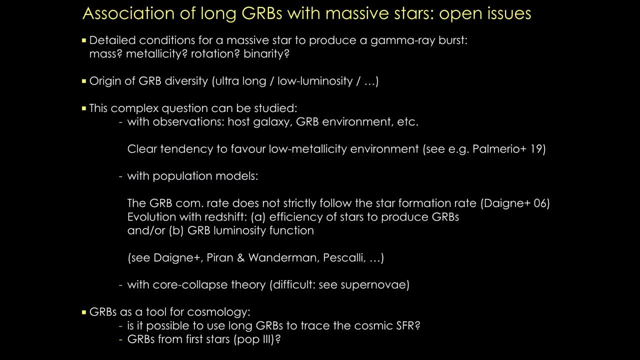 And these are indirect ways to understand the progenitors. For instance, these observations show a clear tendency for gamma-ray bursts to occur in low metallicity environments. It's very interesting, but it does not necessarily mean that the metallicity is the main criterion. 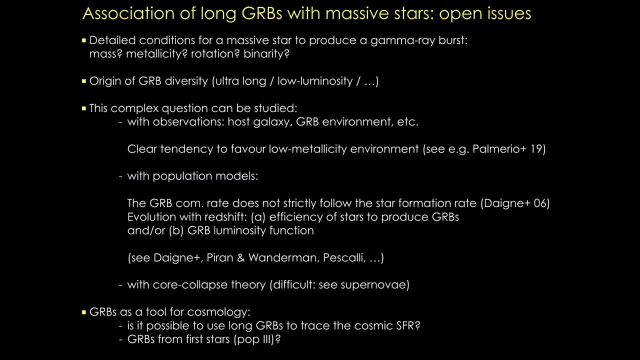 for producing a gamma-ray burst. Metallicity can have an indirect impact. For instance, metallicity has an impact on the star formation process and can have an impact on the fraction of massive stars or the fraction of binary systems, things like that. So it's difficult to. 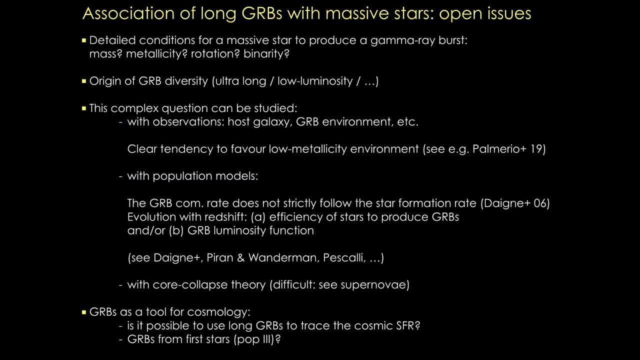 The correlation with low metallicity is clear, but it's difficult to deduce things about progenitors. You can also try to model the population of long gamma-ray bursts to understand, for instance, how the co-moving rate in the universe is evolving or how the luminosity function is evolving. 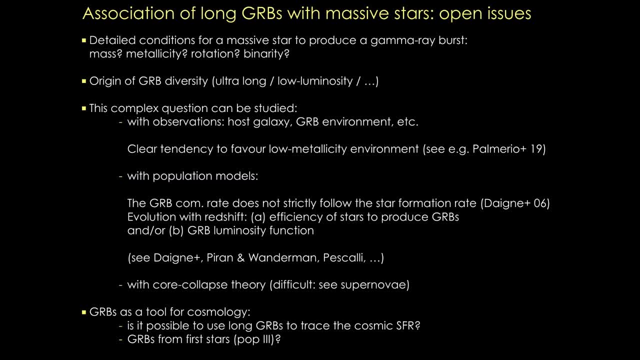 It's something that has been done by several groups. For instance, there are groups who were among the first to show that such studies clearly indicate that the co-moving rate of gamma-ray bursts is not strictly following the star formation rate. So it means that the fraction of massive stars 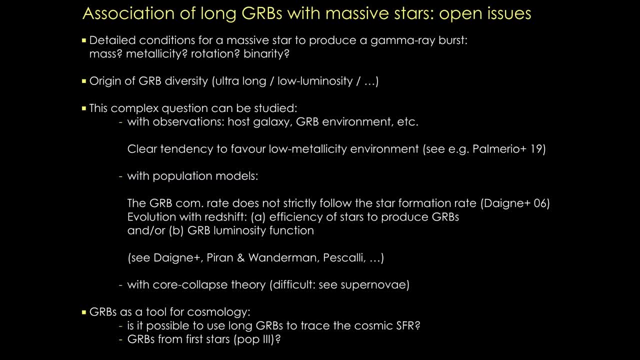 producing gamma-ray bursts is probably evolving, which is maybe compatible with the low metallicity correlation. And, of course, the main way to address the question is theory. but, as you know, the theory of core collapse is extremely complex. It's not very clear. 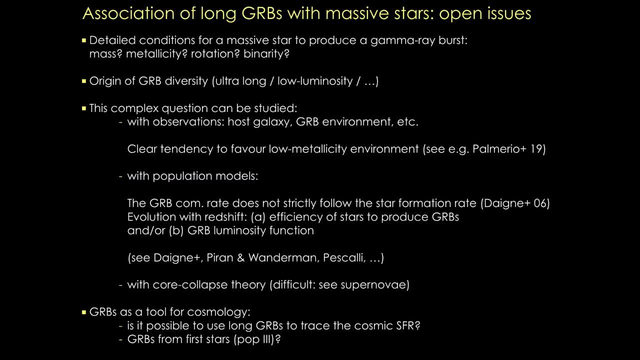 if we have fully understood the main channel, which is the standard type 2 supernova, Just for supernovae, there is a great diversity of supernovae with, for instance, superluminous supernovae, things like that. 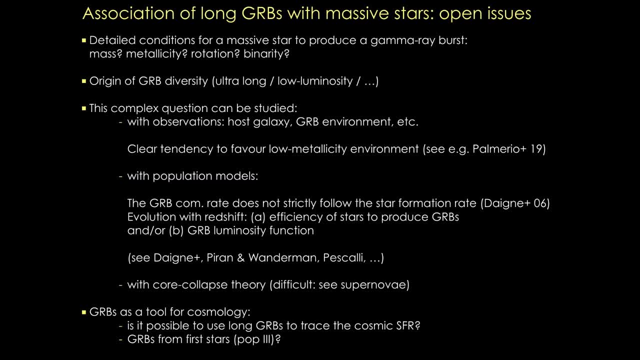 And there are a lot of debates to understand how the core collapse model has to be modified to reproduce this diversity, And gamma-ray bursts are an even more extreme case. so it's really a complex question And I should mention briefly that this question has the consequences. 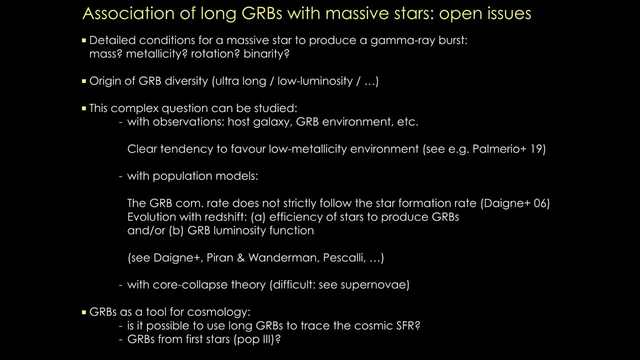 for the use of gamma-ray bursts for cosmology Because, for instance, if you want to use long gamma-ray bursts to trace the cosmic star formation rate at high rate shift, you have to understand precisely the progenitors to correct for a possible bias. 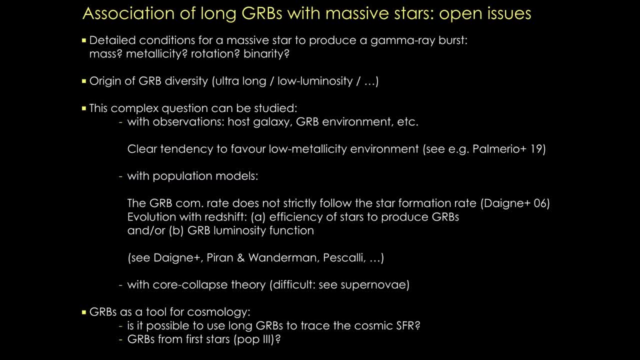 Another very interesting question is to know if the first population of stars was able to produce gamma-ray bursts and what would be their properties, because it may be a unique way to directly probe the explosions of the first stars. I mean, you can expect. 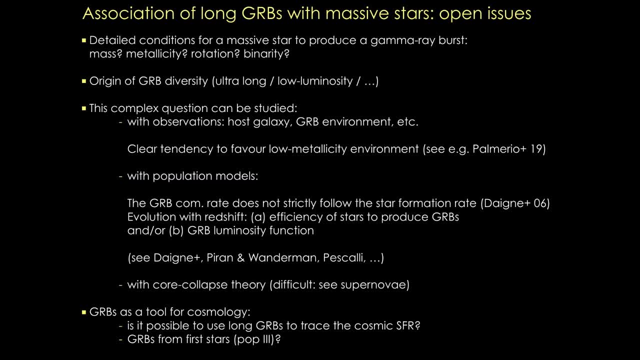 to probe the first star population, for instance, with a GWST observation of very distant galaxies. but for individual stars exploding, it's only gamma-ray bursts which can produce and can be used. Okay, So it was for long gamma-ray bursts. 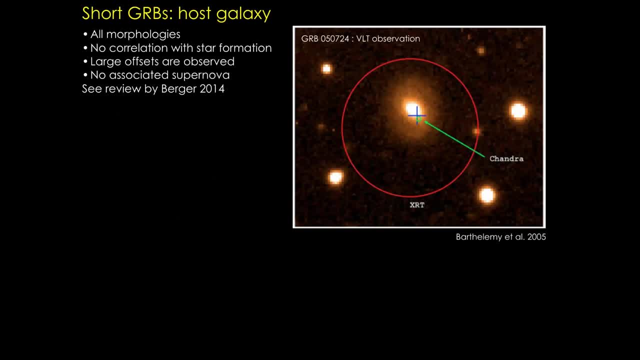 and now one word about short gamma-ray bursts. So for short gamma-ray bursts it's completely different. You can have host galaxies of any type- Some are star-forming, some are not star-forming, And you can also have large offsets. 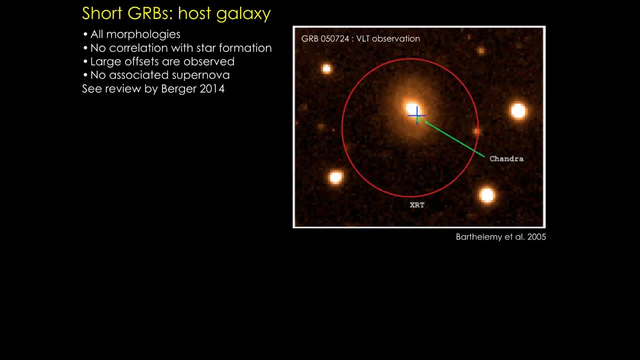 You see sometimes that the afterglow is located in the periphery of the galaxy or even sometimes outside the galaxy, which asks some questions about the reality of the association. You have to make some probability to know the risk of having a wrong association. 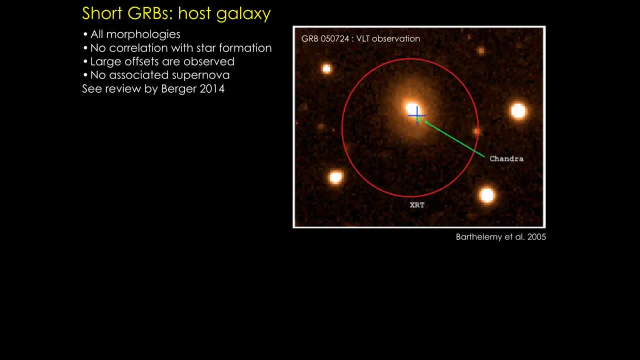 And there are no associated supernovae with short gamma-ray bursts. So for the question about short gamma-ray bursts associated with a massive star collapse, it's a good question, As I said in the first lecture, probably the distinction between short and long gamma-ray bursts. 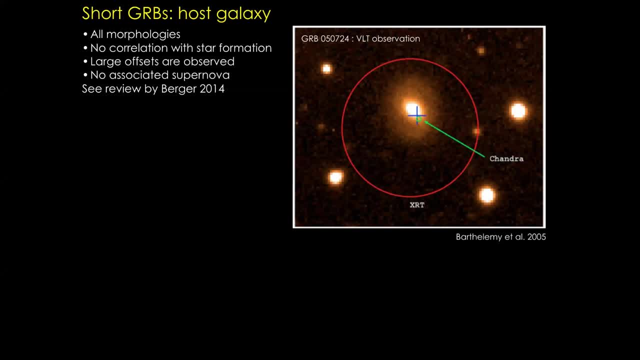 should not be done only on the duration, because there is some overlap at the frontier. So I would say that for the moment there is no clear association of a short gamma-ray burst with a core collapse, For instance, no association with a supernova. 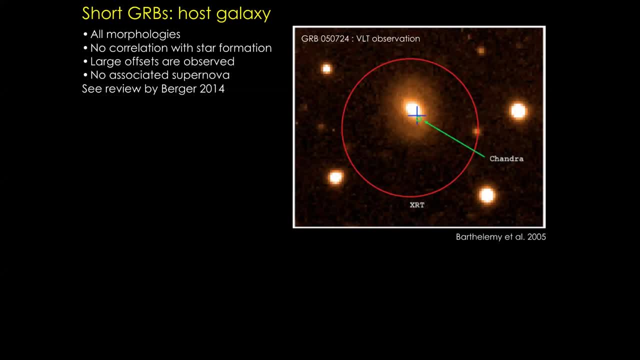 And if we were finding a short gamma-ray burst with an associated supernova, probably it would mean that we are in the tail of the long gamma-ray burst population and we are at the shortest end of this population. So if you are interested in this question, 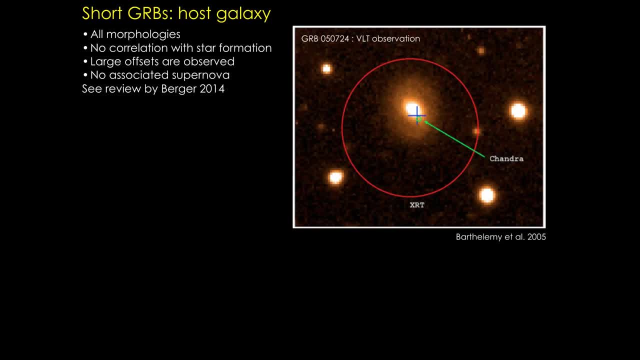 there is an excellent review by Berger listing all properties of this short gamma-ray burst of galaxies And notice that, as the signal is fainter, the fraction of short gamma-ray bursts with a measured afterglow and reshift is much shorter than for long gamma-ray bursts. 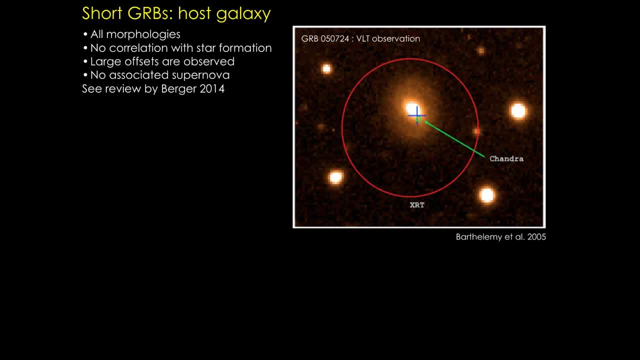 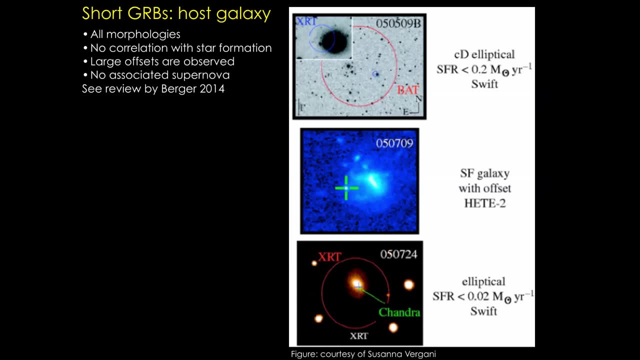 So the sample of host galaxies is not as large. Okay, So here I show another figure where you have three examples of host galaxies, of short gamma-ray bursts, And, for instance, the first one or the last one are elliptical galaxies where the star formation is very low. 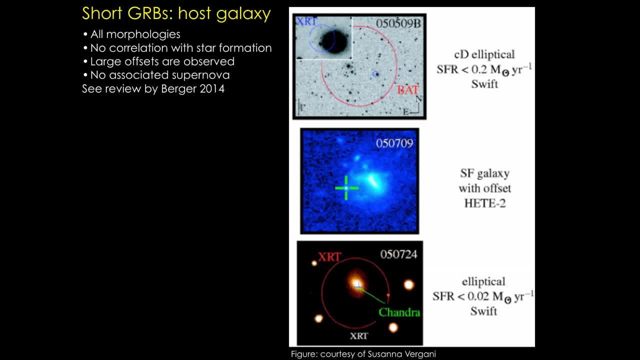 Whereas the second case is a star-forming galaxy, like the kind of galaxies you could expect for a long gamma-ray burst. But here there is a difference: The offset is quite large. You see that the afterglow is not located in the brightest region of the galaxy. 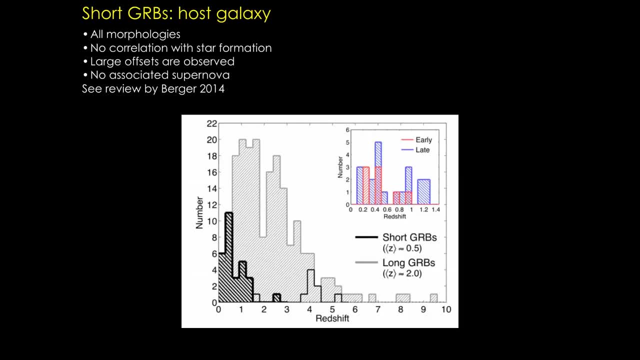 So there is a clear distinction. So another difference is the reshift distribution. On average, short gamma-ray bursts occur at a lower reshift, which is compatible with the idea of a longer delay between star formation and short gamma-ray burst. But you have to be very careful. 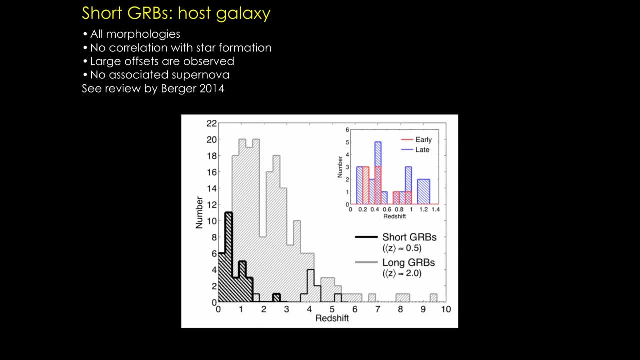 Such a diagram has a strong selection bias. So if you want to really test that you have to make a full population model where you're correct for the detection bias. So it's especially difficult to model the probability of measuring the reshift of a gamma-ray burst. 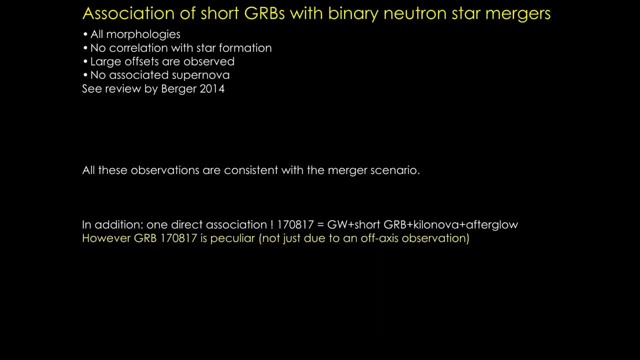 So this diagram has to be taken with caution. So all these facts are fully compatible with the merger scenario. I would like to have a direct association with gravitational waves to really prove that, Because gravitational waves will tell without any ambiguity that it's, for instance, 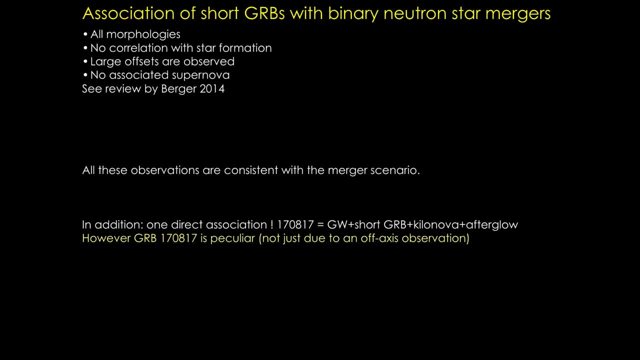 a binary neutron star merger. So we have one case with 170817.. So we could say, OK, now everything is proved. But as I will show at the end of this lecture, the gamma-ray burst associated with 170817 is not standard. 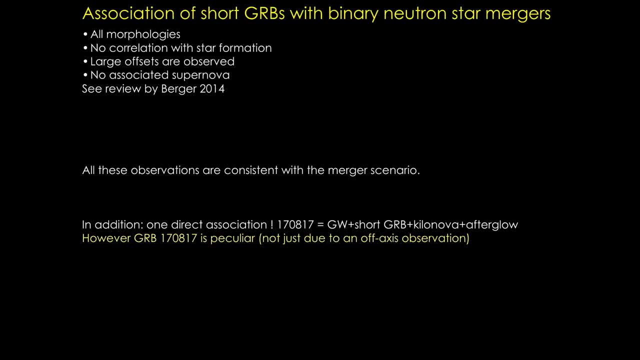 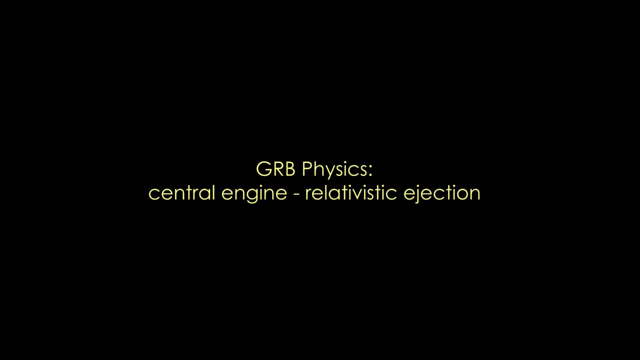 There are two more cases to completely prove this association. OK, so I don't know if there are other questions about this question of progenitors. I'm sorry, I won't give much more details. I would like now to discuss the question of. 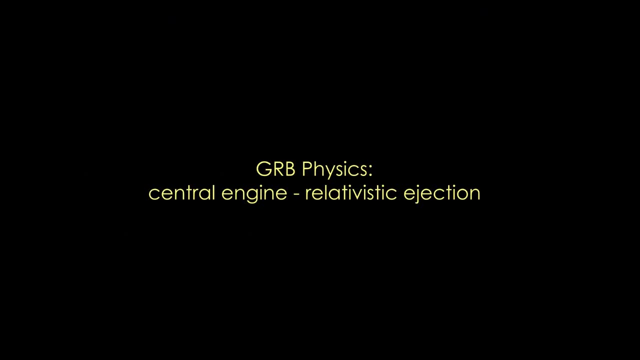 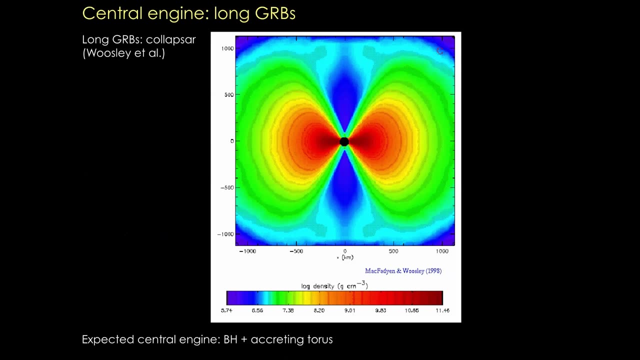 the central engine and the relativistic ejection. OK, so for long gamma-ray bursts, we associate them and it's now clearly proved. as I just said, we associate them with the core collapse of a massive star. So this is the so-called 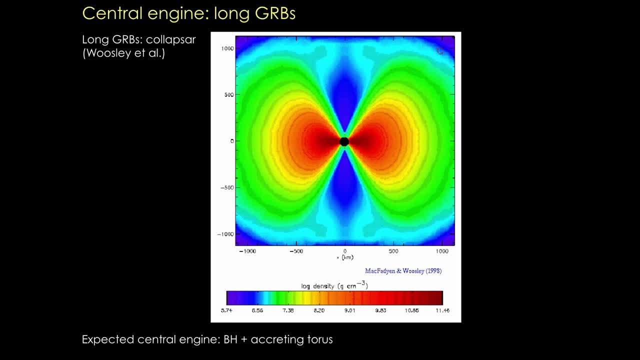 Collapsar model, which was developed by a different person but with a very significant contribution of Housley. And so here you have an illustration leading to the formation of a black hole surrounded by a thick accretion disk. we could say: 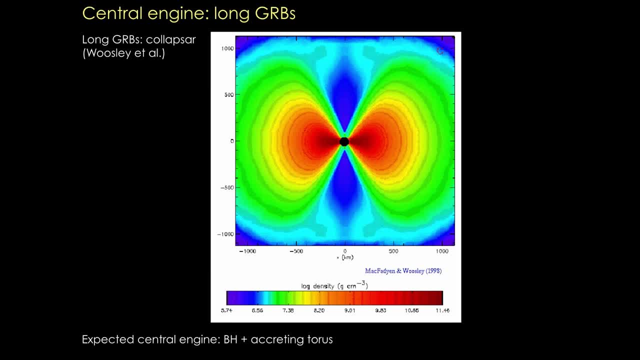 a thick torus. It is not a thin accretion disk like in many other astrophysical sources, because here the material is extremely hot and you cannot have a thin disk. In fact you have an accretion mass flux which is above 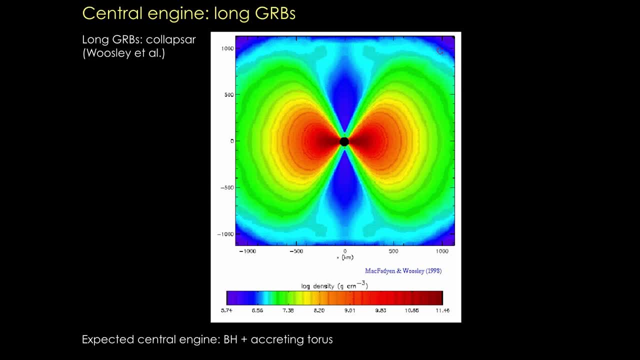 the ending time limit, So your disk becomes very thick. Probably the lifetime of the engine is related to the mass of this torus and to the mass flux, But the link is not very well done And then you could expect some diversity depending on the mass. 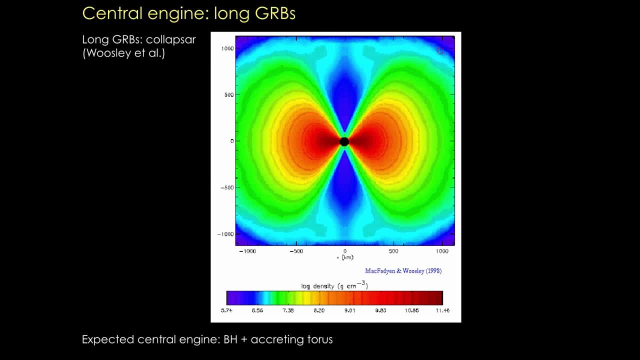 of the projector. You could have different mass for the disk and for the black hole and for the envelope which can still feel the disk when it's collapsing. So you can expect some diversity but then many questions how such a system is producing a relatively thick jet. 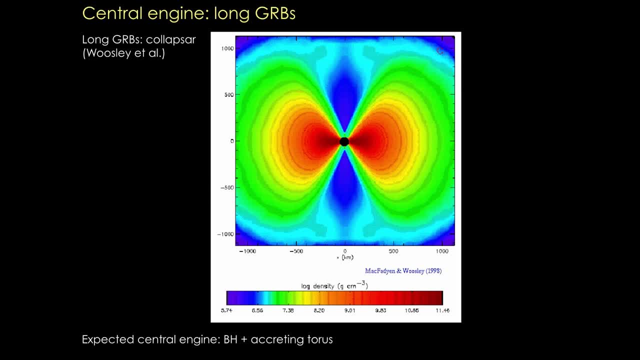 and how the jet is moving. So I'm not going to go into detail on the project today. but there are some groups investigating the possibility that in some core collapse the central object is not a black hole but highly magnetized neutron star or magnetar. 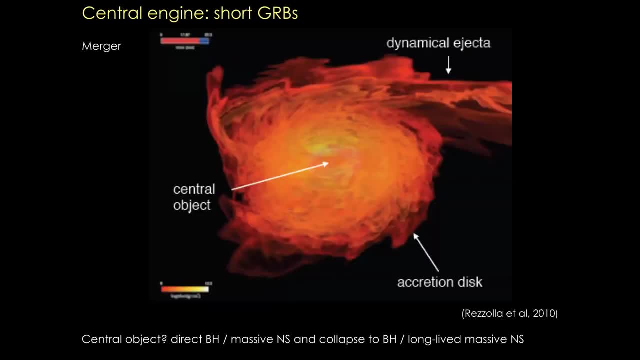 And so in this case the physics of the Ejection would be a little different. Here I show an example of the progenitor expected for short gamma ray bursts. So the central region looks like very much with the previous one. You form a compact object. 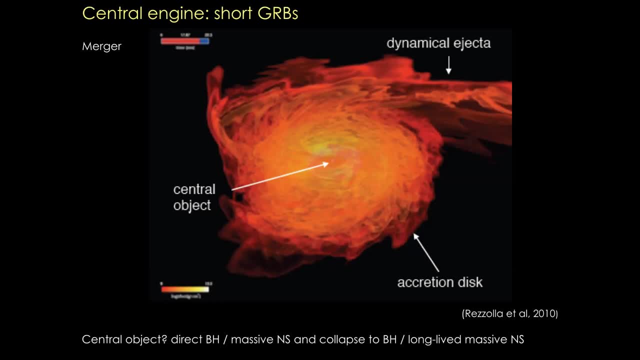 and it's surrounded by a thick accretion disk. But here the disk has a much lower mass than in the previous case, which could be the main reason for these events, for short gamma ray bursts and not long gamma ray bursts. On the simulation you see also the dynamical ejecta. 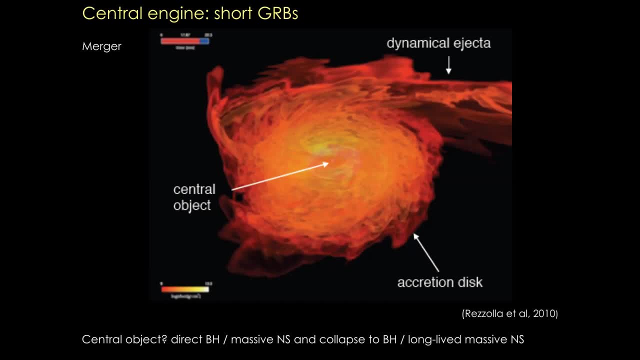 which is related to the tidal interaction during the merger. This dynamical ejecta is probably responsible for the kilonova, but there are some discussions about the possibility of this material to partially fall back on the central source, and it could be one way or another. 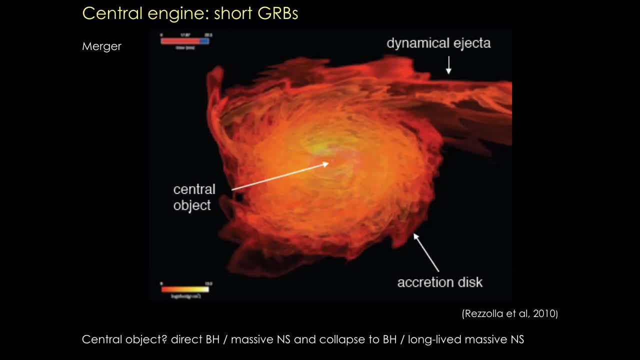 A very important question in this system is the nature of the central object. Depending on the mass of the two neutron stars and depending on the equation of state of ultra-dense matter, you can either expect a direct collapse to a black hole or first the formation. 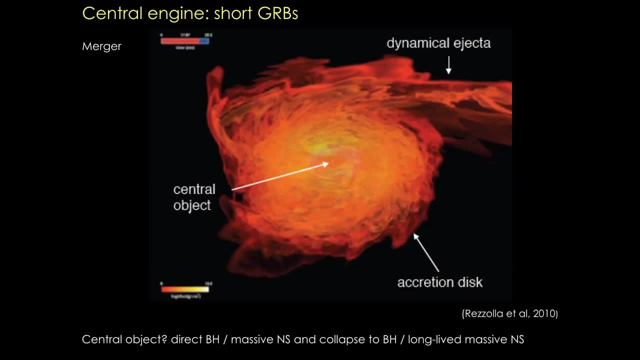 of a very massive star very close to the maximum mass in a dynamical time scale, the neutron star will collapse in a black hole, Or you can even form a stable, long-lived massive neutron star. It's not very clear. it's the same gamma ray, burst physics. 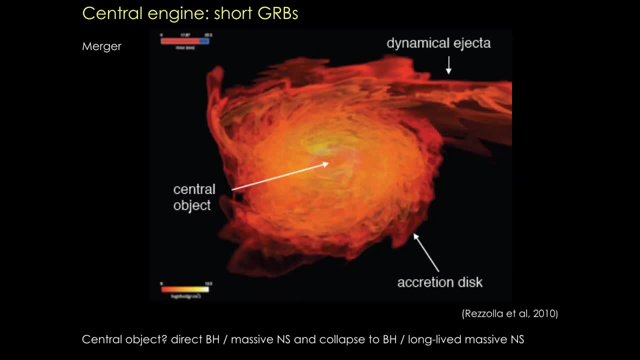 can apply in all these possibilities, and so it would be very interesting to have a clear signature of that from gravitational waves. Unfortunately, in the 170817 which is measured is only for the inspiral phase. we do not have a post-merger signal, which would be a direct 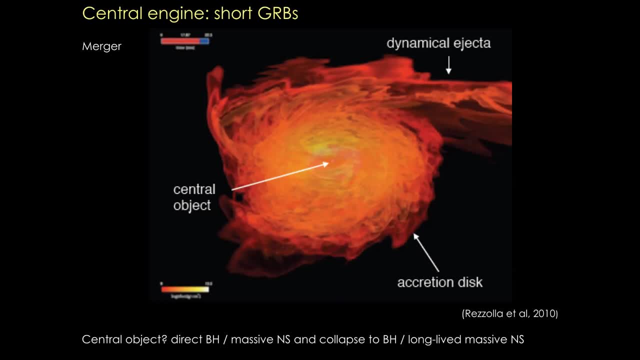 a direct signal for a direct signature for this central object. So maybe we will have to wait for improved detectors or the next generation of detectors to have the final answer. There are a lot of possibilities to have indirect information for the mass of the kilonova ejecta. 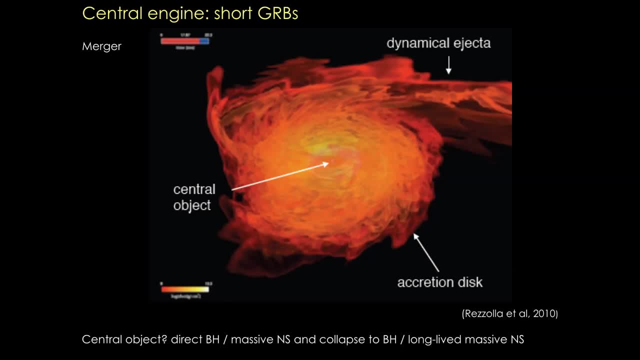 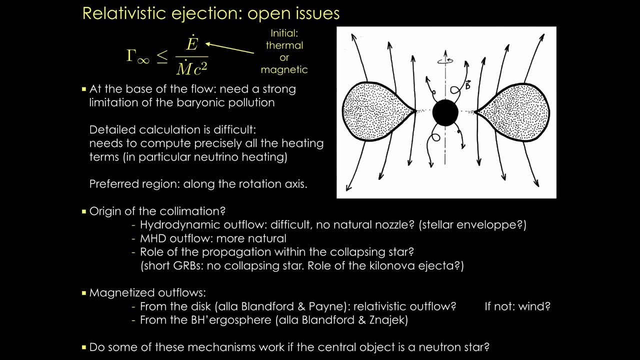 but it's less direct. A gravitational wave would give a direct signature. So let's focus on the most standard case, where you form a black hole surrounded by a thick disk. then you have to produce a relativistic ejecta. So the idea is that 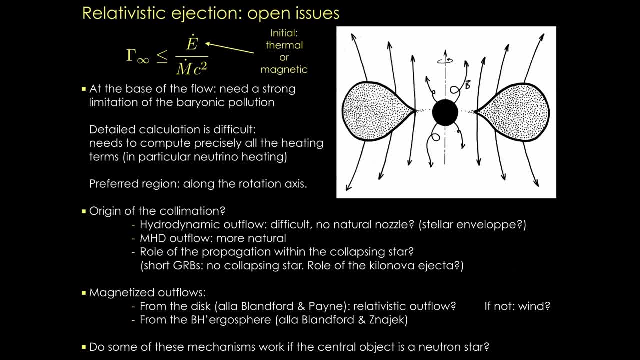 close to the source, you will put some energy, which probably is either 0 or 0. And this energy is ejected in an outflow with a certain mass. And if you want to become relativistic, a very basic condition is that you should have a very low bionic pollution. 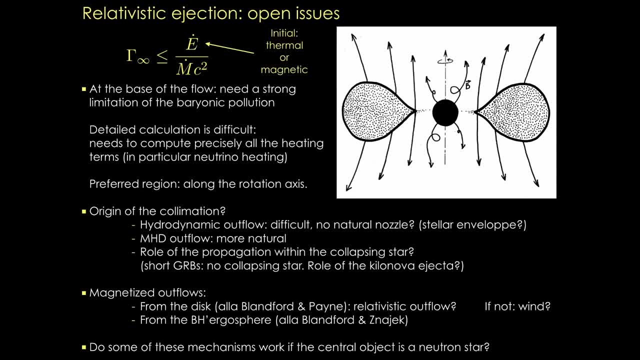 meaning that the ratio of the energy over mc2 should be very high. And then there is a second condition: to reach a high Lorentz factor, you need to convert most of the injected energy into kinetic energy. If you convert 100% of your initial energy, 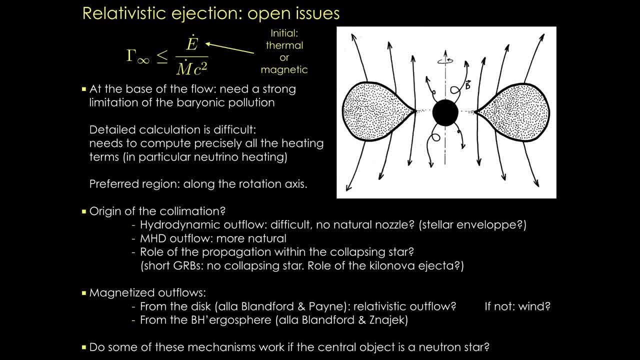 then the final Lorentz factor will be just given by the ratio e over mc2.. If the conversion is not efficient, it can be only lower than that. So there is a question about electromagnetic radiation from the accretion disk around the post-merger product. 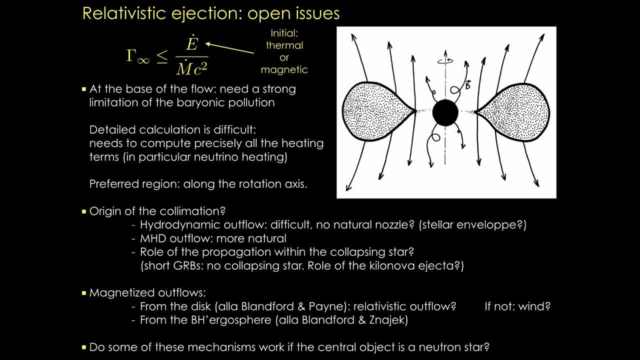 but in fact we do not detect this emission and the source is much too far. So the electromagnetic radiation we received is only associated with ejecta, either the kilonova ejecta or the relativistic ejecta responsible for the gamma reverse and the afterglow. 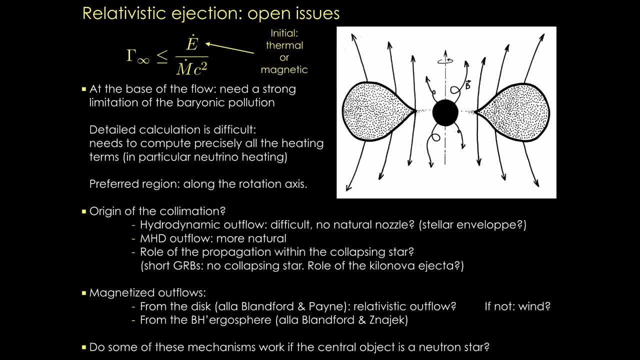 It's not like in an X-ray binary. for instance, You cannot observe an X-ray binary at 1 GPa or even 40 MPa. We do not receive direct light from the accretion disk And, in addition, as I said, we are well above. 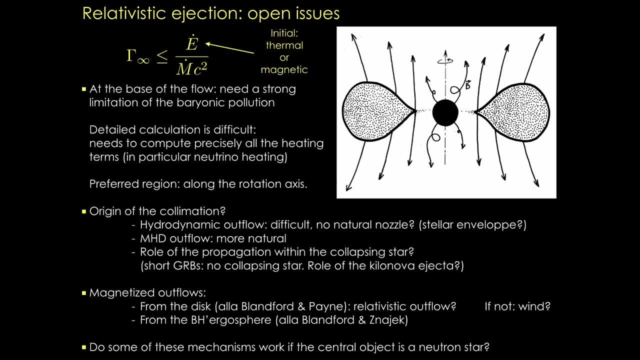 the dicton limit. So it's a good idea, but it's not working. Gravitational wave can help, neutrino could help, but not electromagnetic radiation. The idea is that now a lot of groups, or several groups, are developing very detailed simulations of such systems. 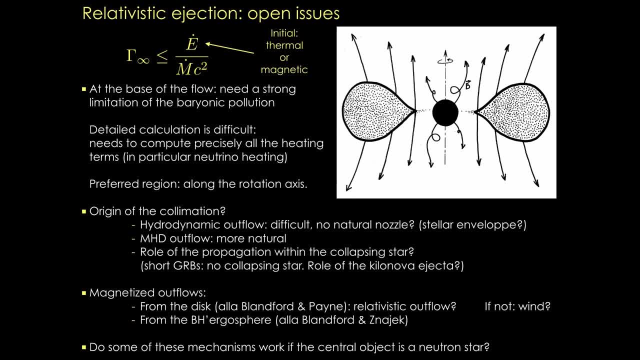 with, for instance, an MHD simulation in GR. so it's very sophisticated simulations, but the question of the bionic pollution remains very difficult to address because, to really address it correctly, you would in addition, in this simulation add a very detailed and precise calculation of all the heating processes. 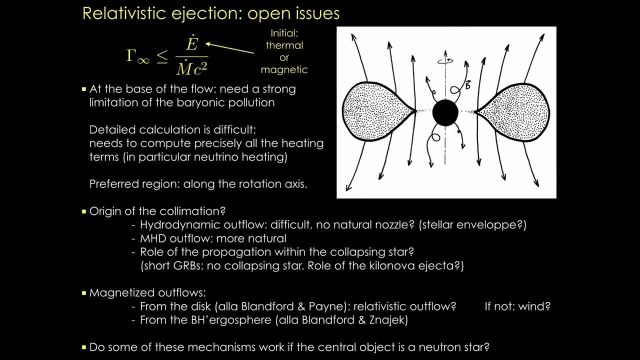 because the idea is that if your region is magnetized outside the disk, matter is forced to follow the magnetic field lines, and the question of how much matter will escape the disk and start to follow the lines is strongly related to the heating. If you heat a lot, the matter. 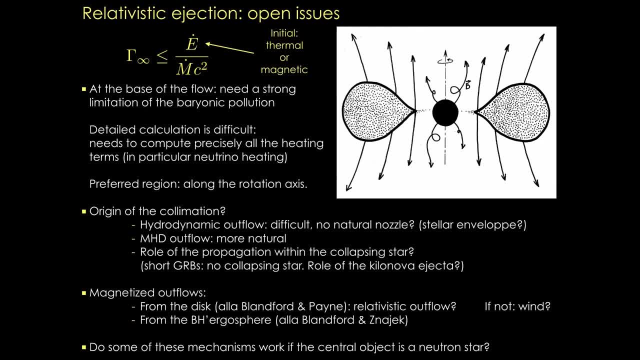 let's say in the corona of the disk. then a lot of matter will start to follow the field lines and you won't reach a high Lorentz factor. so you have to limit the heating And the heating is very difficult to compute because the temperature of the disk 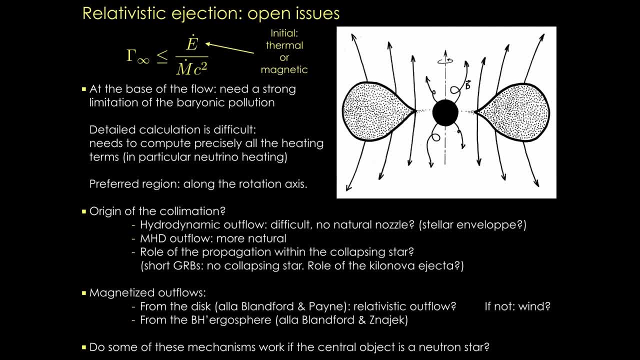 is very high, and the main mode of cooling for the disk is neutrino radiation, and so you have to compute precisely the neutrino emission and then the deposit of energy by neutrinos in matter, and one important process, for instance, is neutrino anti-neutrino annihilation. 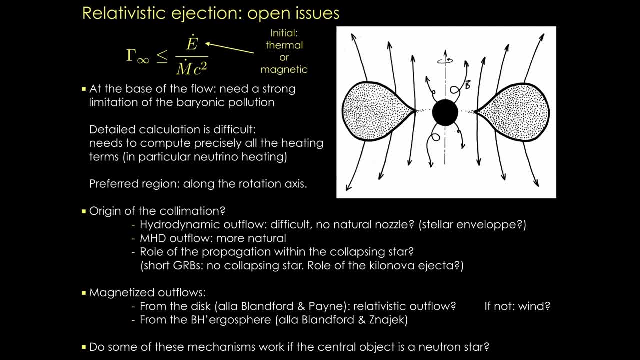 which is very complex to compute. you have just to compute the neutrino emission- it's typically an integral over the whole volume of the disk- and to compute a neutrino anti-neutrino rate. it's a product. so it's six integrals because you have to integrate twice. 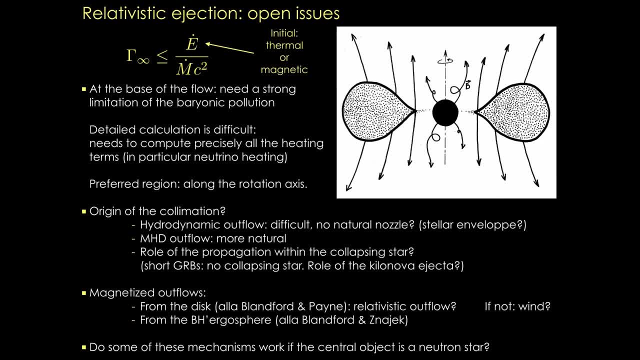 on the volume and in addition, if you are in GR you have to really compute the geodesics of the neutrinos which are not propagating in straight lines in this region. So it's a novel problem and there are some: either some simplified numerical schemes or some. 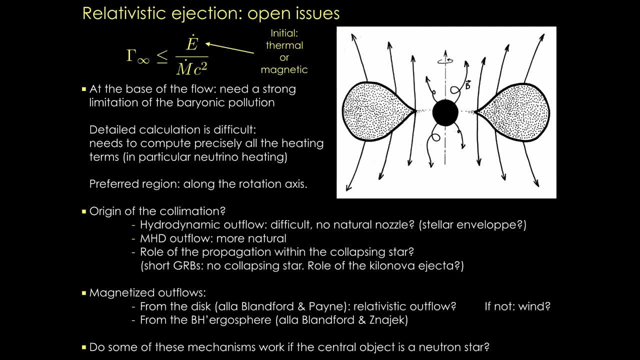 analytical or semi-analytical calculations in simplified geometry. but the full answer is not clear. Clearly there is a preferred region, which is the rotation axis. because of the centrifugal force, it is a region where there is just a small amount of matter. so if you can deposit a lot of energy, 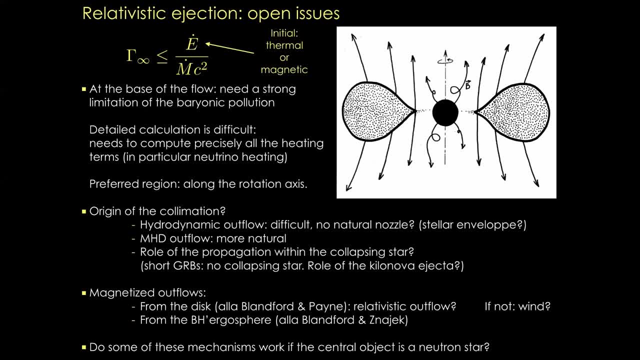 in the centrifugal region, you have a good hope to reach a hydrogen factor. There are several ideas about the possibility to produce a collimated relativistic outflow. probably it's not a pure hydrodynamical scenario like in the fireball that I discussed. 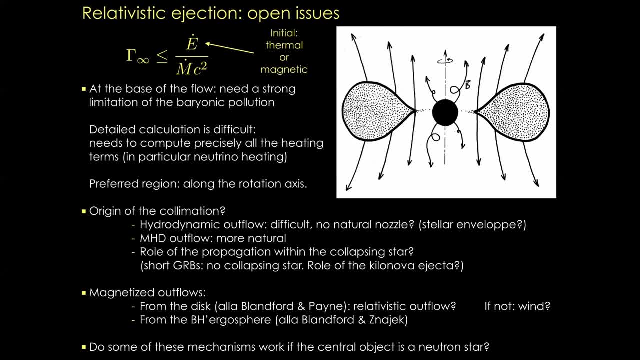 the fireball scenario I discussed yesterday, because, for instance, there is no natural nozzle to produce a collimated jet. in this case, Maybe the stellar envelope of long gamma radars could help, but it's probably not enough. So most probably it's an energy outflow and the magnetic 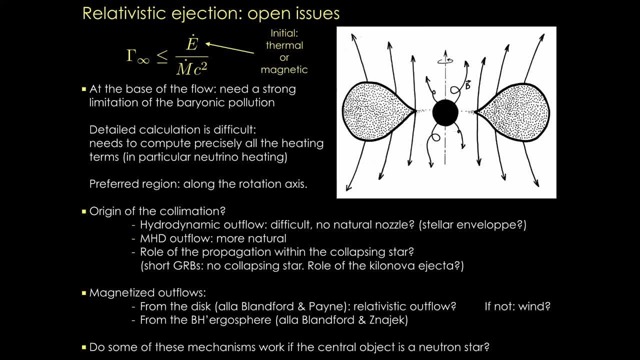 field also plays a role in the collimation. It's observed in other kinds of sources. Then it's a good question to know what will happen in the propagation in the collapsing star. does it play a role for the collimation? does it play a role for the variability? 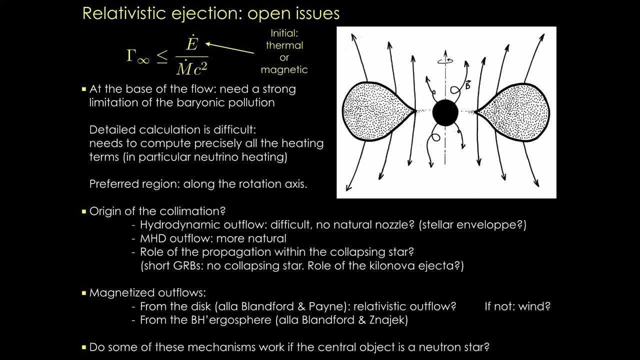 good questions and, in short, gamma radars. there is no collapsing star, so should we expect some difference? but maybe it propagates in the kilonova ejecta, As the outflow is probably magnetized. we have two standard models, either the Blonsford and Payne mechanism for magnetic. 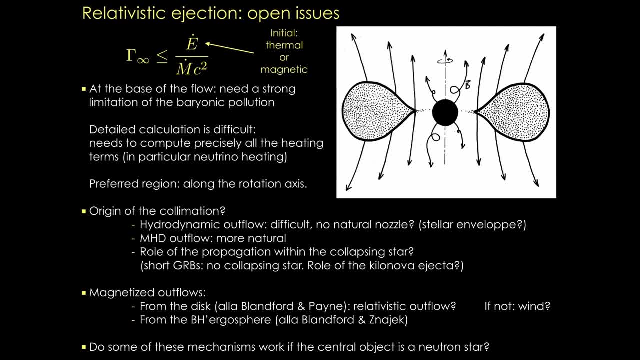 outflow escaping from the disk. it's probably difficult to have a relativistic outflow in this case, but maybe this wind could play a role also, to play a role of a nozzle to help the central outflow to start and to accelerate. and the main candidate is the. 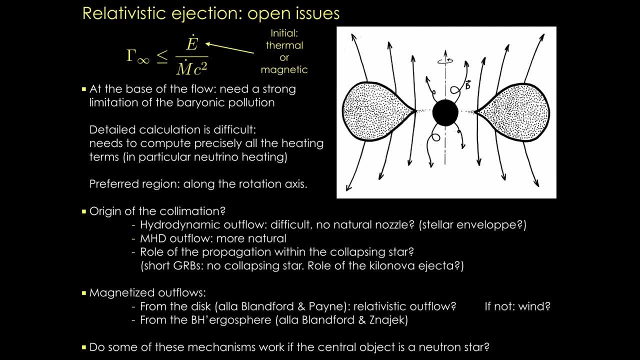 Blonsford-Nayak process associated to the ergosphere of the rotating black hole, but complex physics to compute in this highly unsteady state for such a source. a good question is to know if such mechanism could work if the central engine is a neutron star. 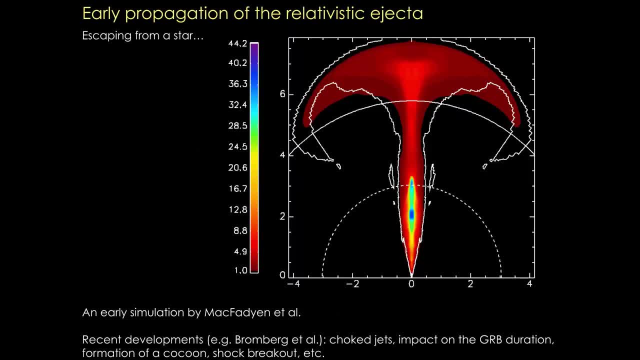 Okay, so I'm listing questions, but I'm not really answering for this part. Here I show a late old simulation by Mike Fabian of the propagation of a relativistic jet in a collapsing star. so now we are in the envelope. there were a lot of. 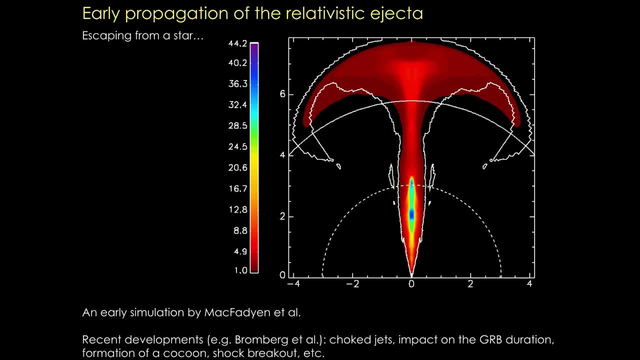 activity recently for this problem, for instance by Bromberg and collaborators, and it's very interesting now we understand better the condition for the jet to escape. in some cases we could have just a shocked jet and an interesting question is to know if we could identify an observed signature. 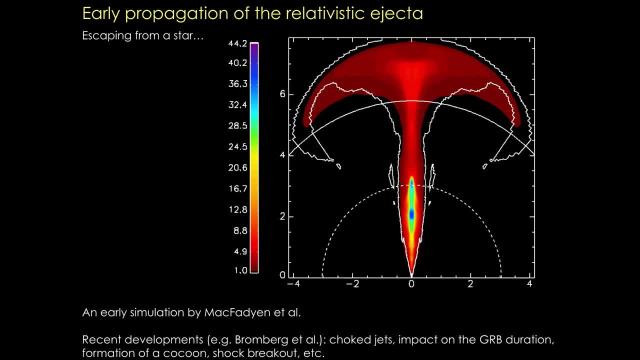 of the shock breakout when the jet finally escaped from the star. so there are a few candidates of precursors- weak precursors in gamma ray burst- which could be analyzed as a shock breakout. it's not very clear. I must say that in this phase you could expect. 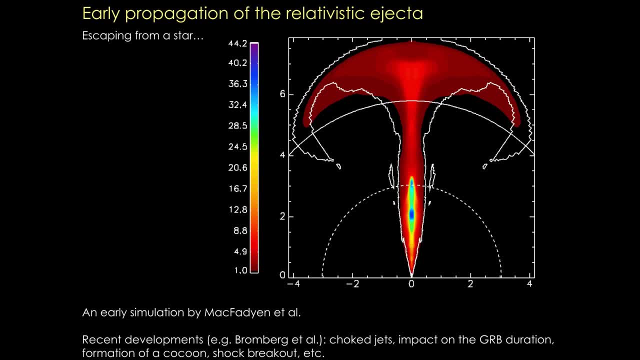 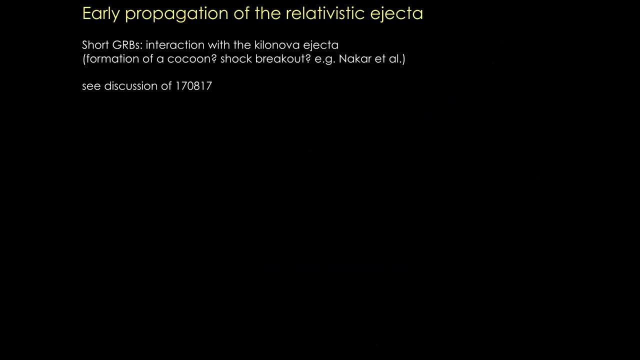 a neutrino emission during the propagation of the jet in the star. so if in the future we have detection of neutrinos, it could be very interesting to learn more about this very early phase for short gamma ray burst. I will discuss at the end of this lecture. 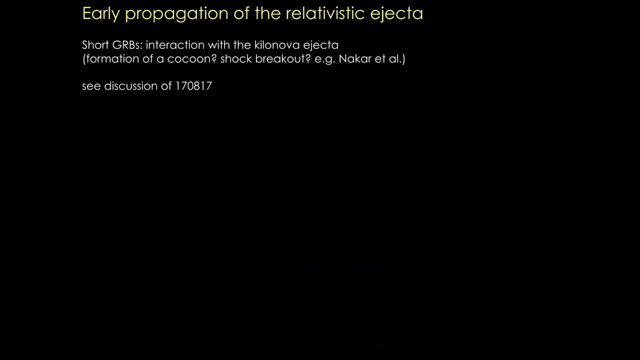 the fact that maybe the jet is propagating within the kilonova ejecta. I won't discuss the kilonova because there is another lecture devoted to this topic, but you know that in 1708-17 there are probably at least two components in the kilonova. 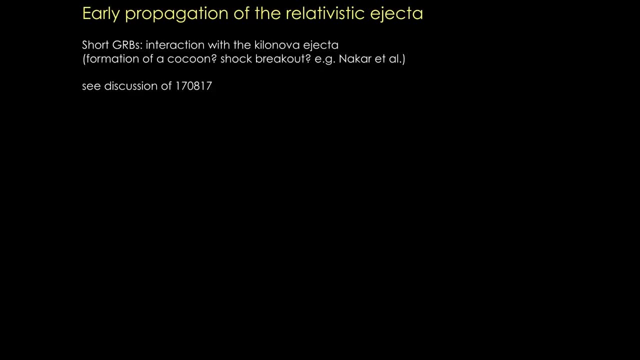 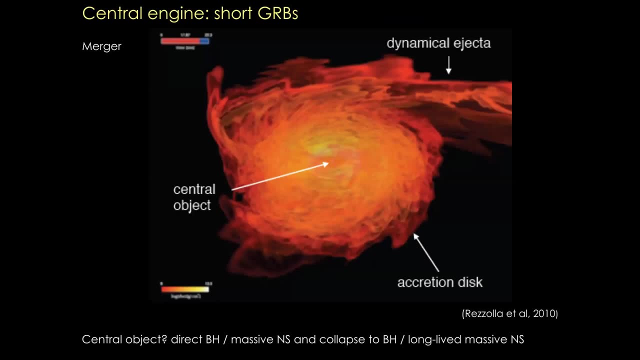 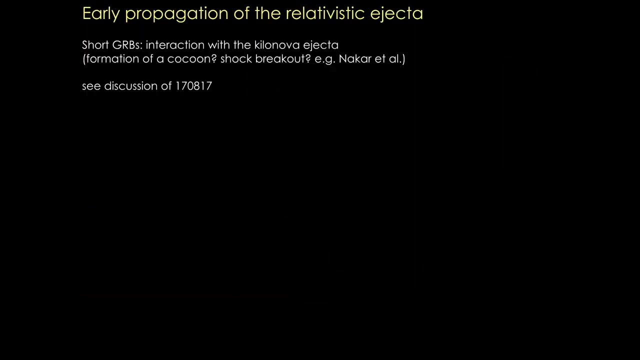 a red component associated to the dynamical ejecta which was shown here, and a blue component which is probably associated to an ejecta related to a neutrino wind and maybe the jet is interacting with this ejecta and there are a lot of related questions. it can affect the jet. 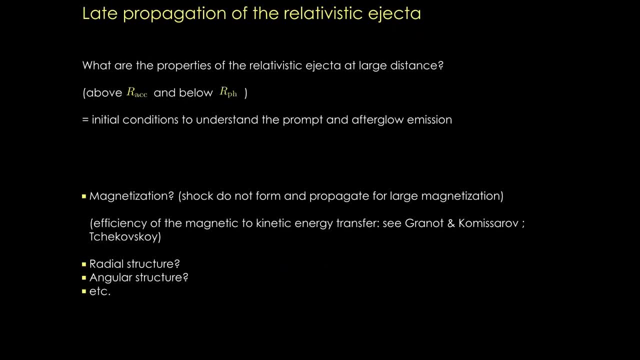 I will mention that, ok. and then, once the jet is free, has really escaped the central source, what are the properties? it's very important to understand that because these are the initial conditions to understand the prompt and afterglow emission. so we are now above the acceleration radius. 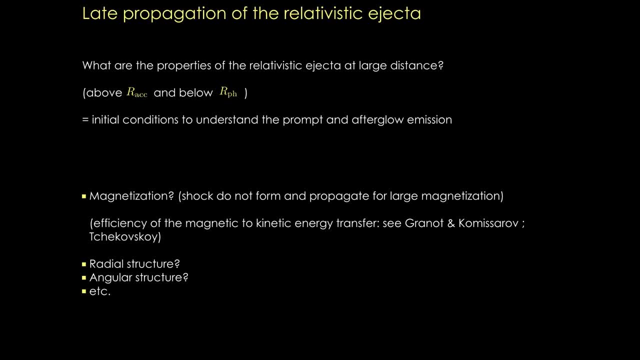 and below the photospheric radius if I use the characteristic radii I introduced yesterday. so, for instance, a very important question is the magnetization. if there is an efficient conversion of the magnetic to kinetic energy, the magnetization at large radius could now be very low, and it's a condition to have 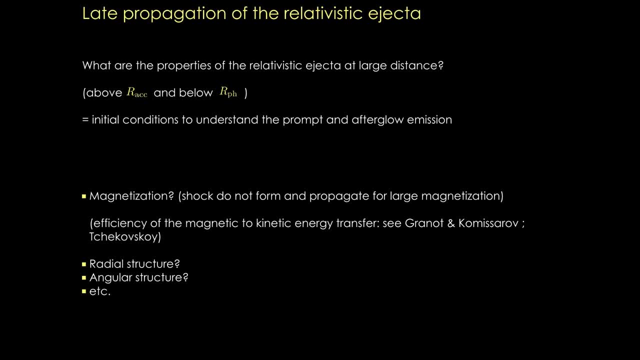 a short propagating within the ejecta. if it's still high, then probably the main dissipation process has to be taken in a reconnection event. so there is a lot of discussion about the efficiency of the conversion of the magnetic to kinetic energy and you could have a look. 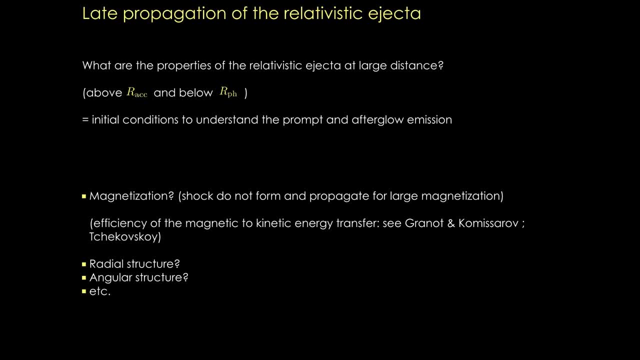 at work by these two groups, for instance Granot and Komissarov, have shown that if the source is highly unsteady, so ejecting impulsively some material which is initially highly magnetized, you could have a very high conversion, a very high efficiency of the conversion. 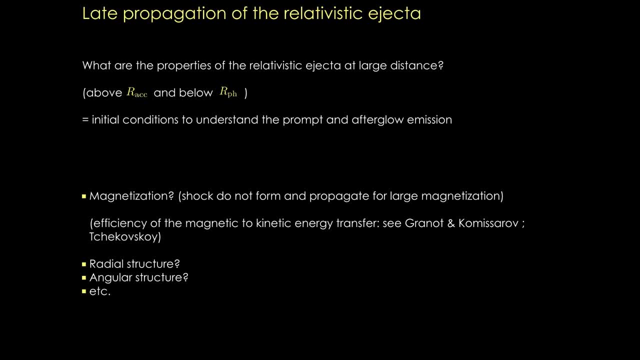 so here magnetization is important, but we will see that, for instance, especially to model the afterglow, the angular structure of the outflow is also very important and it could have been affected by all the processes I listed, and the radial structure is also very important. 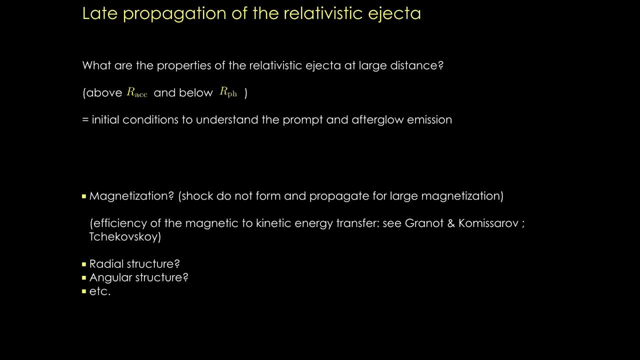 for instance, for internal shock to occur you need an outflow which is still very variable, with a strong gradient of velocity. I see a question about the cocoon energy. so for long gamma ray burst, to my knowledge for the moment there is no consensus about a possible. 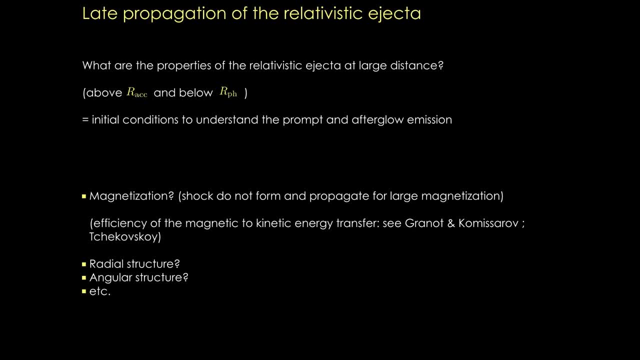 observed signature of a cocoon, but if a cocoon was clearly identified, then the energy in the cocoon should be included in the total energy budget of the phenomenon, of course, but I expect it to be much less than the main jet in the case of 170817. 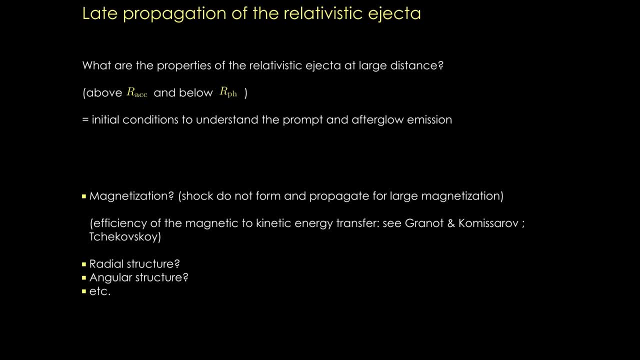 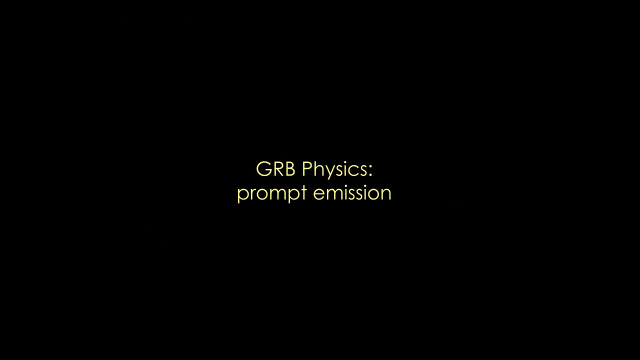 the energy in the lateral structure, which sometimes is called a cocoon, is much less than in the central jet. ok, so I will stop here for the discussion of the progenitor and the relativistic ejection, and now I would like to add a few words about the. 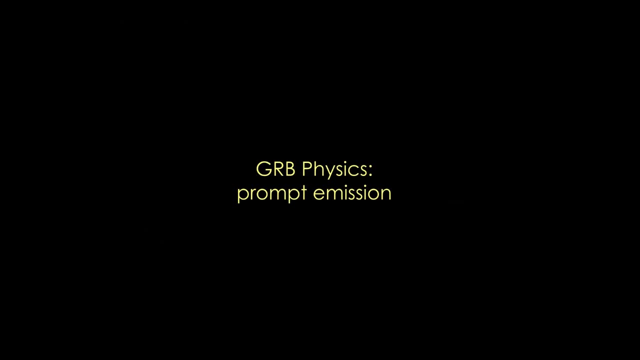 quantum emission. Frederic, there is a question from a youtube viewer. I am just typing that. yes, thank you. it is about the progenitor. that is why I thought I will ask it, so it is an excellent question. in the case of 170817A, we know that. 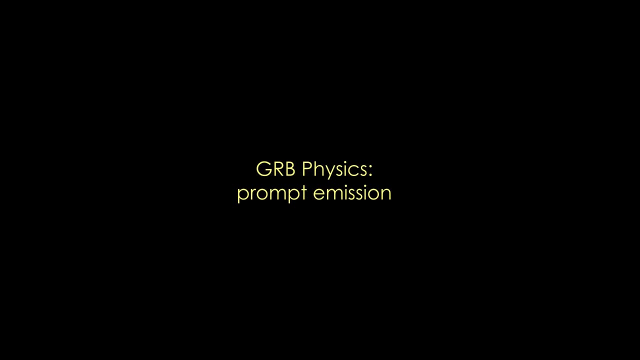 the initial system is a binary neutron star. I think there is still a very small possibility that the initial system has one of the two objects to be a black hole, but the probability is quite low. it is very interesting to expect in the future to have neutron star black hole. 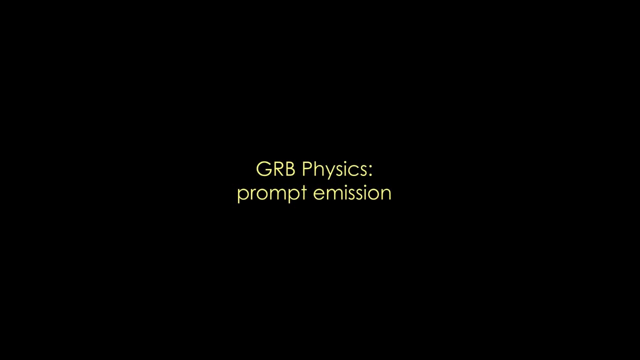 merger. we already have observed such events during the 03 run, but without any electromagnetic counterpart. I hope that in the future we will have electromagnetic counterpart for such events, probably during 04. the capacity to look for counterparts will be much better, especially with the addition of LSST in the network. 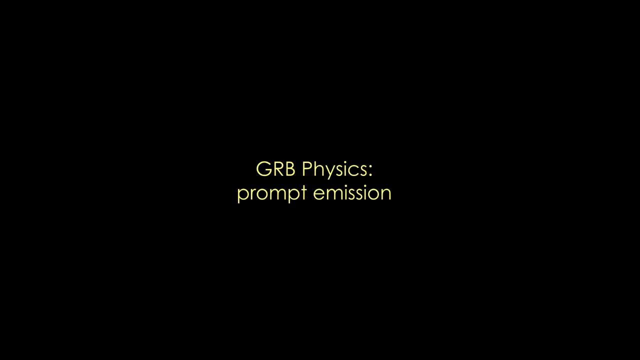 and I hope we will have more electromagnetic counterparts and it is very interesting to know which diversity we will observe when we will compare, let's say, neutron star, neutron star black hole systems with a low mass ratio and neutron star black hole system with high mass ratio. we can expect a great diversity. 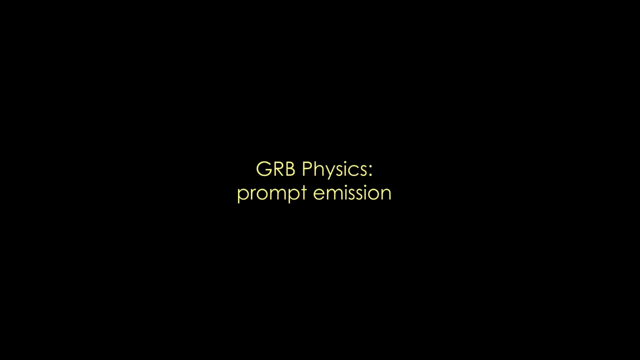 of behavior, because in some cases we can expect the neutron star to be destroyed by tidal forces before reaching the horizon of the black hole and then forming a disk around the black hole, and in this case we can expect the same kind of phenomenology than for neutron star. 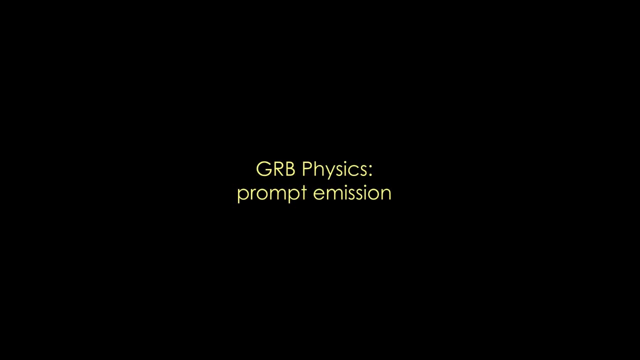 because the reservoirs are not the same and for all high mass ratio, it is very possible that the neutron star just reach the horizon of the black hole without being destroyed, and maybe in this case there is just no electromagnetic counterpart that we will see. so it is a very good question. 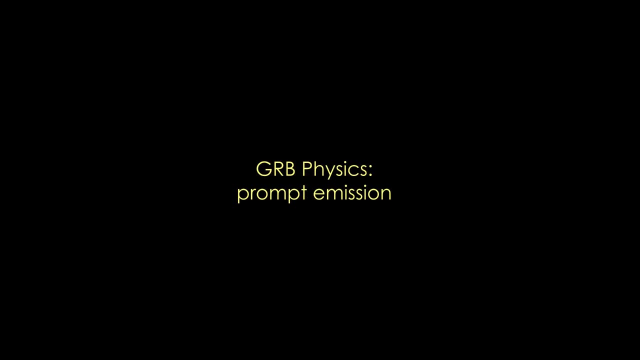 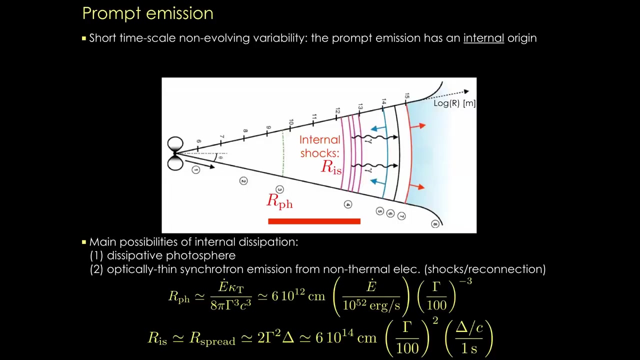 I am very interested in this question, but I will say that for the moment we have to wait for observations. we have to test them now. ok, so now I switch to prompt emission. so I show again this picture with the characteristic radii and I will focus first on the scenario. 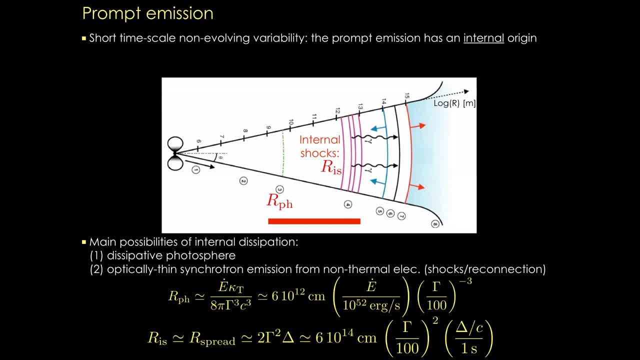 where the prompt emission is produced by internal shocks, because it is the first scenario which has been discussed and it has been used in many other. things can be computed in detail, so you can do a very detailed comparison with observation and so we can use this model as a reference. 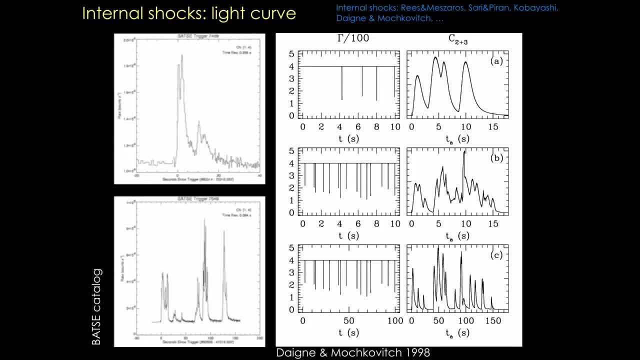 to compare with other possibilities. so here I show for instance again two examples of gamma-ray burst light curves on the left, and I show examples of synthetic light curves produced by the internal shock model. and this is the calculation I made in 1998. so the first column shows: 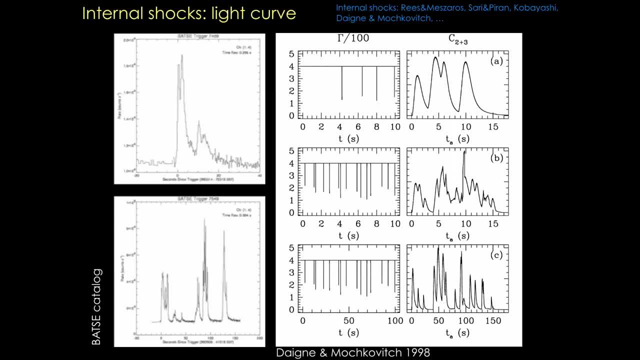 the distribution of Lorentz factor in the outflow. so you see it is a highly relative thick outflow with a mean Lorentz factor of 400, and you have some parts which are have a much lower Lorentz factor, for instance because suddenly, 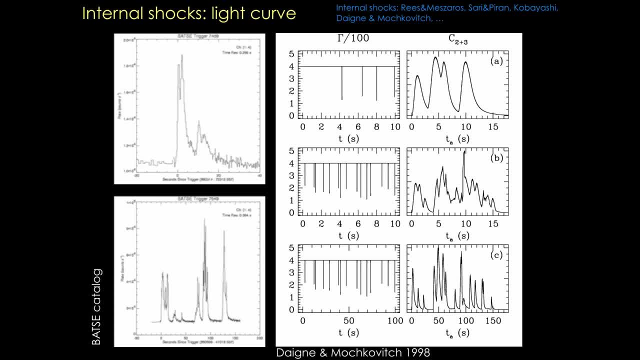 the bionic pollution was higher than before. and then the idea is that the fast part with the slow part, producing shock waves propagating within the ejecta, and electrons are accelerated in the shock region and the magnetic field is amplified and these electrons radiate by synchrotron radiation. 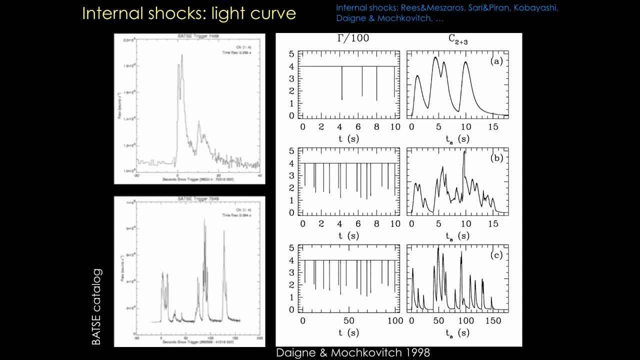 to produce the light curve which is on the last column on the right. I see that there is also a question about the opening angle of the gamma-reverse and the off-axis view. so for the off-axis view, I think that it's a pure external parameter. 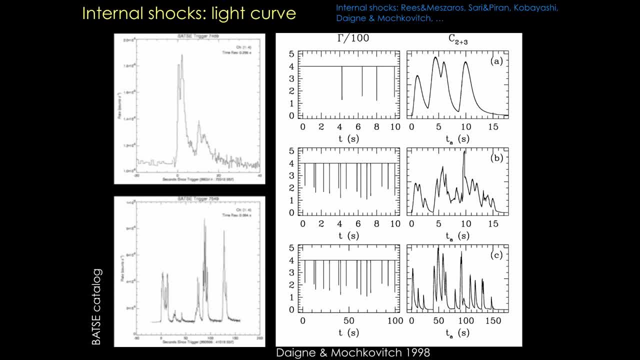 it just. you can compute the probability to observe a given system with a certain off-axis view. but if you believe that there is no preferred direction in the universe, there is no impact of the nature of the source on the probability of the off-axis view, except a small effect. 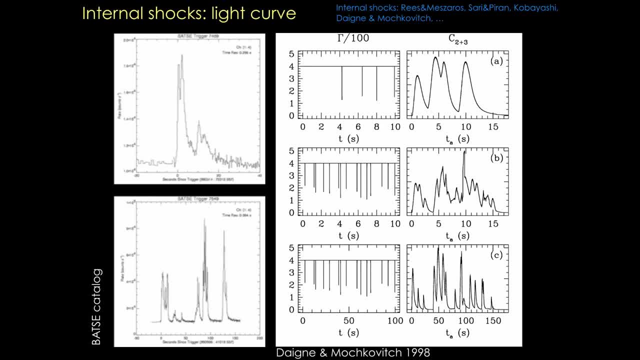 which is that for gravitational waves you are a little more sensitive if you see the system face on, so it produces a small bias here. on the other hand, it's very possible that the mass ratio has an impact of the opening angle on the nature and mass of the central object. 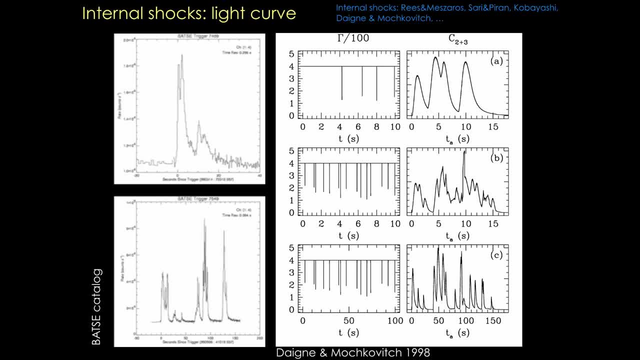 on the mass of the disk and then it should have an impact on the ejecta, maybe the opening angle, but maybe also the duration of the ejection, the energy, many things we do not know yet. ok, so maybe I will just make a short calculation to explain a very important fact. 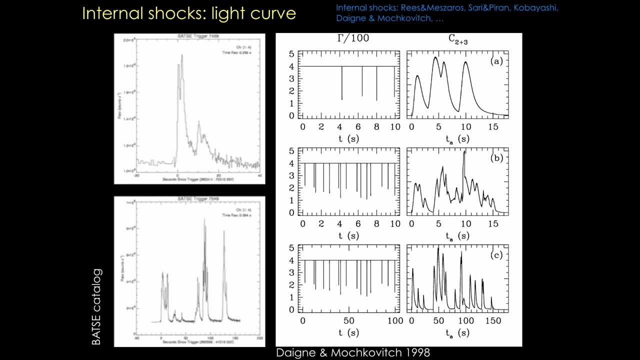 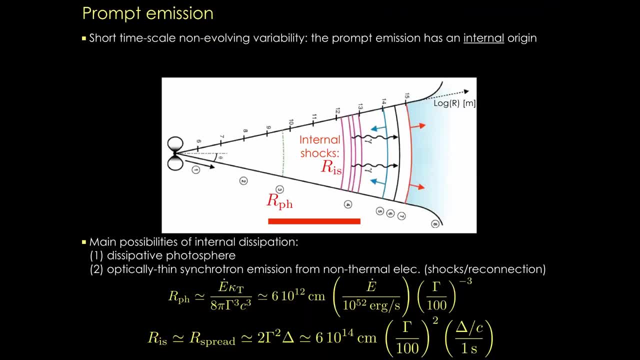 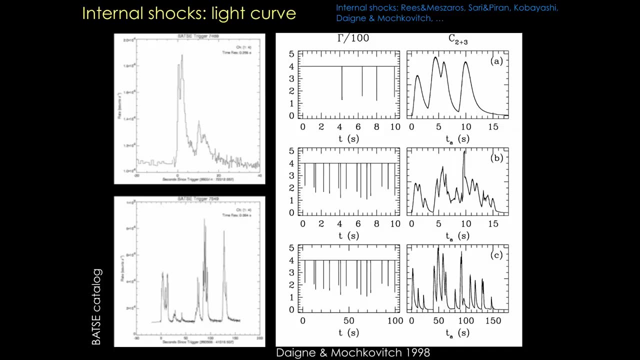 here you see that the emission which is shown on this picture is produced at a large radius. it is shown with this equation here- sorry this equation, but still- we see a strong variability in the light curve. in fact, we see in the light curve the same variability than the variability introduced by the central energy. 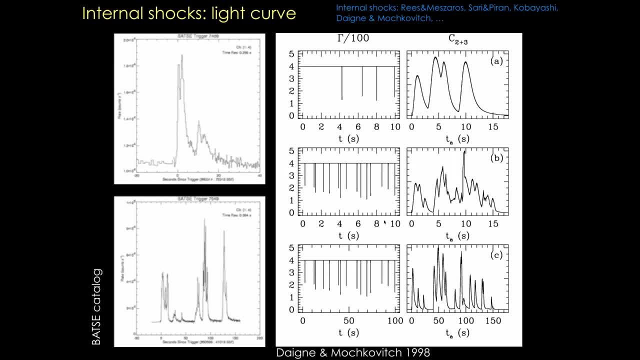 you see here that, for instance, the ejection lasts for 10 seconds, with variability below the second time scale, and the gamma ray burst lasts for also a little more than 10 seconds and with variability at the sub second time scale. so it seems that the light curve. 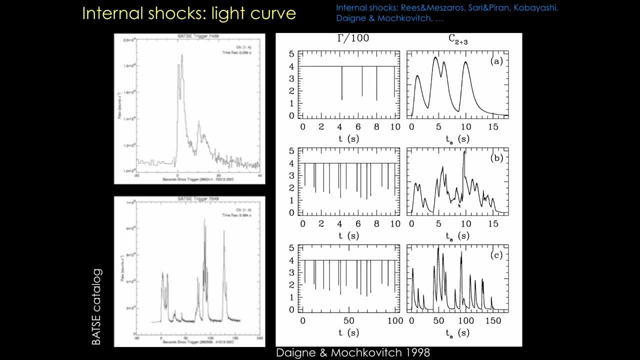 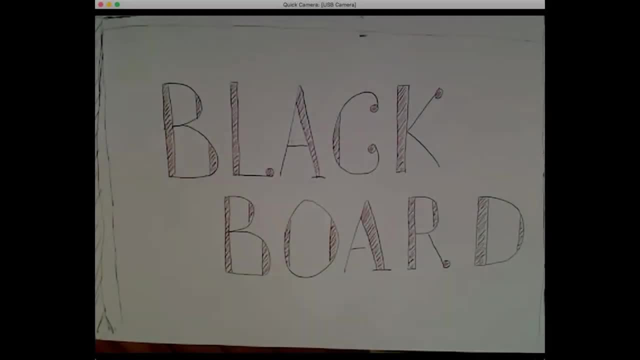 is a good mirror of the activity of the central source and it is very easy to understand. so I will show that with a rapid calculation. so I switch to my camera one second. so the idea is the following: I will make a very basic version of the internal shock model. 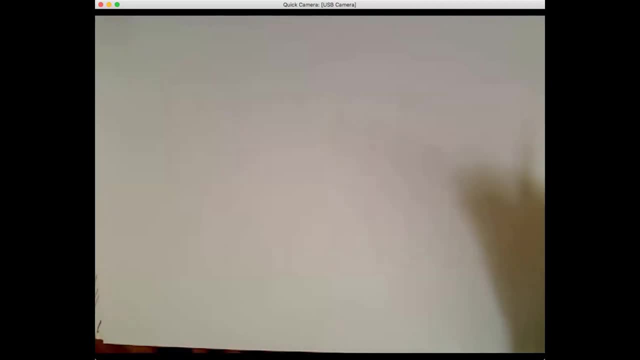 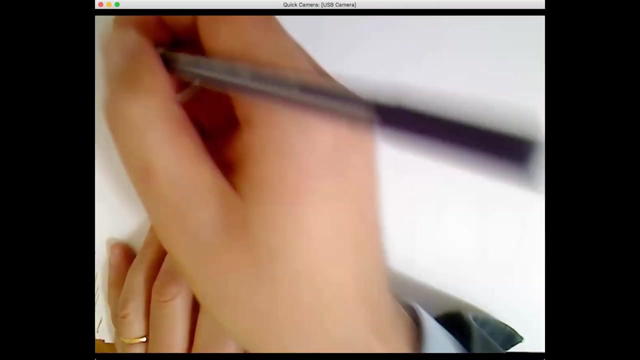 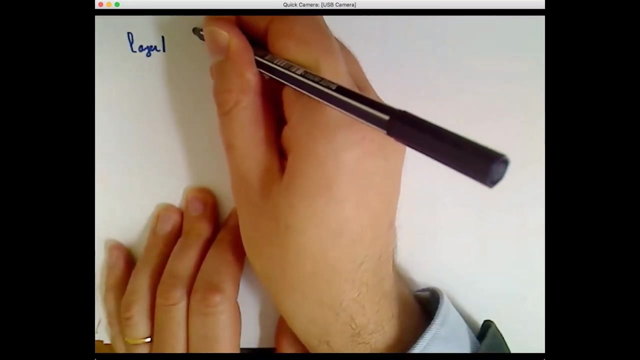 where I will do what is called a ballistic approximation. I neglect all the propagation of pressure waves. I will consider two layers which move ballistically and will just directly collide when they meet. so let's consider the first layer emitted at time: Te for ejection with velocity. 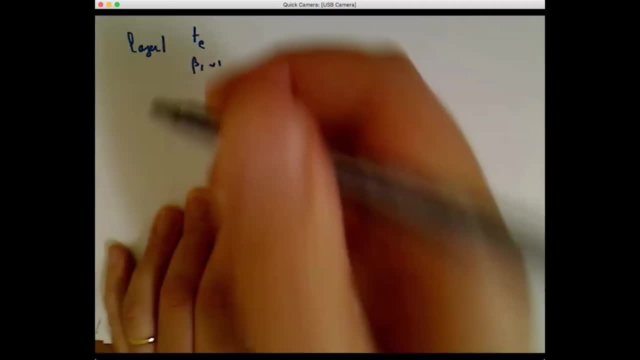 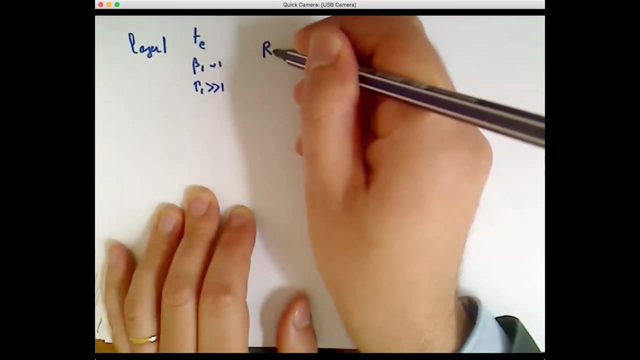 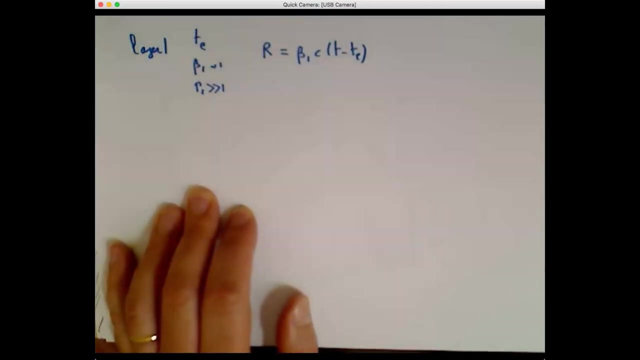 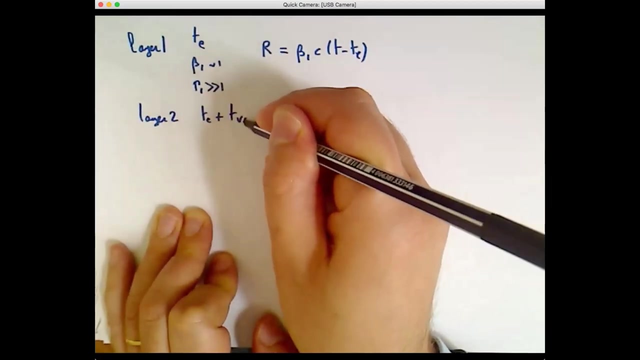 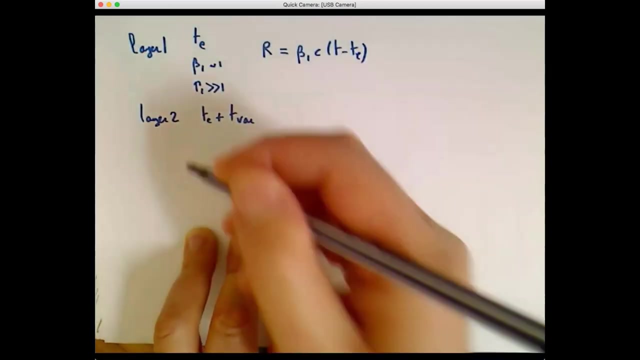 beta one, which is close to one, or gamma one Lorentz factor, which is larger than one. so the motion of this shell is just given by this simple equation. and consider a second shell which is ejected later, and I call Te var the typical duration between the two ejection times. 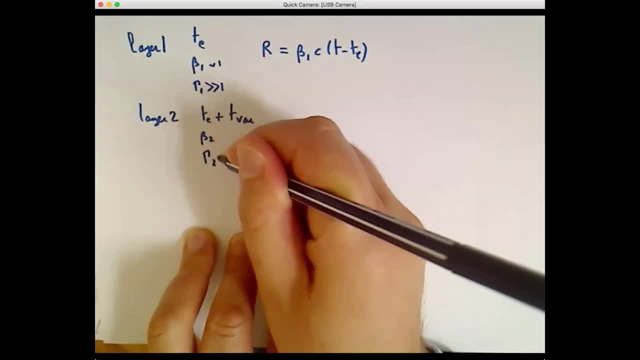 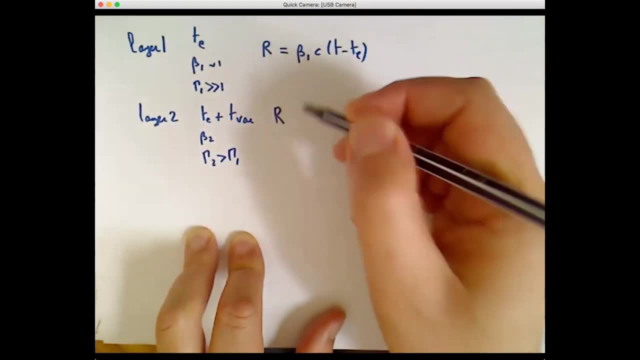 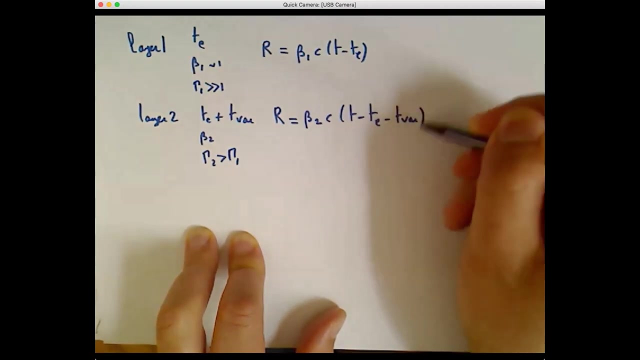 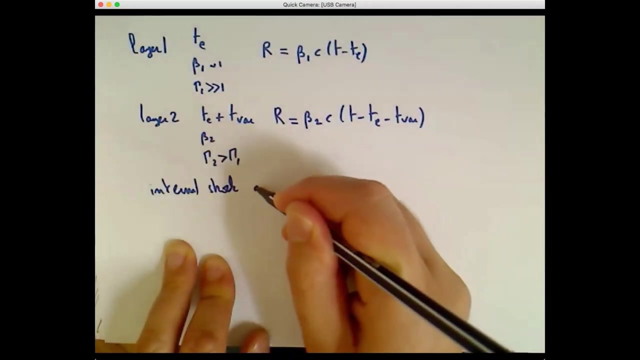 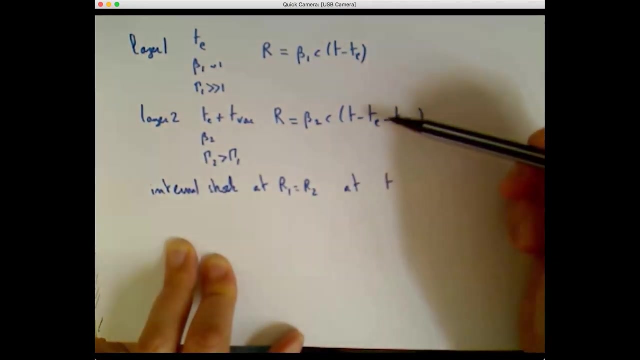 now beta is beta two and gamma two is larger than gamma one, so it means that it goes faster and it will collide with the first one. ok, so now internal shock will occur when the two radius are equal, so it corresponds to a time. so I have to find equality between these two radius. 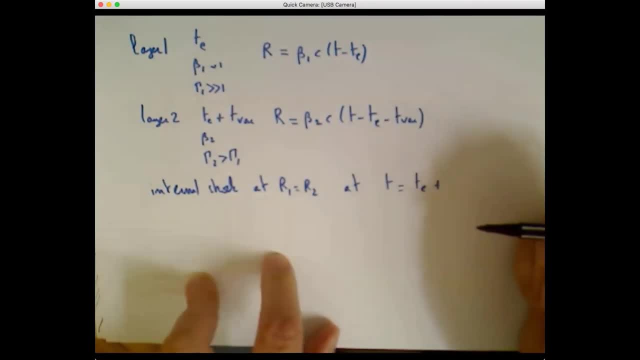 and you see that it's the emission time, the ejection time, plus beta two over the relative velocity, beta two minus beta one times Te var. ok, and then I will call that the internal shock time. and what is the internal shock radius I have to inject this time? 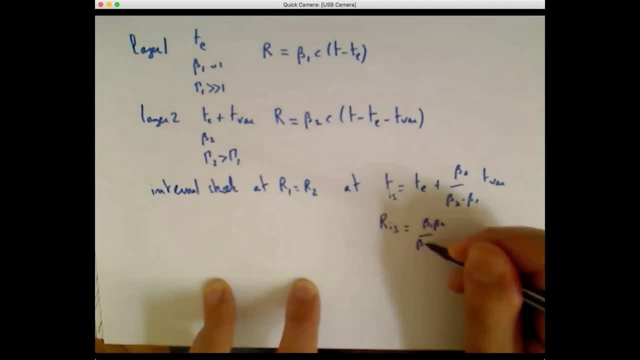 in this equation and I get beta one, beta two over beta two, minus beta one, Te var, I can make a ultra relativistic approximation. I can say that beta is small to one. so this factor is one and this factor is just the difference of one over two gamma square. 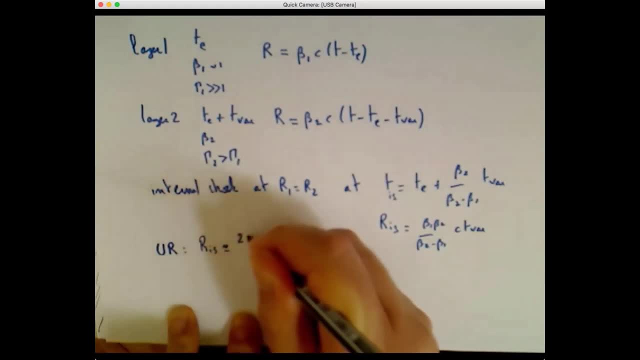 so it will give a radius which is two gamma one square, gamma two square divided by gamma two square minus gamma one square, Te var and then I can say that beta two is larger than gamma one, just for simplicity. it's not mandatory for the model, but here it's for simplicity. 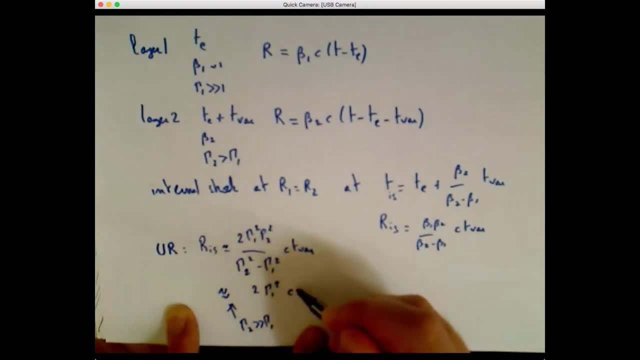 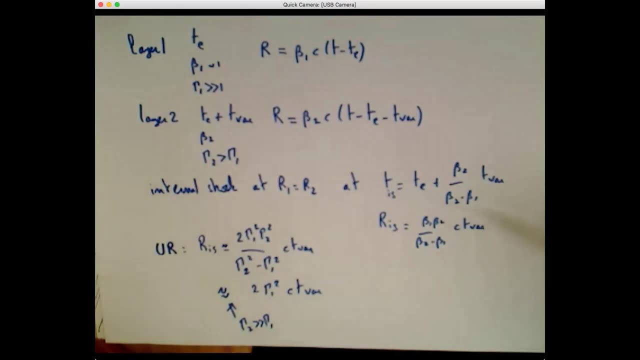 you see that here gamma two cancel and I get two gamma one Te var, which is exactly the estimate of the internal shock radius I gave yesterday. but here the derivation is a little more precise. so once I know that the collision occurs and at which radius, a very important 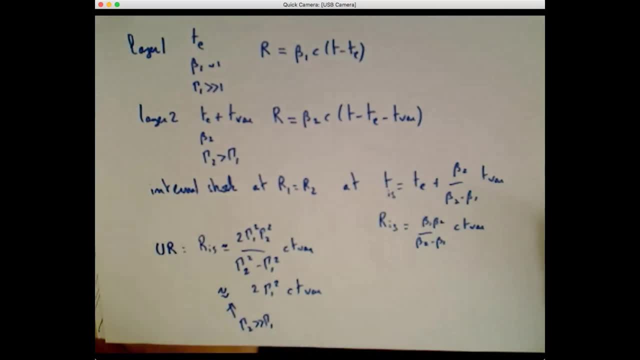 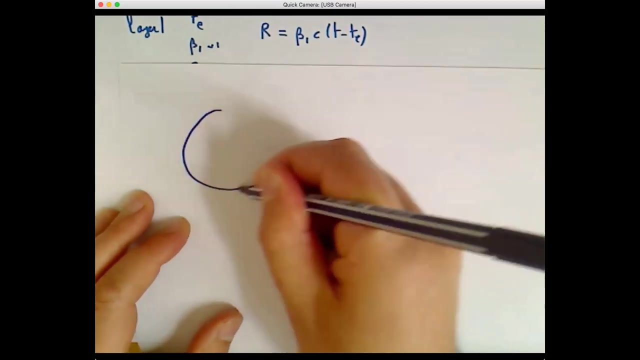 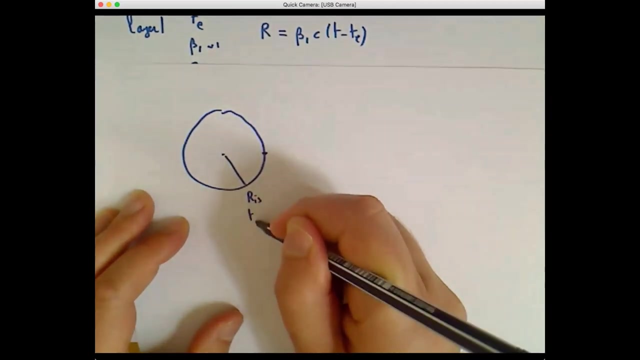 additional information is the time at which the observer will receive the emitted photons by the collision and on which time scale this emission will be smooth. so I can compute that easily: if, if the emission is produced at the radius of the internal shock and time of the internal shock. 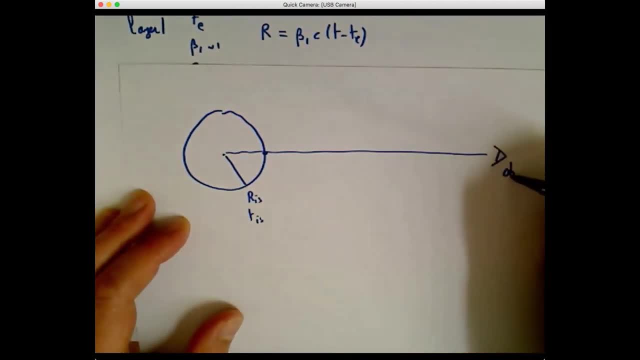 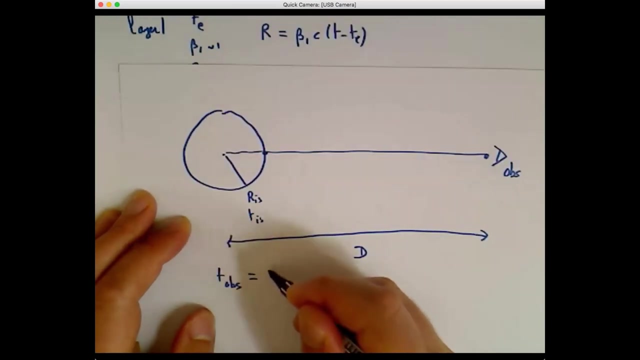 and if the observer is here- this is the distance between the source and the observer- then the overall time of photons for the observer will be given by the emission time plus the time needed for photons to go from the location of the internal shock to the observer, which is 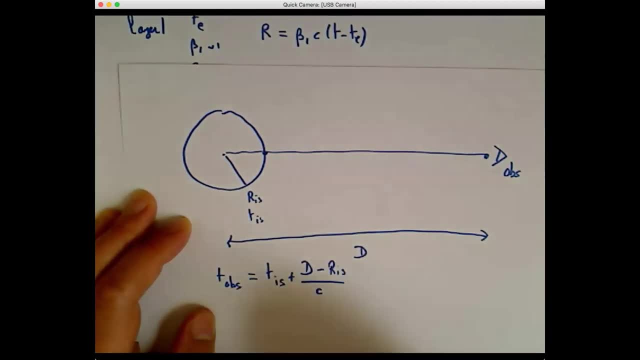 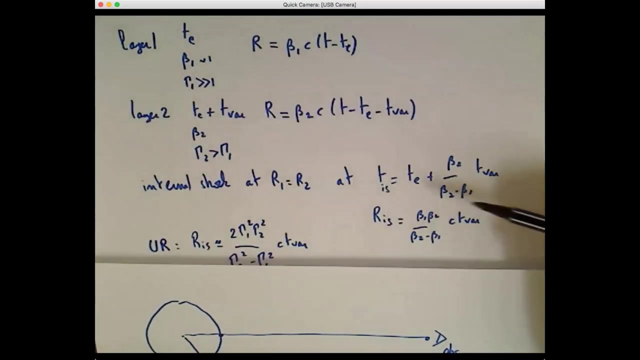 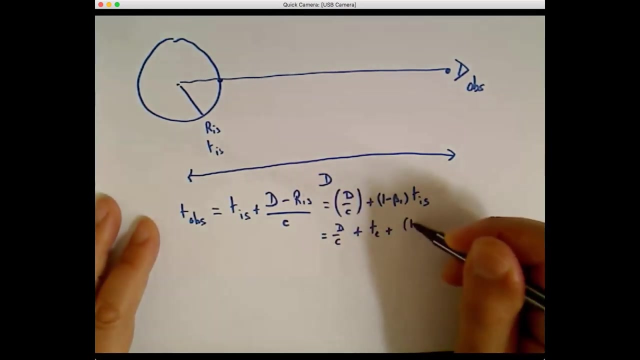 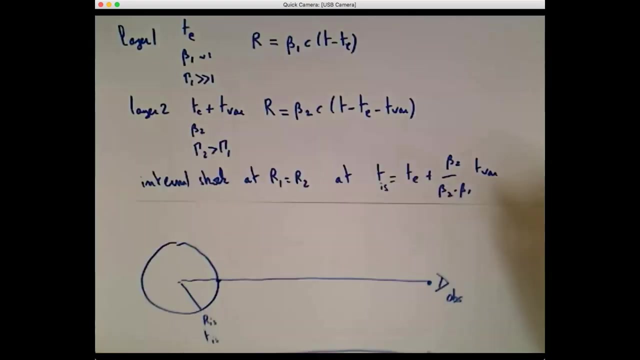 d minus l internal shock divided by c. so d over c is not important, it's just a constant and this factor is just even than one minus beta one time of internal shock. so if I use this expression, I get this. I inject that in this and I get this expression. 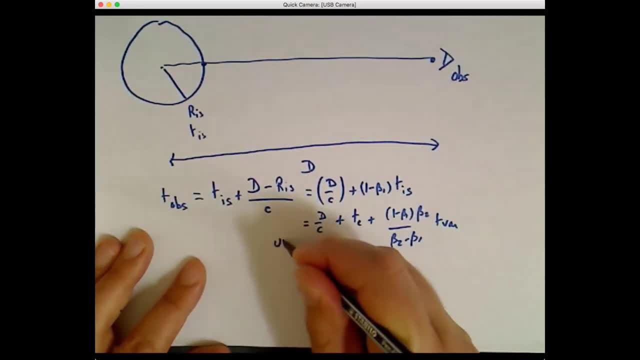 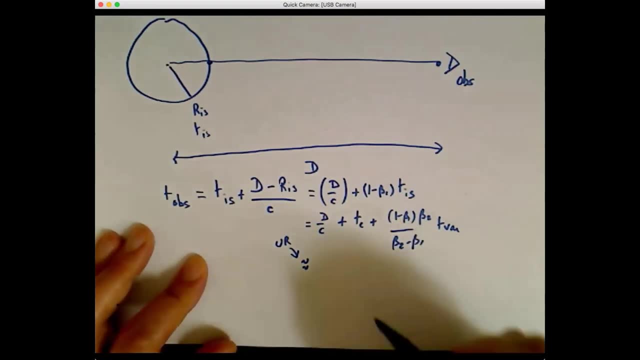 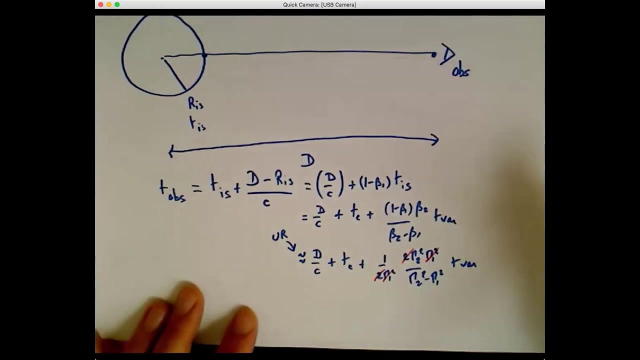 and if I take the ultra-relativistic limit, you see that this is one, this is one over two gamma one square, and so I get d over c plus te, plus one over two gamma one square. two gamma, two gamma, one over. so this factor cancels. 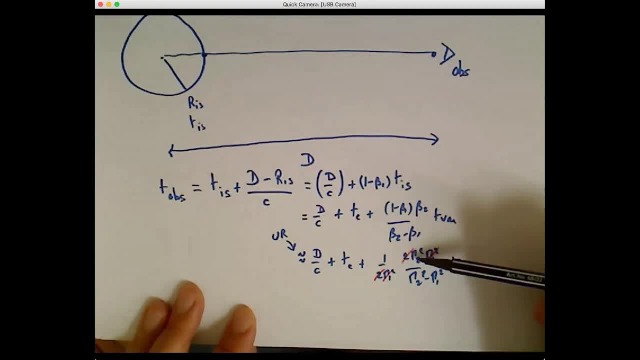 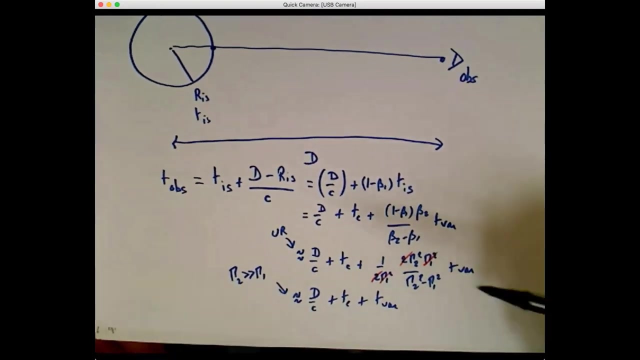 and if, in addition, I assume, like before, that the second Florence factor is much larger than the first one, I get a very simple expression like this. so you see, it's very nice, because it means that it's dominated by the ejection time and it means that 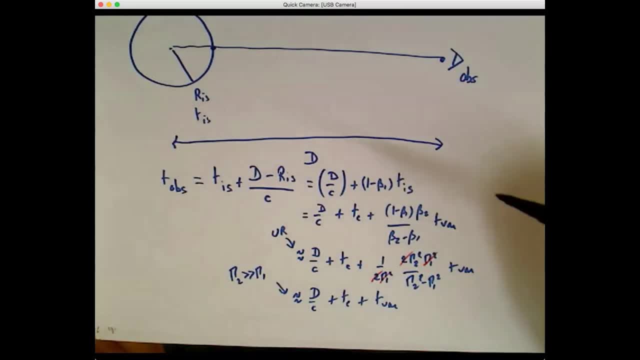 I have a clear mirror of the activity of the source. if I have an ejection at 0.5 seconds, then one second, then three seconds, then five seconds. I will see as many pulses in the light curve so that this emission is not smoothed out over a too long timescale. 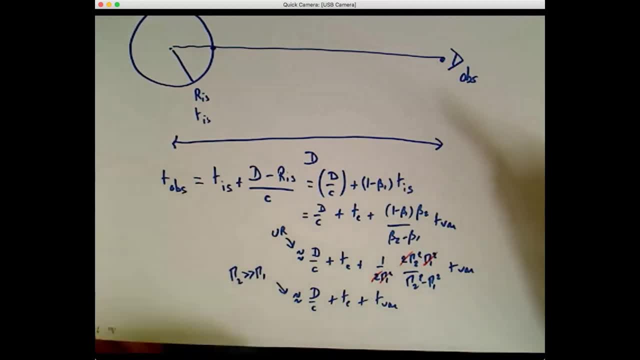 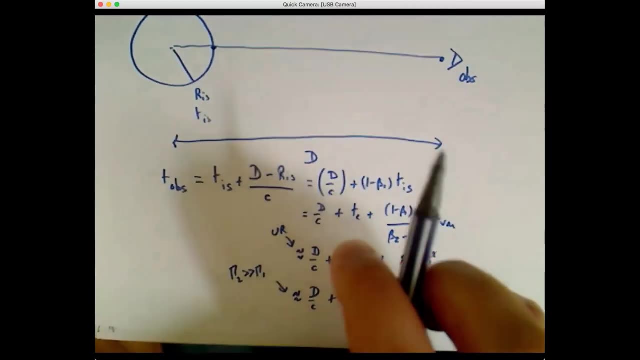 otherwise it would smooth out everything. so I can also check on which timescales the contribution of each collision is smoothed out, and it is done by using the same timescale I computed yesterday. you remember that before because of the relativistic beaming, I observed radiation coming only. 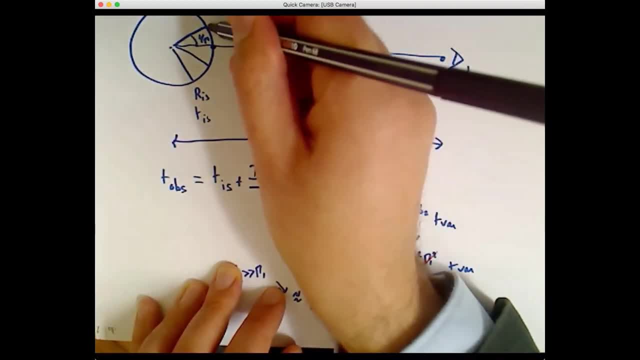 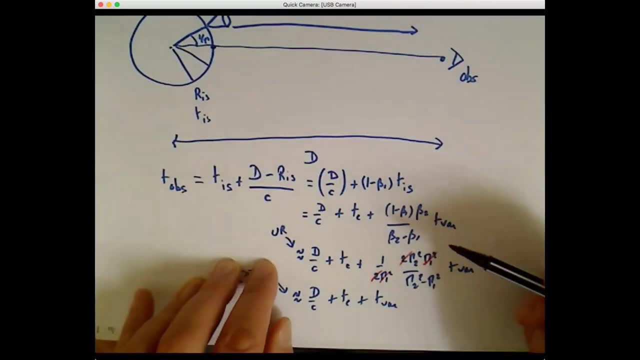 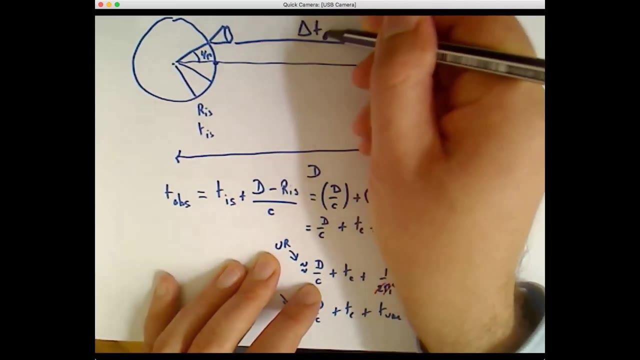 from this region with an opening angle 1 over gamma, because here the relativistic beaming is still like that, and at higher latitude the relativistic beaming is such that I cannot receive photons. and you remember that we estimated that the corresponding smoothing timescale for the observer 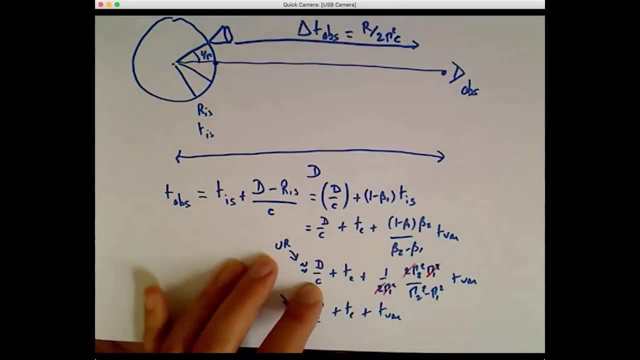 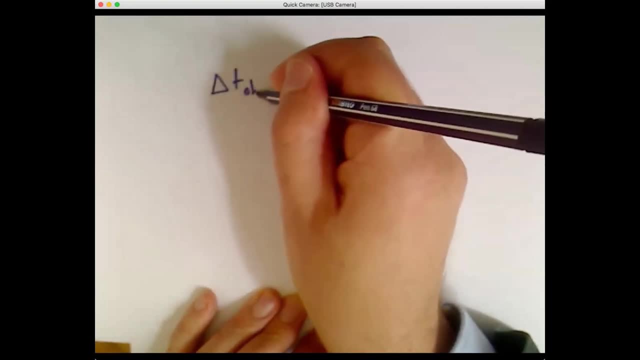 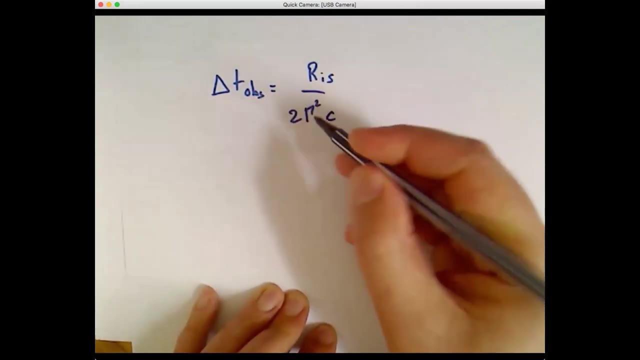 was r over 2 gamma squared c, so I can compute this for internal shocks. it will be the radius of internal shocks divided by 2 gamma squared c. what should I take for gamma? I should take the Lorentz factor of the shocked material. so it should be. 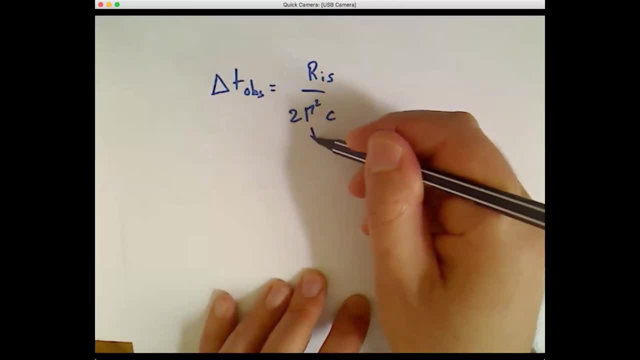 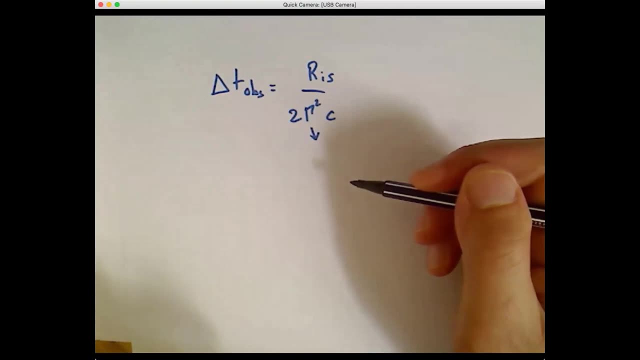 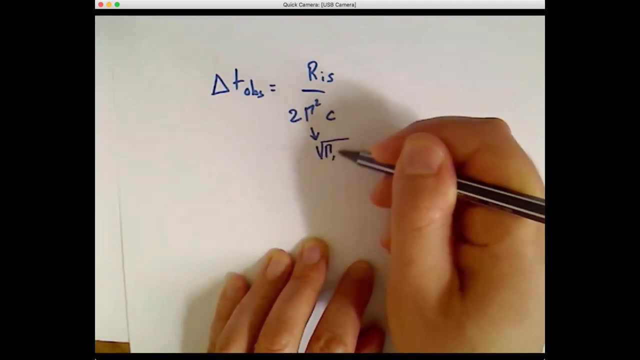 between gamma 1 and gamma 2 after the collision. you could show from standard relativistic kinematics that if you have a mid-elastic collision between the two layers where they merge and if the two layers have the same mass, it is just the geometrical mean. 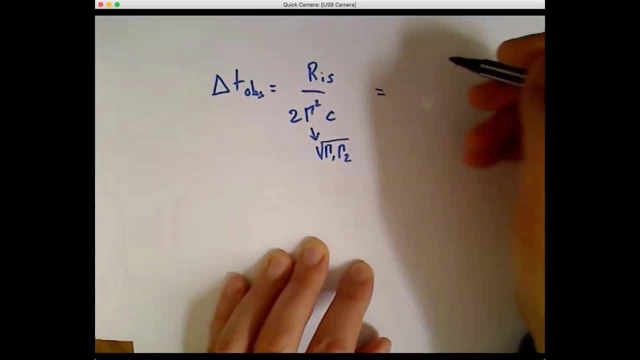 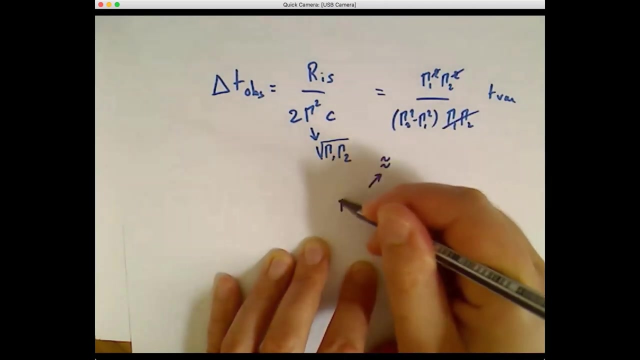 of the two Lorentz factors. and so if you replace, you get that and you see that it vanishes like that. and again, if gamma 2 is large compared to gamma 1, this term is dominant and I get gamma 1 over gamma 2 t bar. 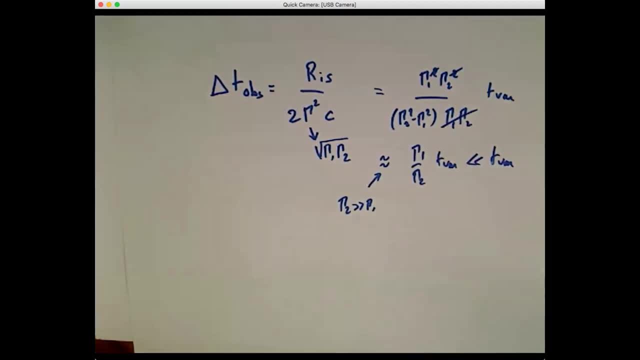 which is much smaller than t bar, so I can recover the initial variability in the engine. so this argument is really important because you see that in the internal shock model the light curve is really a direct history of the relativistic ejection of the central engine. of course it's not so direct. 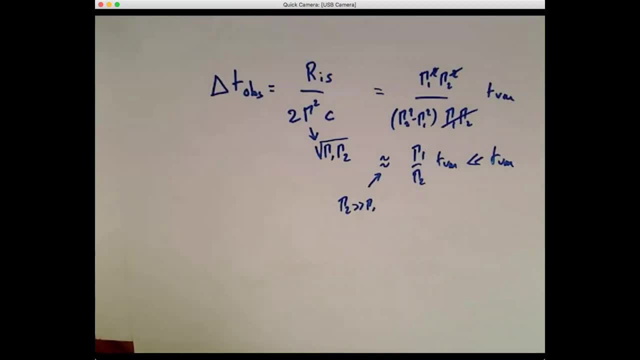 if you take into account additional physics for the acceleration of particles and then the radiative processes, so the spectral corrections, things like that. but still you can consider that, for instance, the duration of the burst is clearly related to the duration of the relativistic ejection and the different variability timescale. 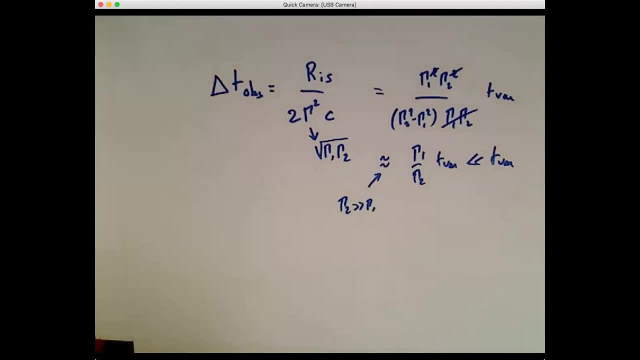 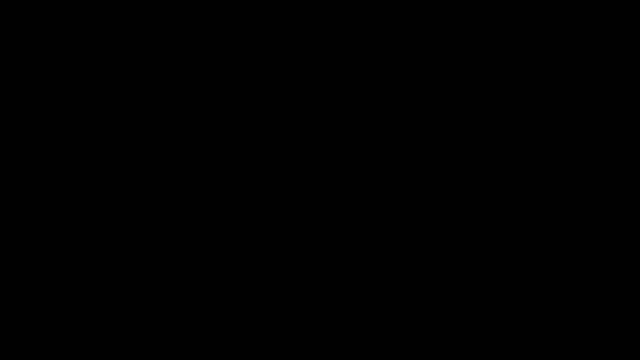 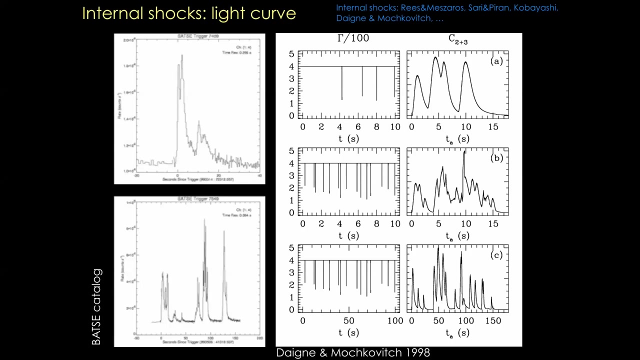 found in the light curves are directly related to the initial variability timescale in the central engine. so it's a very nice property of the internal shock model, and here I have just shown the basic calculation showing that. ok, so I come back to my keynote. so I don't know. 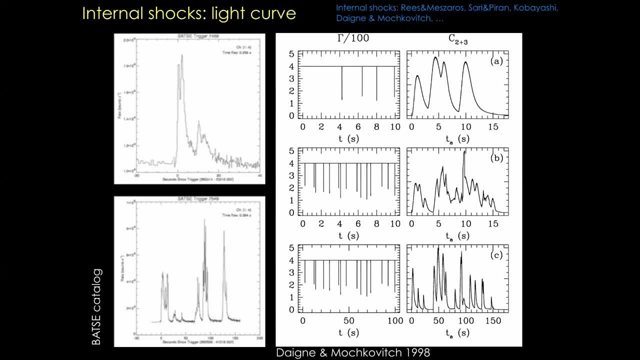 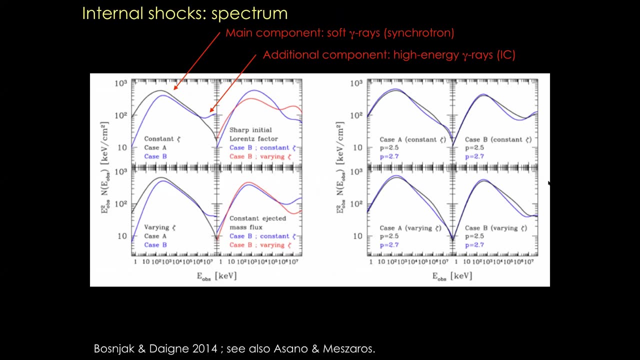 if you have some questions about this calculation. and then once we have understood light curve and the origin of the variability in the light curve, we can focus more on on the relative processes. so here I show a more recent calculation where now the dynamics of internal shocks is coupled to a full 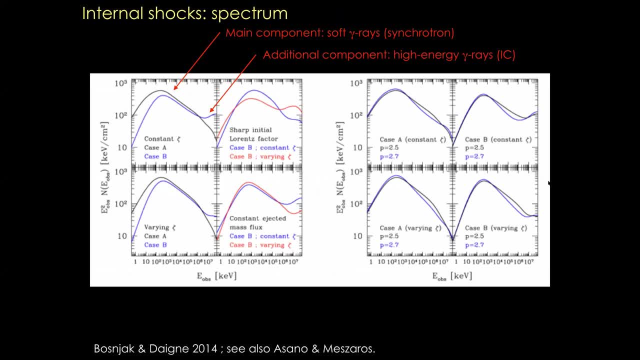 radiative calculation so included the cooling of electrons by synchrotron radiation- inverse quantum scattering. it includes also the adiabatic cooling due to the spherical expansion, and many radiative processes are included. in addition to synchrotron and inverse quantum, we have also the gamma-gamma annihilation. 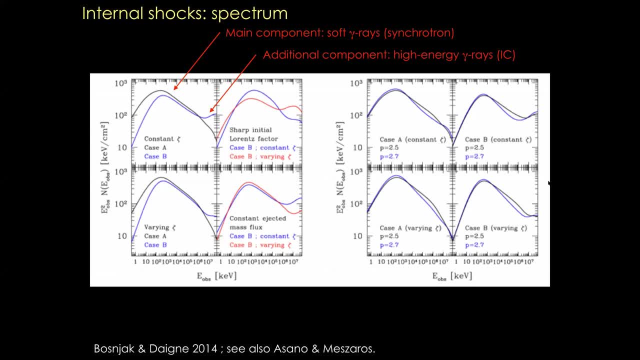 that I discussed yesterday, and also the synchrotron self-absorption. so it's a very detailed model and you see that we can clearly reproduce a soft gamma ray component, which is dominant, and an additional component due to inverse quantum, which can be either or emerge. 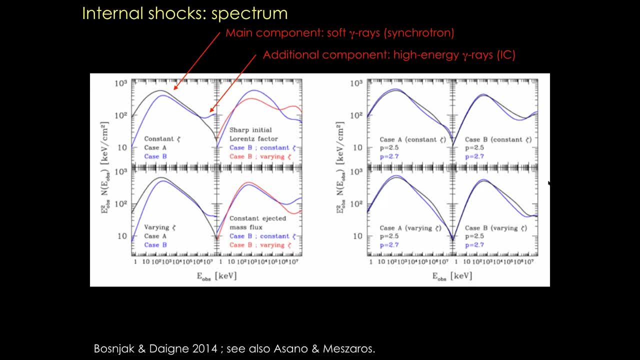 and which could reproduce a diversity of in Fermilat. I should mention that we are here in a case where electrons responsible for the synchrotron radiation are very high in Lorentz factor, and then we reach very easily the Klein-Ishina regime. 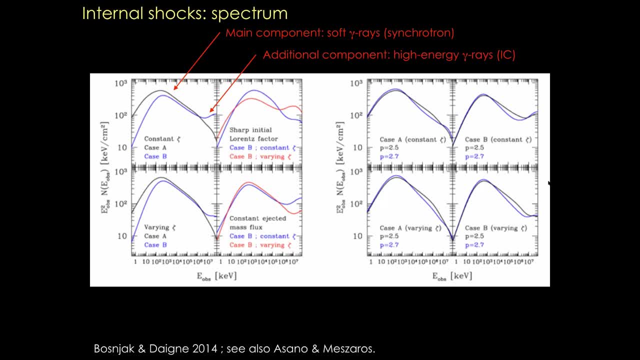 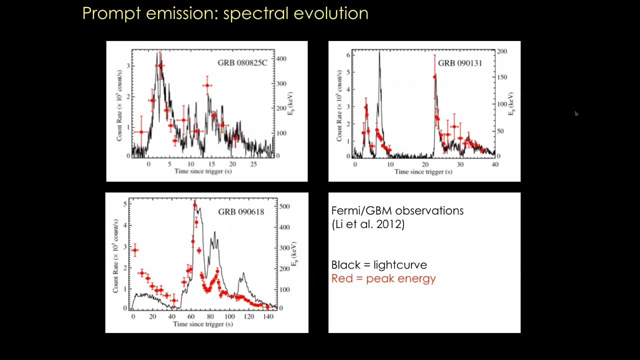 so inverse quantum scattering are strongly limited and the main component is the soft gamma ray component, in agreement with observation. another thing that we can test for such a model is the spectral evolution. here I show a few examples of Fermi bursts, where the bursts are bright enough. 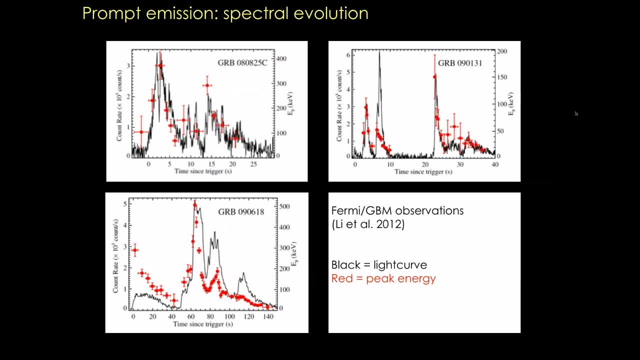 to allow for spectral analysis, which is time dependent, and the black curve is a light curve and the red points show the peak energy of the spectrum evolving with time, which is a strong evolution, and especially that we should consider that there is a strong evolution within each burst. 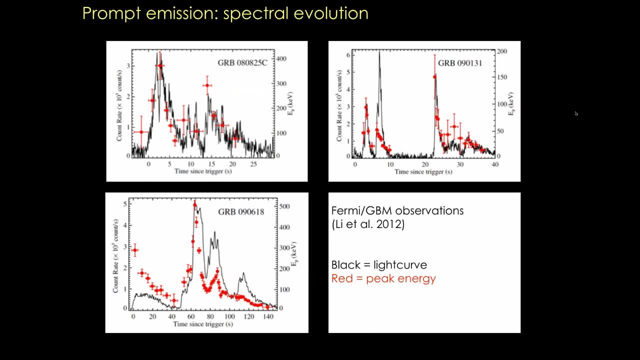 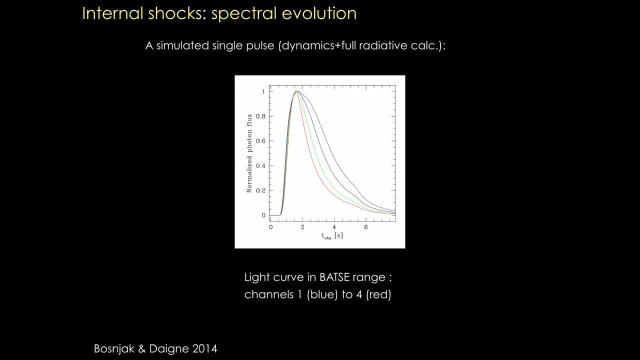 initially the peak energy is very high and it decreases when the flux decreases. so in internal shocks we can reproduce that, because initially the shock is very strong and then it propagates in the ejecta and it becomes weaker during the radial expansion, and so the condition in the shock region evolves. 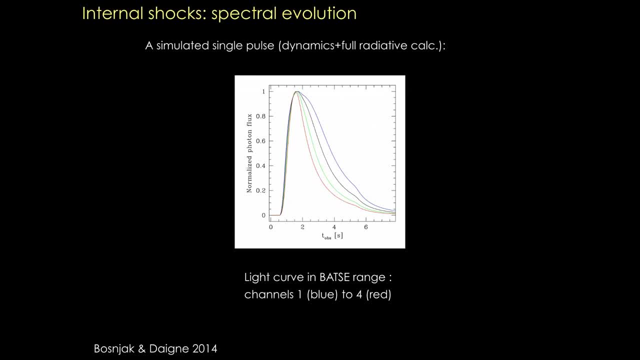 and we expect the synchrotron radiation to move towards a softer region. so here I show an example of a synthetic pulse computed with the same model as before, and I show the light curve in different energy ranges. blue is at low energy, red is at high energy. 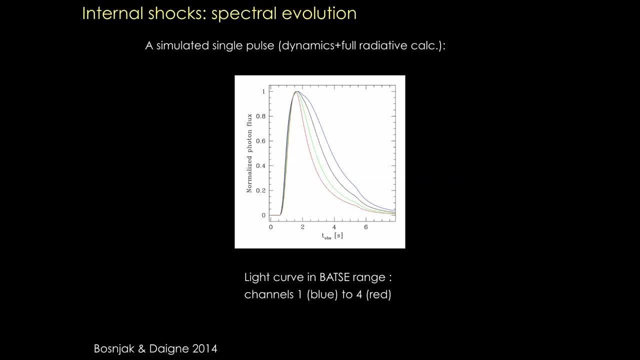 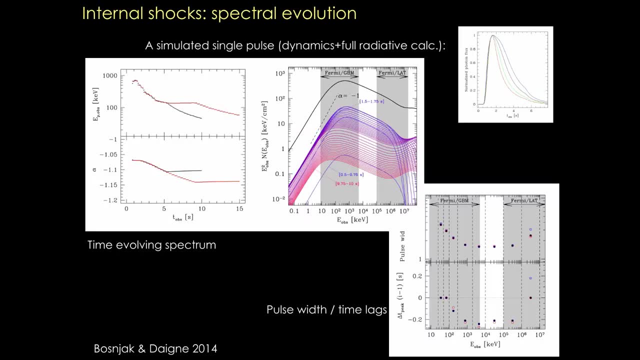 and you see clearly that the pulse shape is not the same. it's smaller at high energy and it's broader at low energy, and this is in agreement with observation. and here I show some details. here this is the evolving spectrum corresponding to this pulse, and here this is the evolution. 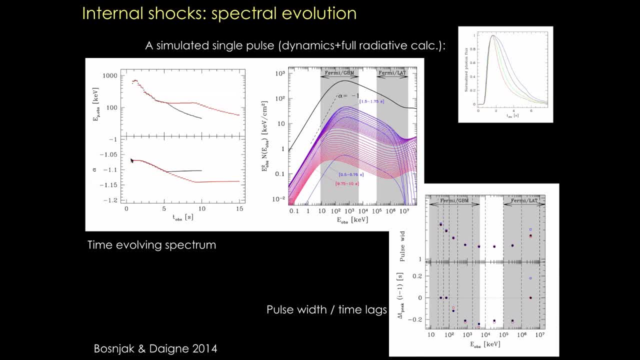 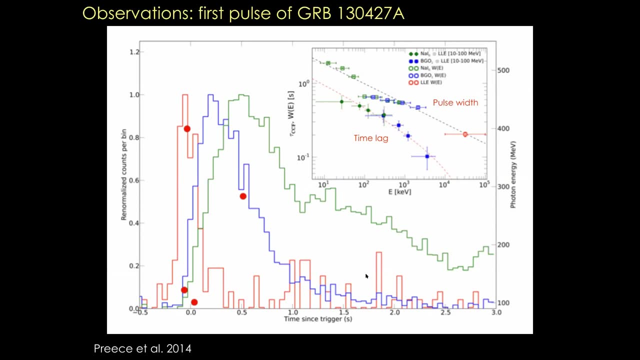 of the peak energy during the evasion and also the low energy flow. as I don't have time, I will not comment this figure, but there are other properties that can be tested in a few very bright camera rivers. here it's an extreme case where we can really make. 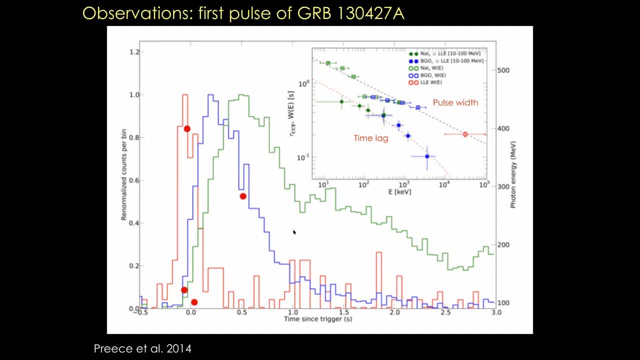 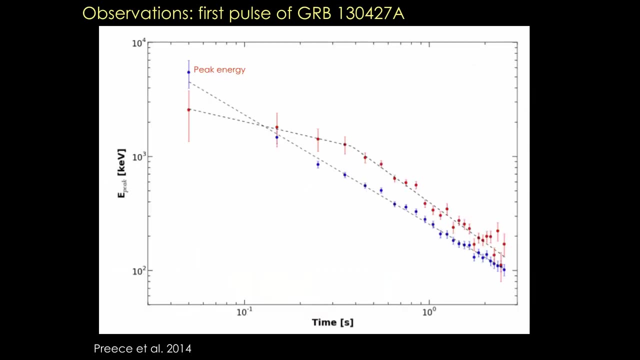 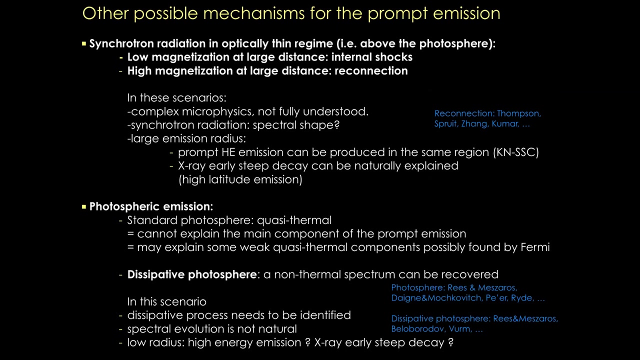 time-resolved analysis of one pulse and compare with such detailed calculation and I can say that the tendency is really well reproduced by the model. the details of the slope of the evolution of the peak energy, for instance, are not fully reproduced. now general discussion about the prompt emission. 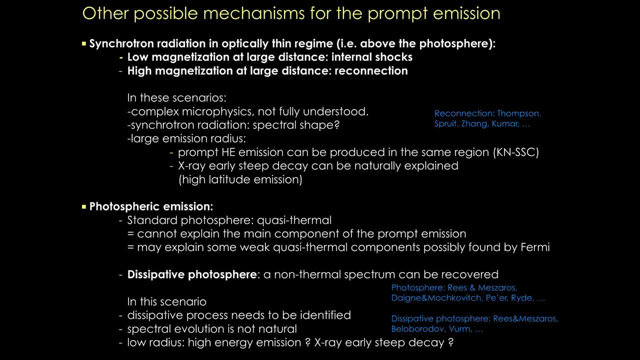 here I have shown the simplest model: internal shocks. but there are other possibilities. so either you consider that the prompt emission is produced above the photosphere in the optically seen regime and probably by synchrotron radiation, then either you have to consider internal shocks, like what I just did. 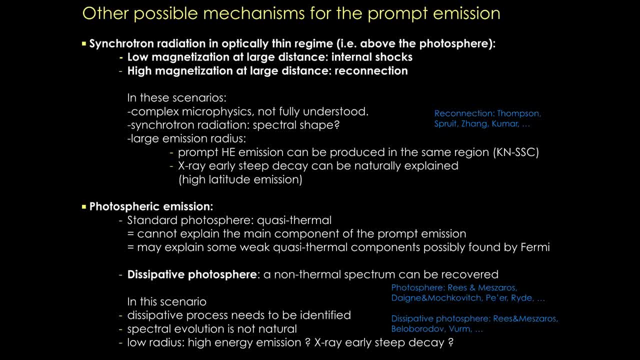 or if the magnetization is still high. you have to deal with reconnection in both cases to the complex microphysics at the plasma scale in the relative sixth regime. there are also some debates about the capacity of synchrotron radiation to reproduce perfectly the soft gamma ray spectrum. 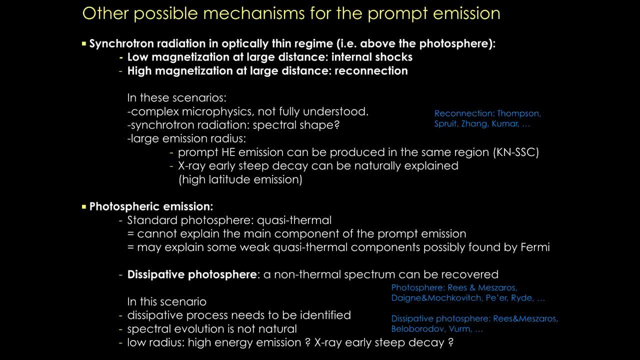 and especially the low energy slope. I will discuss that in one slide later. a nice property of this first class of model is the fact that the radius is high. we are above the photospheric radius, so the high energy can also, the emission can also escape, and so in such model 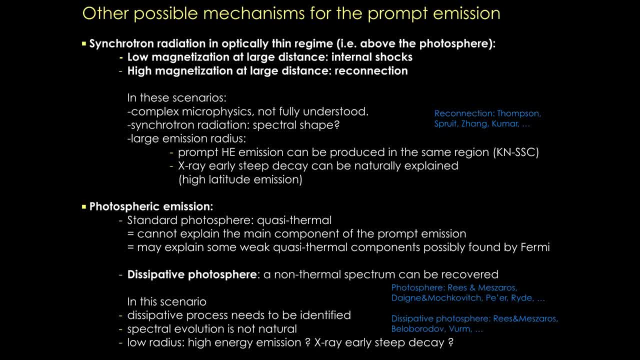 you can produce both the soft gamma rays and the high energy gamma rays in the same place, and another nice property is the fact that, as the final radius in this phase is high, you can also reproduce naturally the transition which is observed in X-rays between the prompt emission. 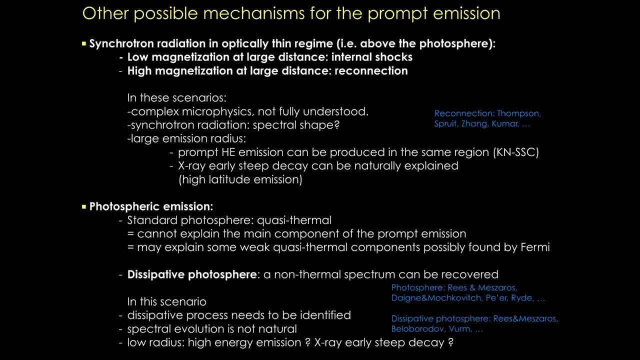 and the afterglow, which is called the early steep decay, if you rather prefer to believe that the prompt emission is produced by at the photosphere when the ejecta becomes transparent, which is also a very natural idea. the first one is natural because the source is highly variable. 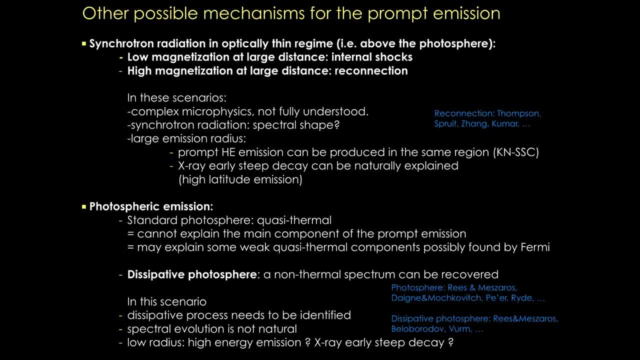 so you expect shocks, for instance. and the second one is very natural, because when something becomes transparent, you expect radiation. if you consider a purely standard photosphere, the result is a quasi-sermal spectrum which is not in agreement with observed spectra, except for a few cases, so it's not a good model. 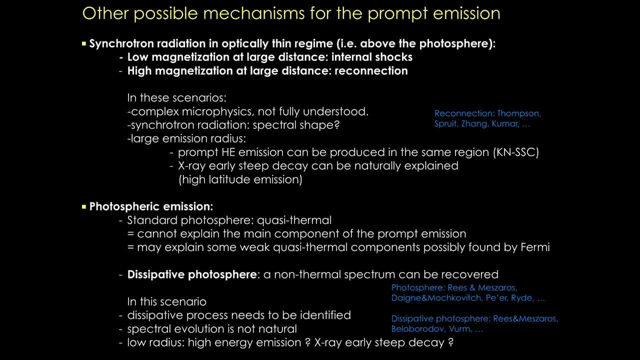 but it's something to consider if you want to reproduce, for instance, weak quasi-sermal components which are maybe identified by Fermi-GBM in a few bright bursts. but if you want to produce the main soft gamma ray emission with a photosphere, you have to consider a more complicated model. 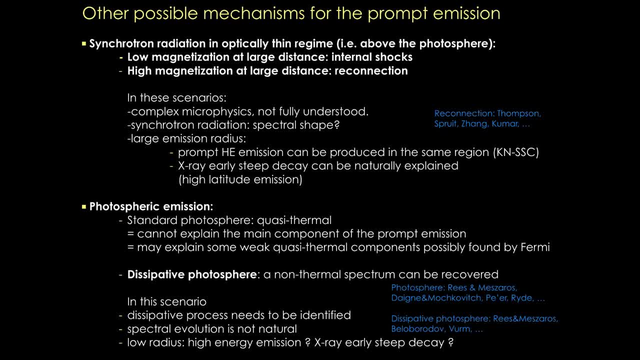 which is called a dissipative photosphere, where you have some dissipation process just below the photosphere, for instance internal shocks or reconnection, and then, when the medium becomes transparent, you have non-sermal electrons in the medium. so you have not only thermal radiation but also some synchrotron radiation. 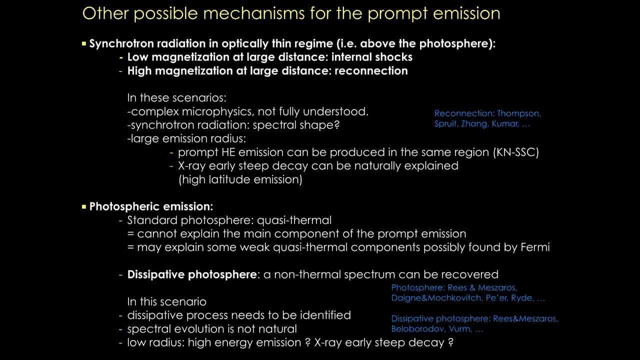 and some inverse-compton scattering. it's now inverse-compton scattering in the regime of high optical depth, so you have a comptonized high energy component which appears and with that you can also produce a non-sermal spectrum, as observed. there are also open issues. 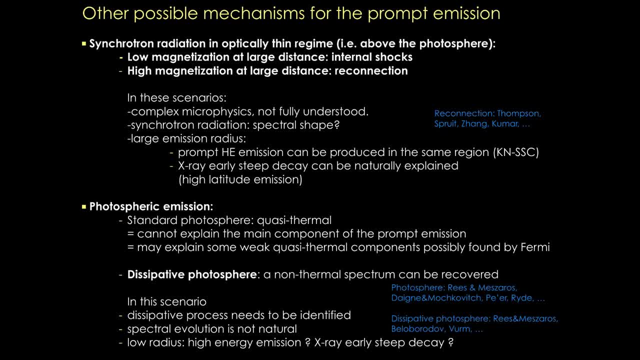 for this scenario. for instance, you need to identify the dissipative process, and it's not very clear if this scenario can naturally produce the same kind of spectral evolution that is observed. and another question is the fact that in this model the radius of emission is much lower. 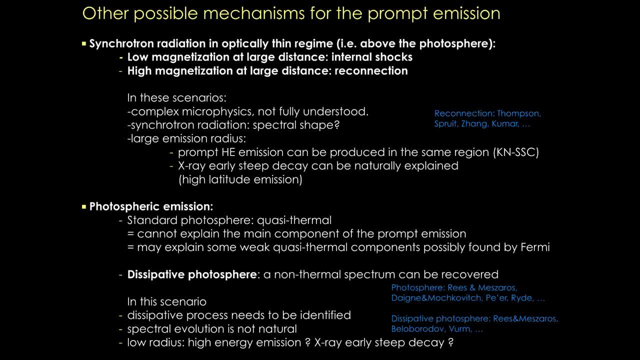 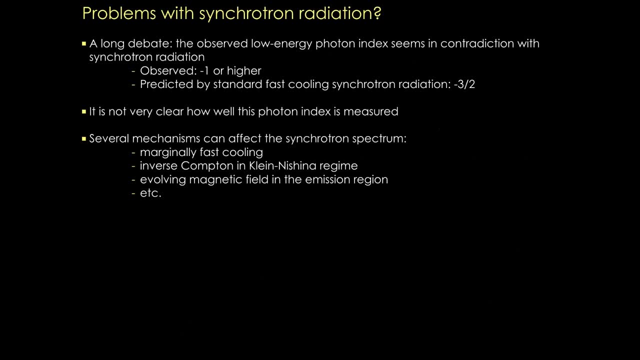 so you have probably to invoke to produce the prompt high energy emission or to explain the X-ray early state decay emission. so I will just show briefly some discussion of some of these points about the low energy slope of the synchrotron spectrum. it's a very complex question. 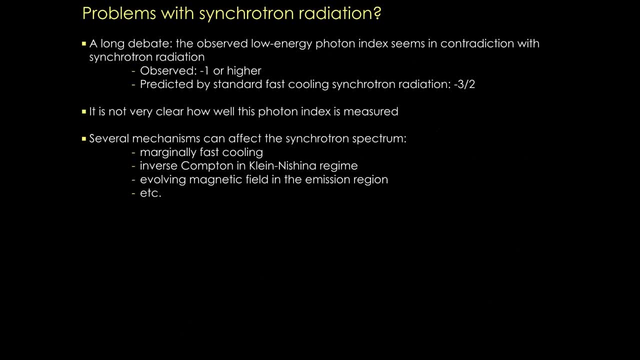 it's true that the pure synchrotron spectrum produces in the regime of high efficiency photon index, which is rarely observed. usually the index is above that minus one or even higher. but there are a lot of debates about the capacity of well measuring this photon index in data. 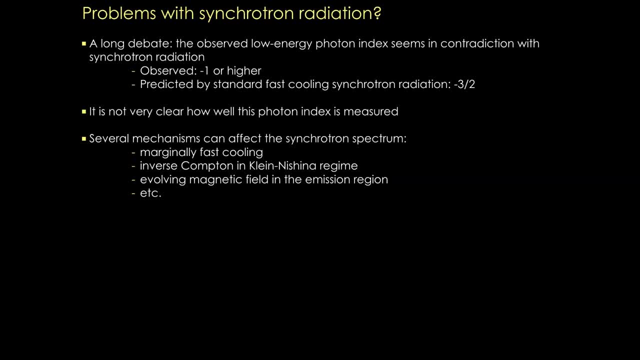 and there are a lot of theoretical possibilities- I am listing a few of them here- to change this low energy slope of the synchrotron spectrum. if you include additional processes like inverse compton scattering and so on, so it's a complex question which is highly debated. 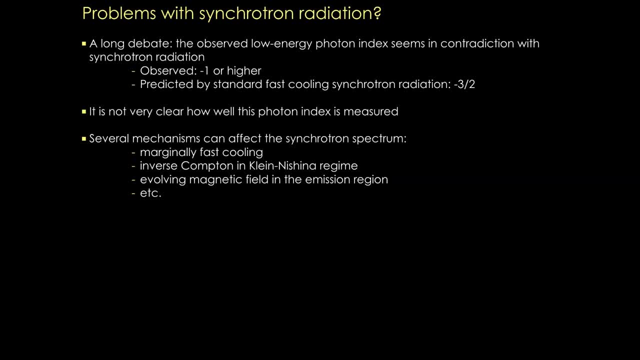 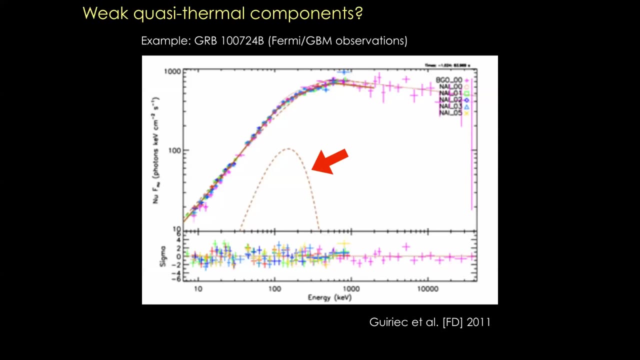 in the committee- and I belong to the sub-community- believing that we can find an agreement. but there are also strong advocates of the opposite opinion. here I show an example of a bright gamma-ray burst oxide like Fermi, where there is maybe a quasi-thermal faint component. 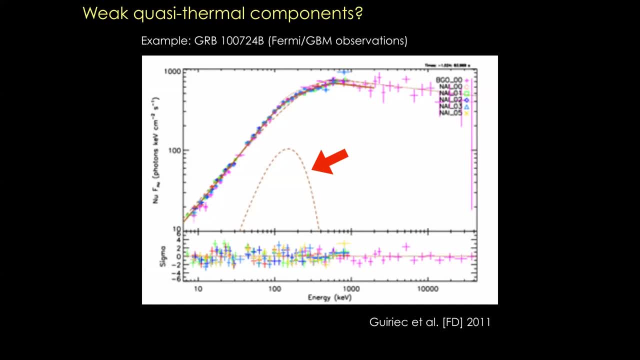 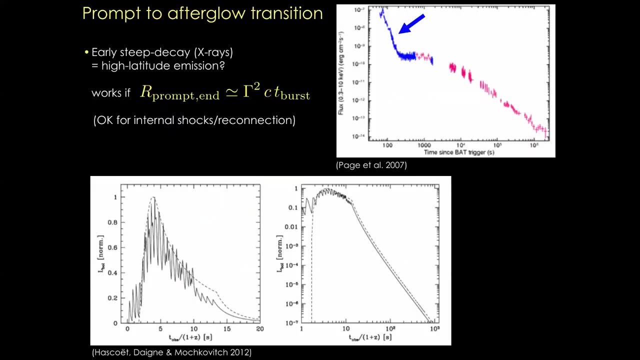 it could be a signature of the photosphere and it would say that the photosphere is not very hot, which would probably mean that a large fraction of the initial energy was not thermal but magnetic, which is in agreement with most ideas about the relativistic ejection. 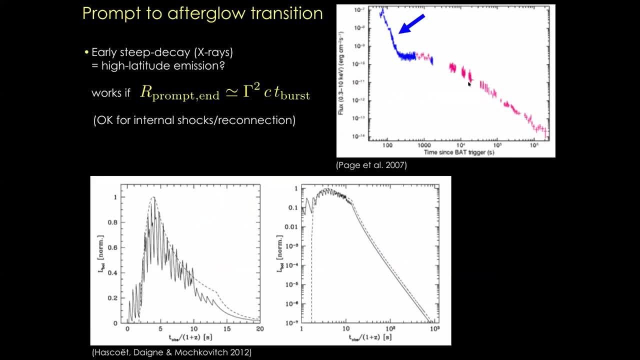 here I show an example of a transition between the prompt emission in blue here and the standard X-ray after blue here, and you see that there is a very steep decay at very early times. the early steep decay has a natural explanation which I think was proposed by Kumar. 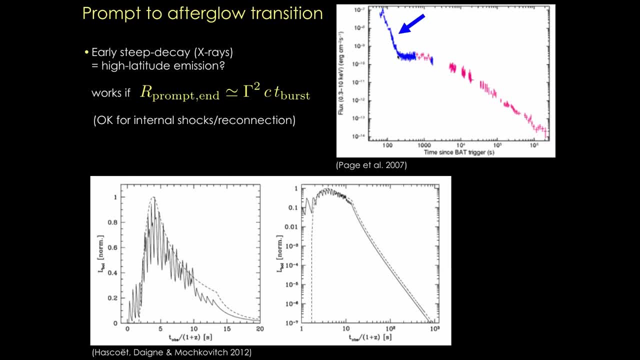 I should have mentioned his name here, Bhagwan Kumar, and the idea is the fact that when the prompt emission stops, you first receive the last photon emitted on your line of sight and then you will have photons coming from higher latitude, but the corresponding emission is much fainter. 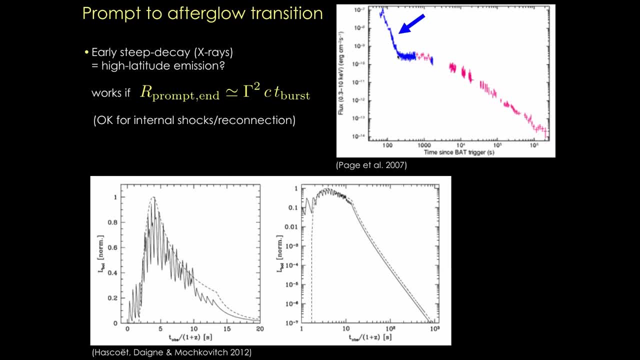 due to the relativistic beaming of the Doppler, the relativistic Doppler factor, and you can compute that and it produces naturally a steep decay with a slope close to minus 3, as observed, under one condition, which is to have a final radius for the end of the prompt emission. 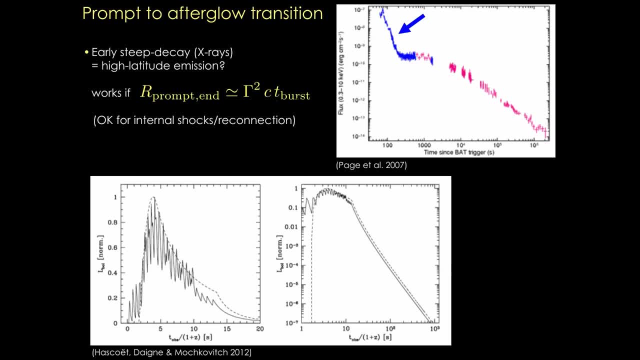 which is of the order of this estimate: gamma square C times the total duration of the burst and from the calculation I did before, it's a very natural expectation for internal shot. it's also probably natural for reconnection models. it's not natural at all for photospheric models. 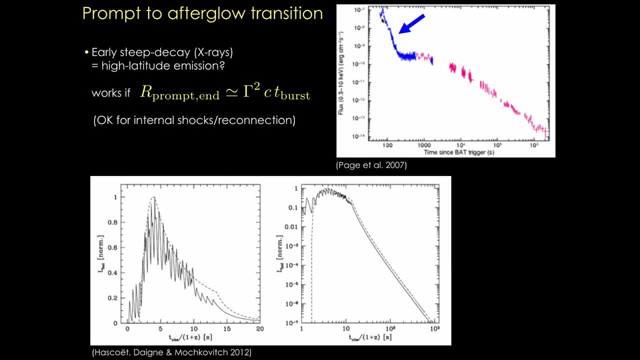 where the radius is much lower. so in photospheric models this steep decay cannot be produced by high latitude emission. it has to be a signature of a universal behavior of the central engine. at the end of the ejection it says something about the way the central engine is switching off. 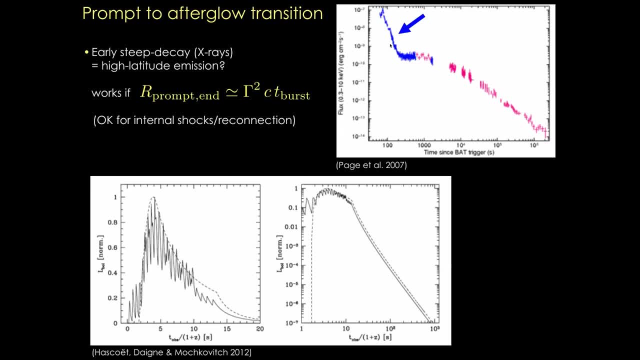 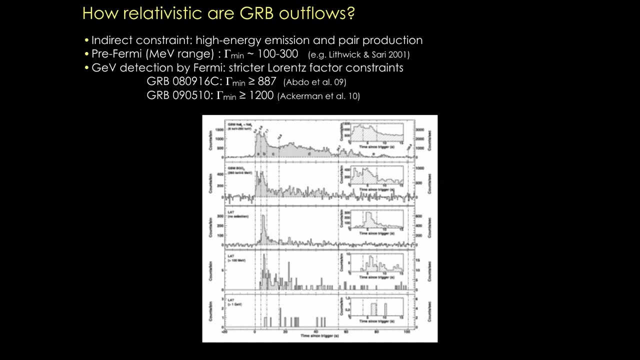 and this feature is really common. I think it's in more than 90% of bursts that it is observed. so here I show a simulation of internal shocks with a variable burst and an early steep decay with a right slope compared to this one, as time is running. 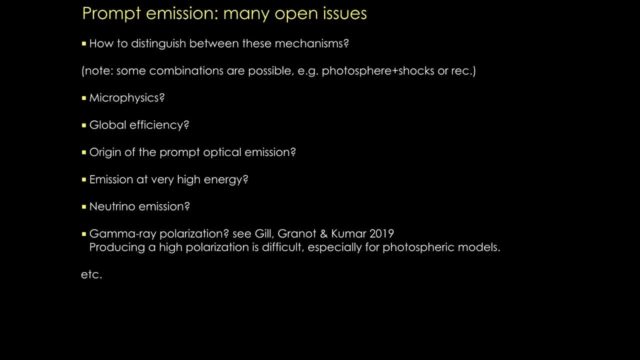 maybe I will skip that and I will end the discussion about the prompt emission with this list of questions, and we could discuss hours each of these questions. there is a lot of very complex physics behind, so I already mentioned, for instance, the microphysics, the global efficiency of the process. 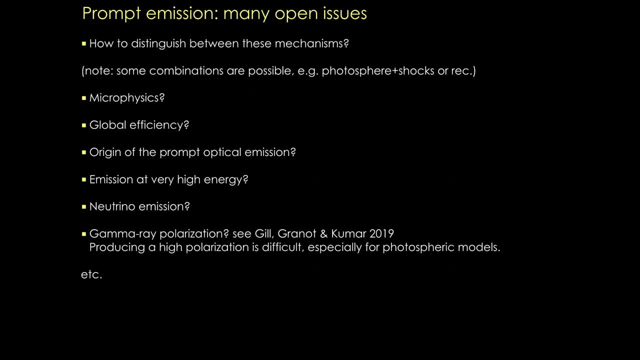 may be an issue: the origin of the other components, the prompt optical emission or the very high energy emission I mentioned at the first lecture. should we expect a neutrino emission? it's possible. if you also accelerate hadrons in the emission site, then the interaction of hadrons 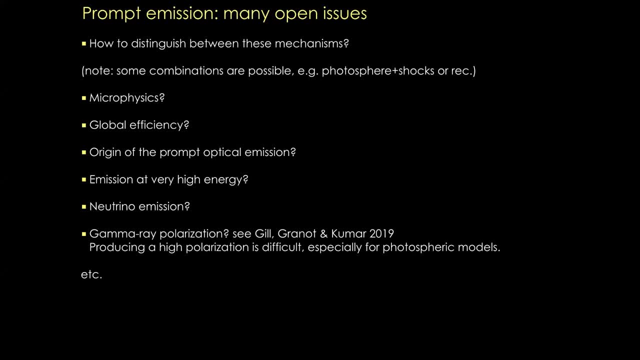 with gamma ray photons. how is it possible to distinguish between this mechanism that I discussed? one possibility would be to use a gamma ray polarization, so I will maybe say one word about that, because maybe there are some people working with astrosat who could be interested with this question. 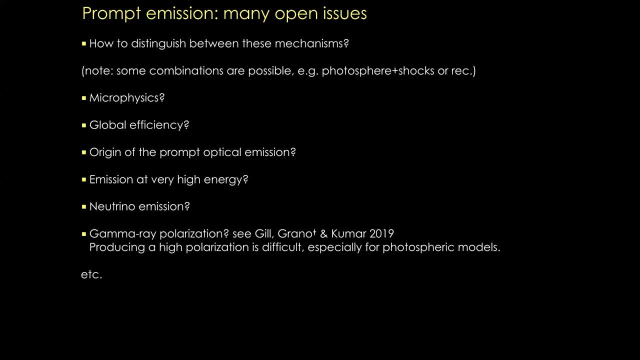 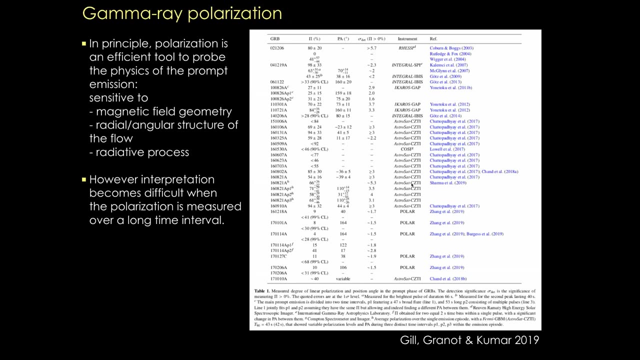 amongst the audience. I mentioned a very recent paper by Jill Granat and Kumar which makes a very good summarize of what is possible with gamma ray polarization for comparison with models. so in this paper they list all measurements which are available and one difficulty is that a lot of measurements. 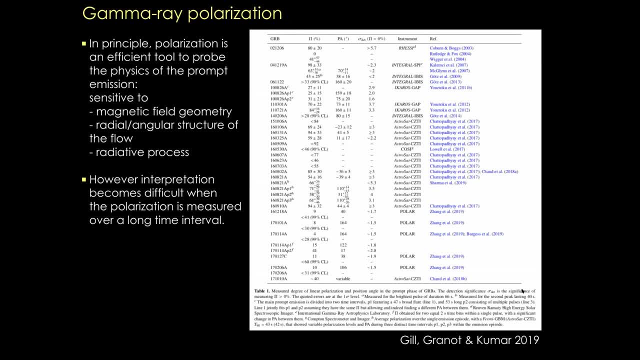 are made on a long time interval and this is a major problem for the comparison with models, because the idea is that, in principle, polarization is a good signature of several things like the magnetic field geometry. it's related also to the radial and angular structure of the flow. 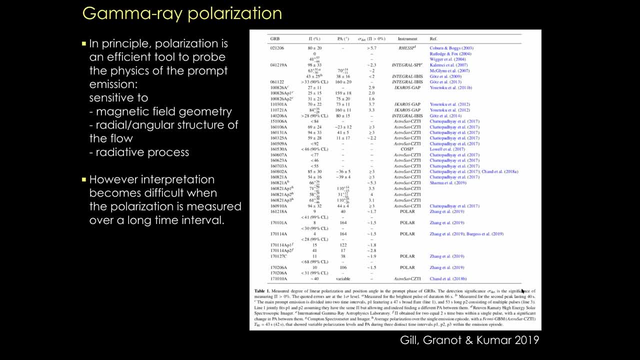 and it's also dependent on the radiative process. so it should help to distinguish between several models. but the difficulty is that once you average things over a long duration where you can have contribution from many different emission regions in the jet, then most cases would just predict a low level. 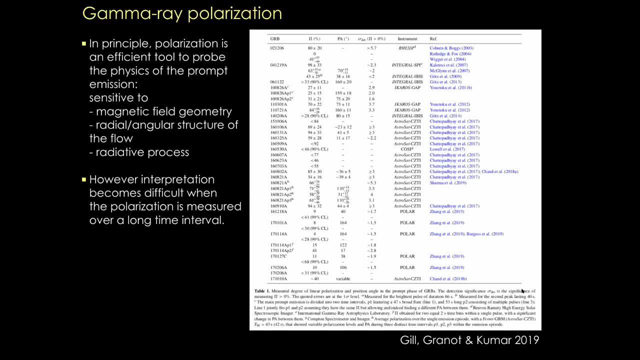 of polarization. so I would say that the measurement of a very high level of polarization in one case would probably eliminate a lot of models. but for the moment such high polarization were always very controversial, and if it remains at a level which is not too high, then it maybe starts to be difficult. 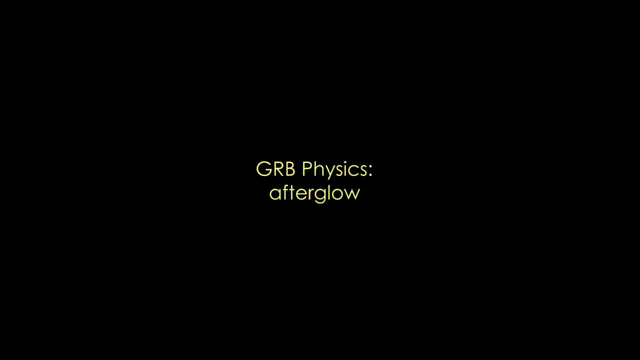 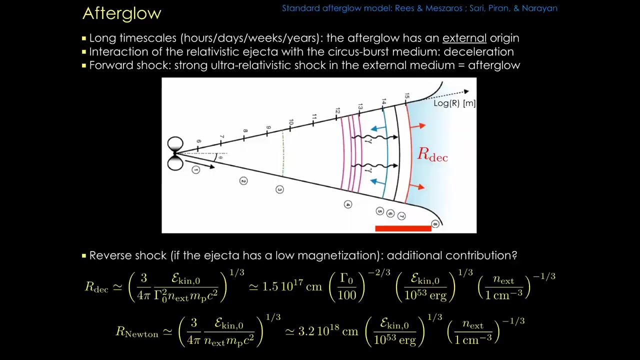 for photospheric models, but it's still compatible. so now rapidly a few words about the afterglow phase, if there are no questions about what I discussed on the prompt emission. so afterglow, here the standard model is very clear. the afterglow emission is due to a synchrotron radiation. 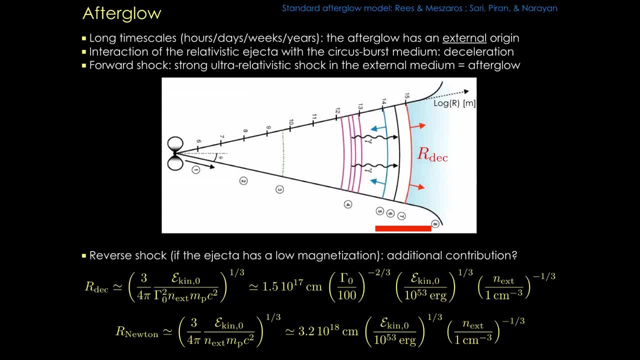 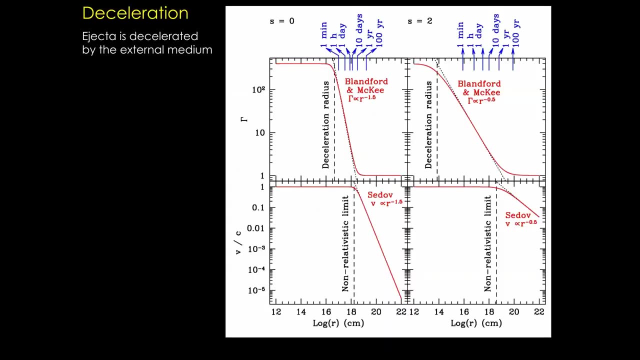 from shock accelerated electrons in the forward, shock propagating in the external medium due to the deceleration in the external medium and we estimated yesterday the corresponding deceleration radius where this process is starting. so I have shown that, which was the predicted dynamics and you see that there is. 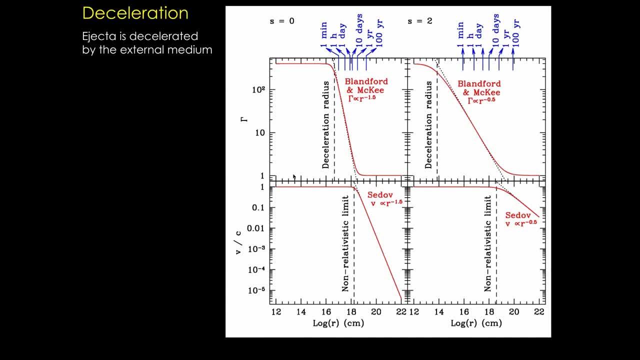 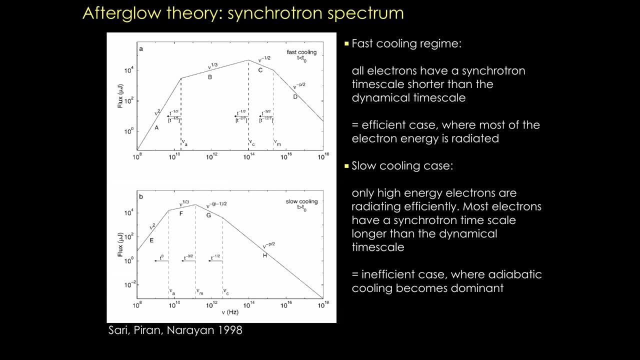 a power-low behavior for the dynamics which can explain the power-low decay of the observed afterglow flux. then to make a precise prediction you have to add the prediction of the spectrum, which has been done perfectly for the synchrotron process only by Sari Piran and Narayan. 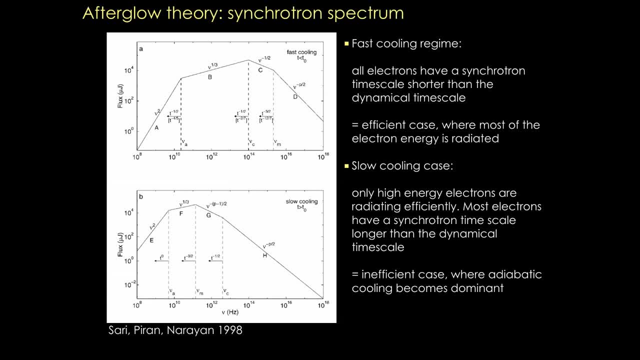 in 1998 and it predicts a non-thermal spectrum with several breaks. the idea is that among electrons you have two types of electrons. you have electrons with high Lorentz factor, where the synchrotron time scale is smaller than the dynamical time scale. 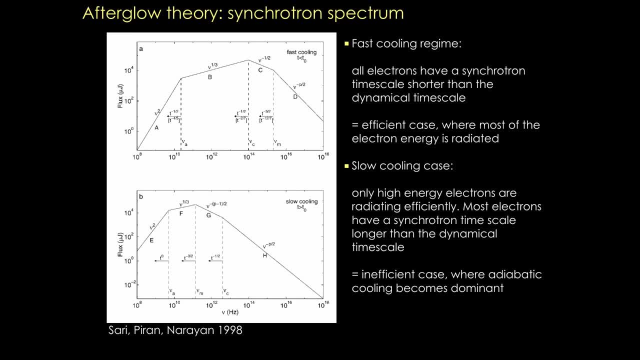 so these electrons will radiate efficiently, and electrons where the radiative time scale is larger, and then these electrons won't radiate efficiently. so if all electrons are radiating efficiently, we are in the so-called fast cooling regime, and it's a very efficient case, but it's expected only at very early times. 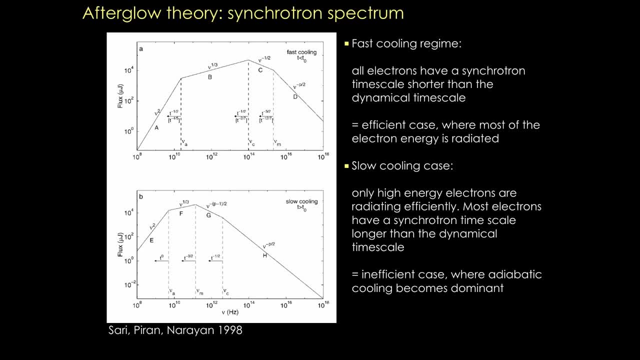 for the afterglow. on the other hand, this is the regime for the prompt emission. usually you are in the slow cooling regime, meaning that it's not very efficient and that most of the energy is in the cooling due to the spherical expansion, and so, if you convolve such a spectrum, 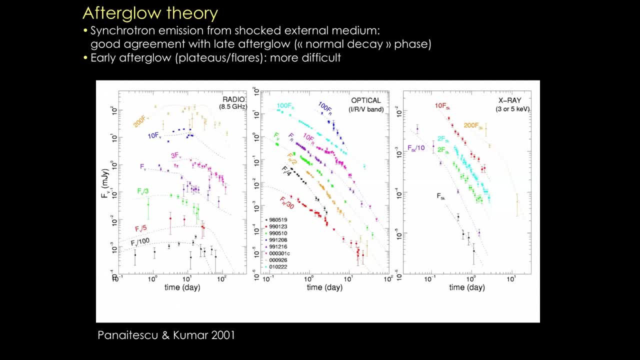 with the dynamics we have estimated yesterday, you can predict light curves at different wavelengths and for the late afterglow usually it works not too bad. here you have a whole paper where they fit well: the sample of afterglow in radio, optical and X-rays. 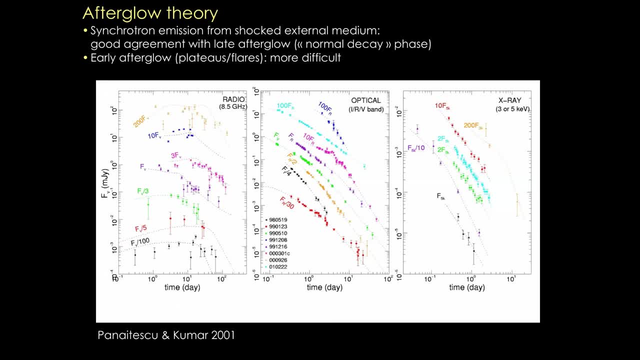 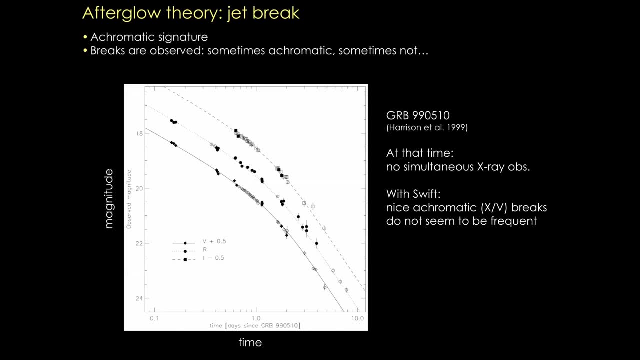 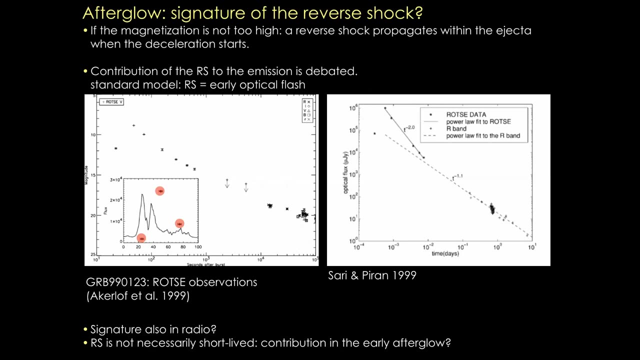 but then, if you look into more details, there are some problems with the standard model, so I will skip that. I have no time, I'm sorry. a good example, for instance, is a question of the signature of the river shock. first, to have a river shock, you need a low magnetization. 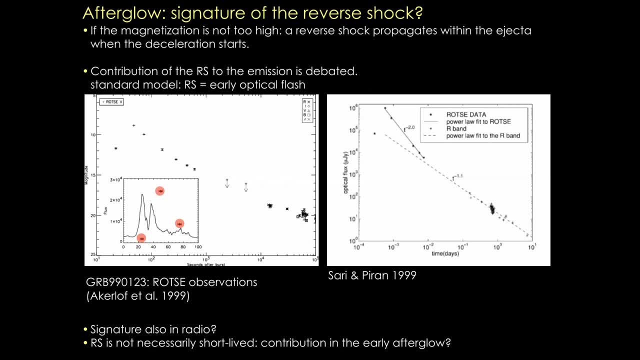 so it's important to try to identify river shock signatures, because they could say something about the ejecta. the river shock is propagating within the ejecta, and so the standard model is a contribution, mainly in optical and probably also in radio, which is short lived, which is, for instance, called an optical flash. 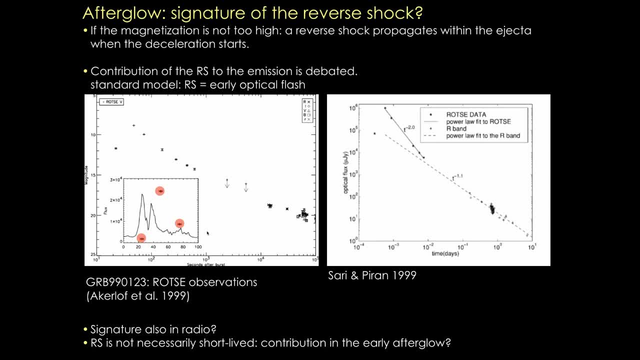 and historically it has been discussed first for GRB 990123, where there are these three measurements in optical during the prompt emission and as shown in this figure. these three points are well above the extrapolation of the optical afterglow and are well reproduced by the prediction of the 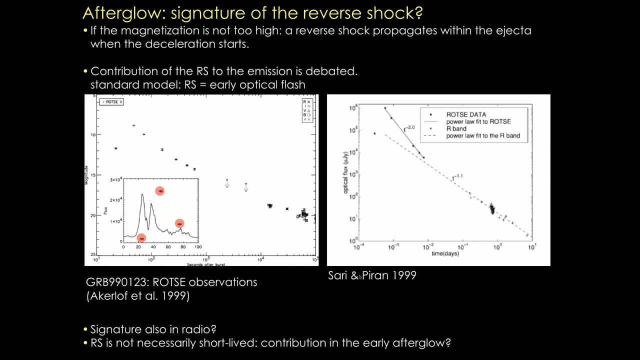 river shock emission. so this is a standard model. I see a few problems with that. first, if you consider more realistic radial structure in the outflow, the river shock is not necessarily short lived. and second, in many calculations the microphysics parameters which are used to feed data. 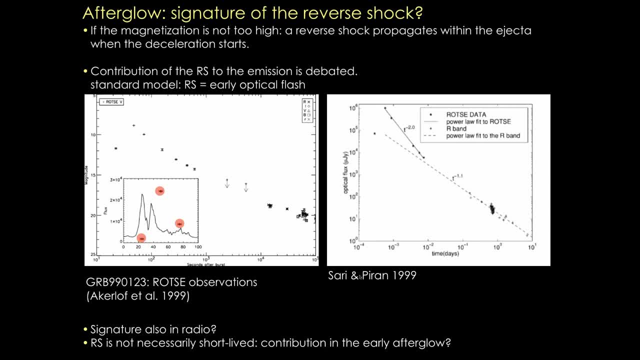 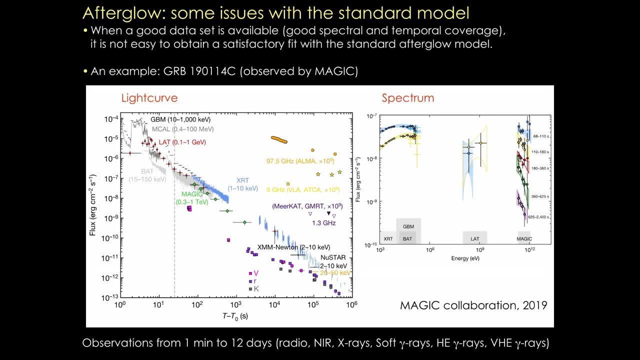 with the river shock would predict for internal shocks something which would be an extra emission and not a gamma ray emission. so there is some contradiction between the two interpretations. I see a good question that I will answer in a few minutes about the spin down of the neutron star. 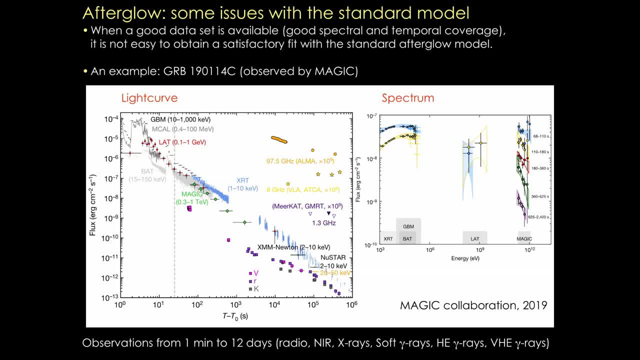 another example of problems we have with the standard model for afterglow is the fact that when we have a really good data set, often it's difficult to feed the data. here I show again the burst which was observed by magic. it's a good example because we have many, many observations. 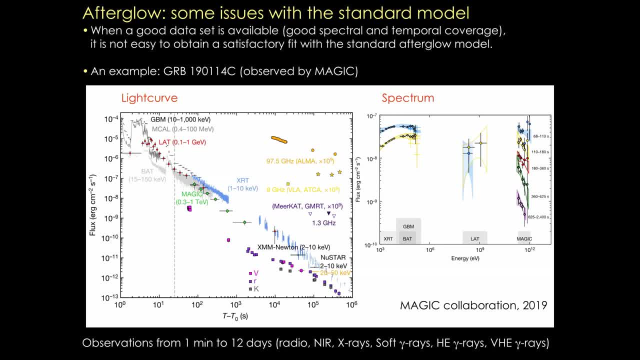 you see all the instruments here. so it has been observed from 1 minute to 12 days in radio, in near infrared, in X-rays, in soft gamma rays, in high energy gamma rays and even in very high energy gamma rays. so we have a very nice light curve. 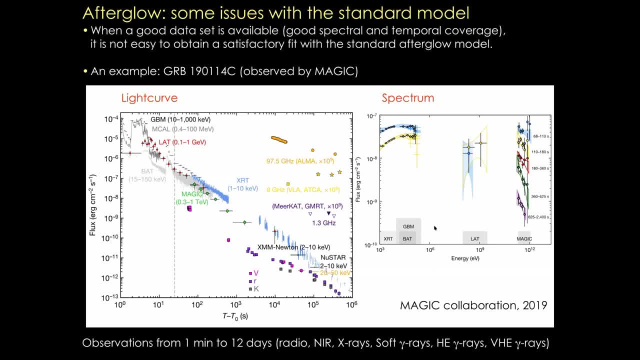 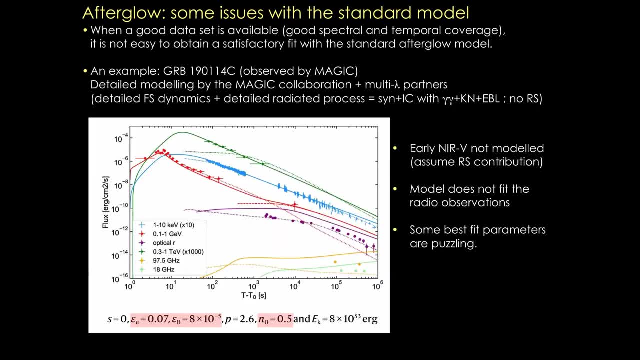 at different wavelengths and a very nice spectrum, and the magic collaboration in collaboration with associated multi-wavelength observers, has produced a very detailed modeling of this burst and you see the results. you see that they can provide a good fit, but they do not model the near infrared. 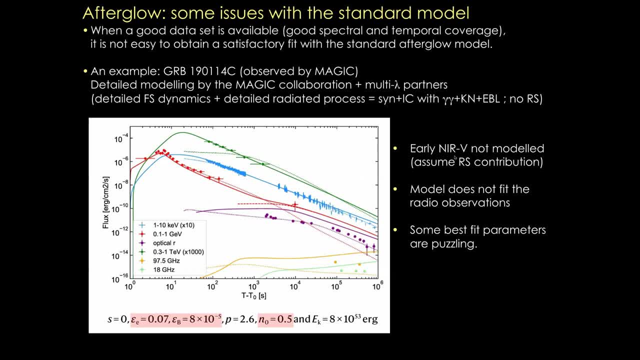 and visible emission at early times. so this is a reversal contribution. so another component, and it does not fit at all for the radio observation, which are the orange and green curves which are slowly rising, and it's very common to have difficulties to fit the radio observation. so it's puzzling. 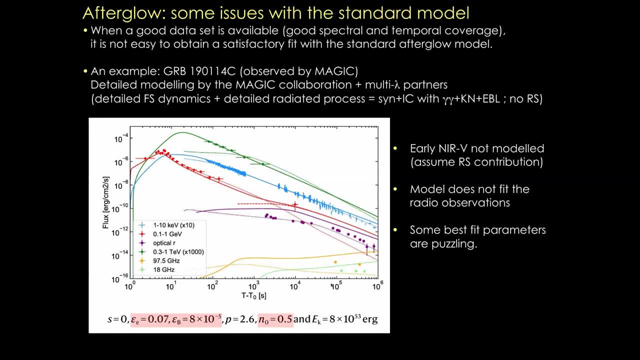 and, in addition, the parameters of the best fit are also puzzling. for instance, this burst is a long burst associated to the explosion of a massive star. the principal massive stars are in dense environments and the best fit parameter for the density of the external medium is 0.5 particles. 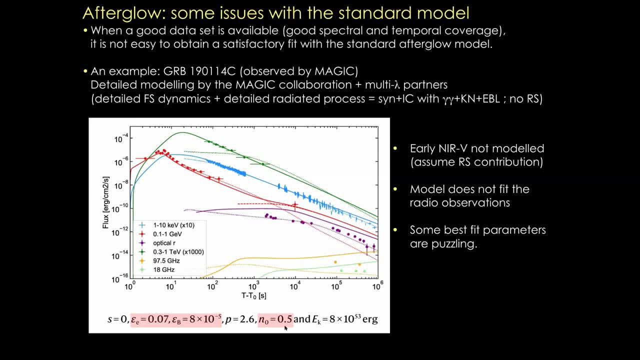 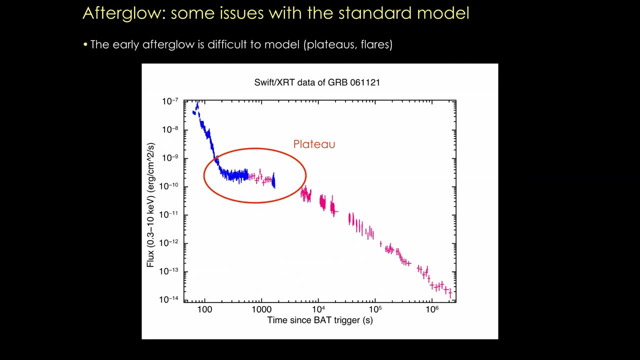 per cubic centimeter, which is very low. the value of the fraction of the magnetic energy is also very low. so there are things a little strange and in addition it's very difficult with a standard forward shock model to explain the behavior of the early afterglow. 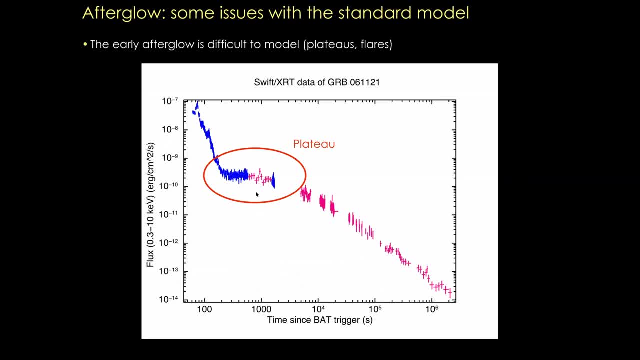 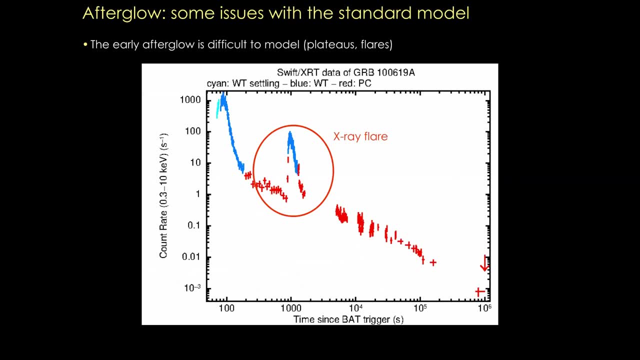 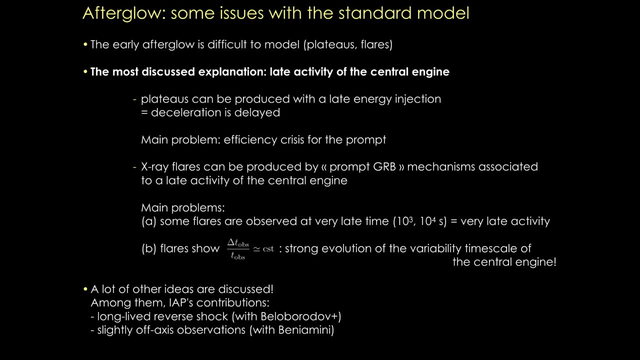 especially in X-rays. so, for instance, we see plateaus, like in this example, or we see variability like X-ray flares, like in this example. so there are ideas to reconcile the standard model with this behavior, and most discussed ideas are related to elect activity of the central engine. 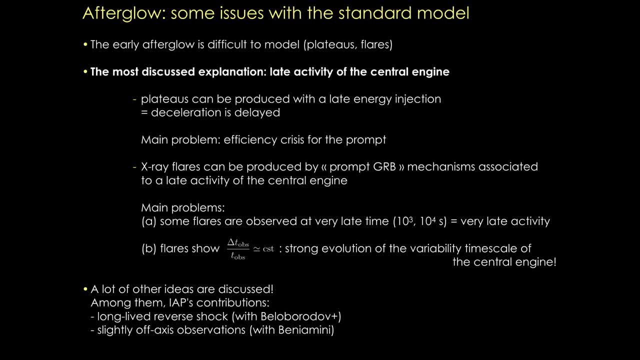 for instance, you can produce a plateau in the ejector. if you add some kinetic energy, you will delay the deceleration and get a plateau. and you can produce X-ray flares using the same physics and for the prompt emission, but associated to very late ejection times. 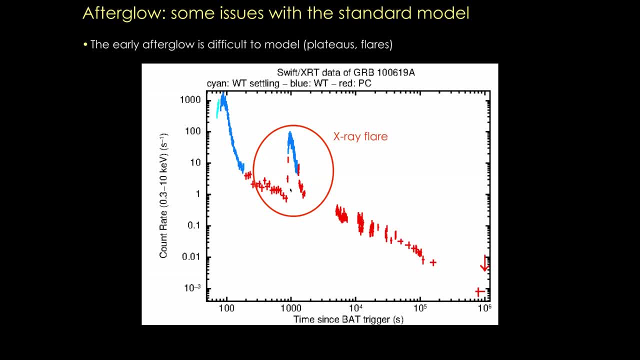 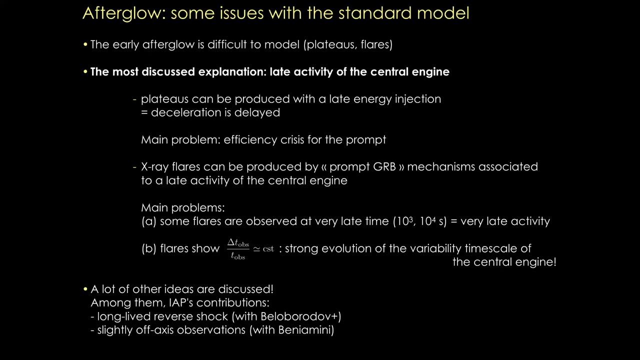 so that it produces very late emission, like here. but you see, if these are, for instance, late internal shocks, that the ejection occurred one thousand seconds after the initial event, so it's a very long lifetime for the central engine. it's a problem. so another problem is the fact that if you assume, 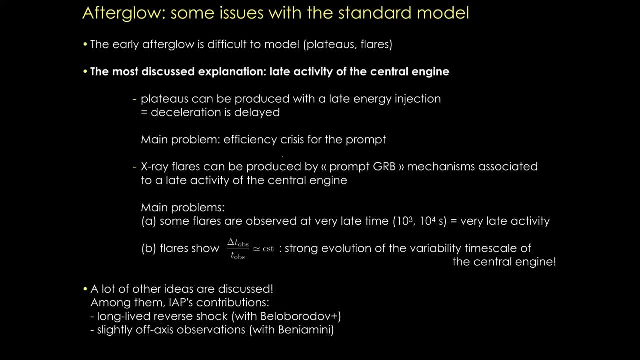 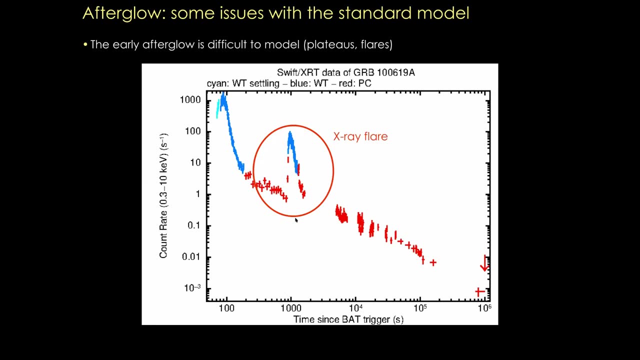 late energy injection for the plateau. it usually leads to a constraint on the prompt emission, which is very strict for the efficiency. you need very efficient prompt emission mechanism above 50% efficiency. in addition to the problem of the late activity, another fact is the fact that usually X-ray flare 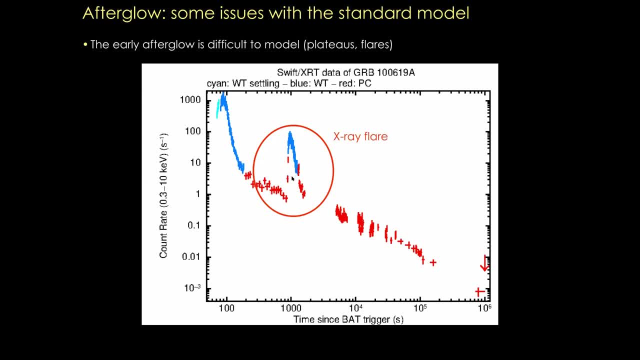 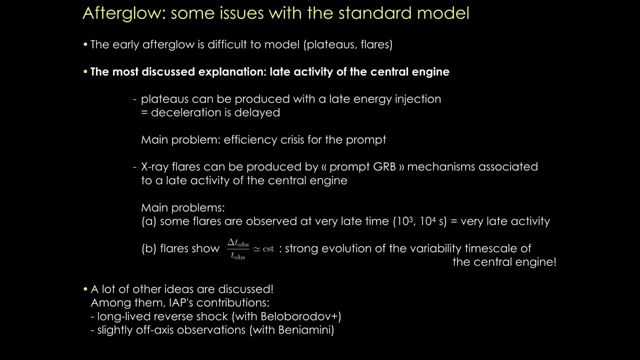 show always the same shape in log. log delta T over T is constant and it means, as the variability is related to the variability in the central engine, it means that the variability timescale of the engine is increasing linearly with time, which is not very natural. so there are a lot of other ideas. 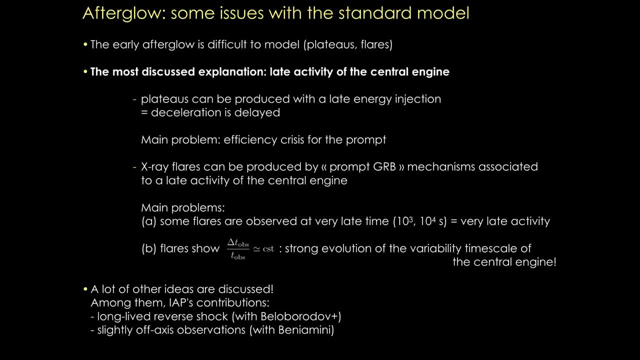 to list them, but I just mentioned that, for instance, in our group in Paris, we are trying to investigate two possibilities: one related to the radial structure of the ejection- the possibility to have a long lived reverse shock- and another one, inspired by 170817, is the idea to have a lateral structure. 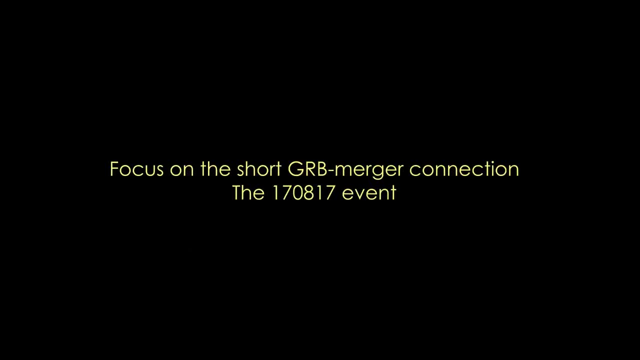 and to have a burst, which is seen slightly, of axis. ok, so this is the last for afterglow physics, but I try to show the success of the standard model, but also many open questions. and now for the remaining 15 minutes I would like to discuss. 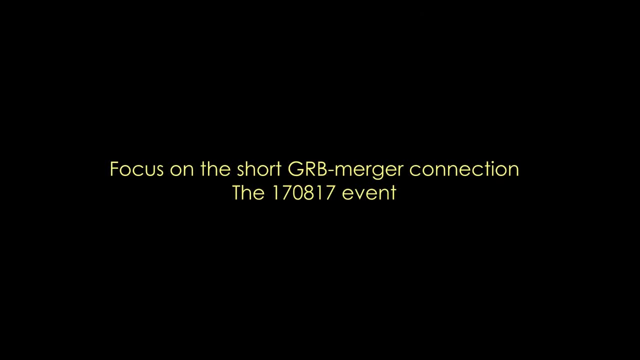 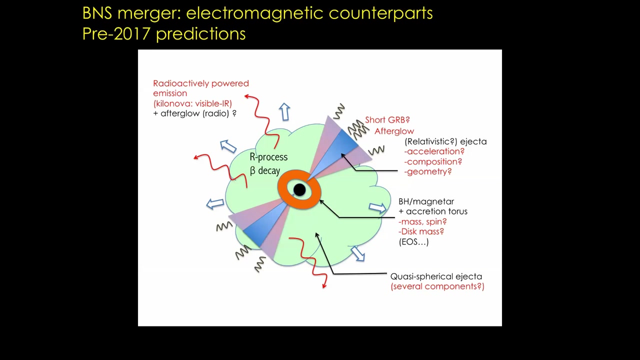 finally, 170817. there are no questions about it, so probably this event has already been discussed in other lectures, so I will go fast on the introduction. you know that you can expect to have a lateral structure of two neutron stars. you expect many counterparts because you expect. 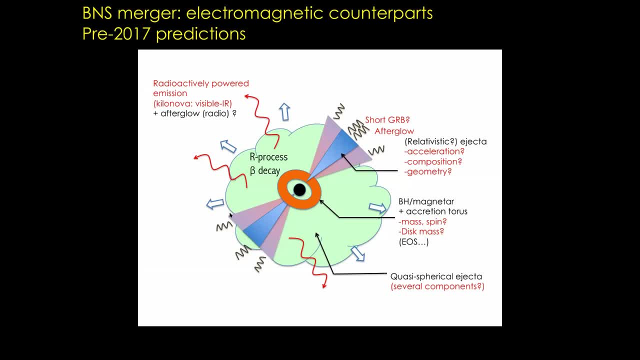 some dynamical ejecta producing a kilonova associated to radioactive elements produced by the rapid neutron capture process in this ejecta, and you can also expect electromagnetic counterparts associated to a relativistic ejecta related to the formation of a very compact object in the center. 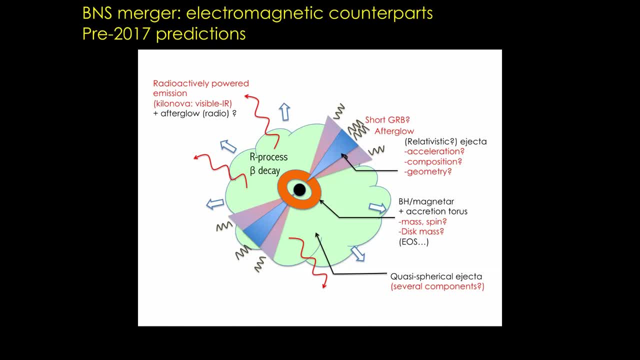 this is the physics of the gamma ray burst we have discussed in these lectures. notice that if the post merger evolution is complex- and this is an attempt to answer to the question about the spin down- and especially if, for instance, you have an intermediate phase where you have a neutron star, 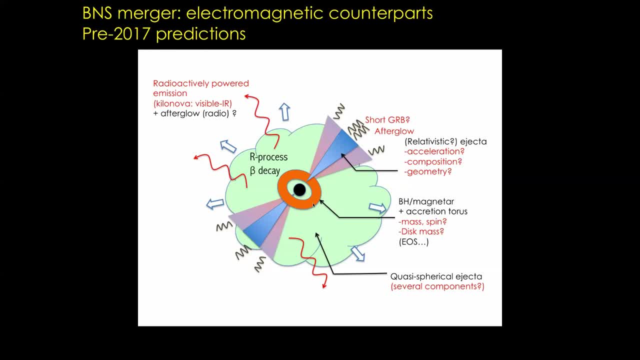 before collapsing to a black hole, you could have some delay between the relativistic ejection and the merger itself, as observed in gravitational waves, and you could also have an additional electromagnetic signature of the intermediate phase, where you have a neutron star. some groups have tried to estimate what could be. 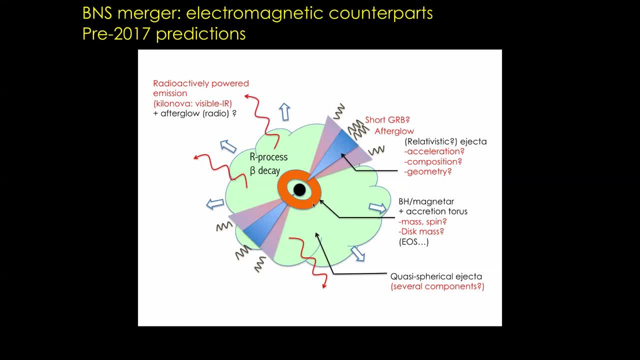 the contribution of the spin down of the neutron star to the emission and, for instance, have a hope to explain the plateaus which are observed in some bursts or the late X-ray emission which is observed in some gamma ray bursts. with this I would say that for the moment, 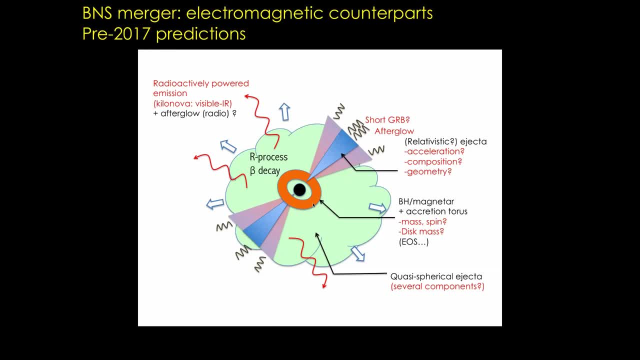 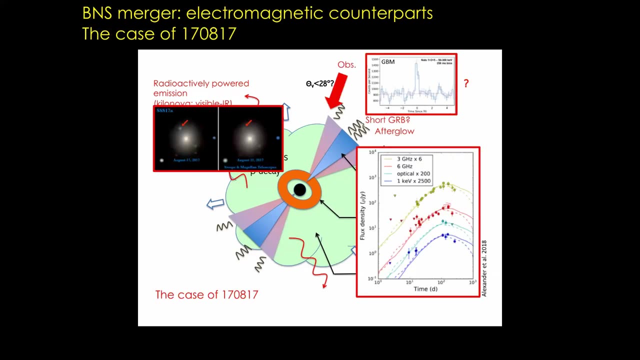 models are not very detailed and they should be coupled to a more detailed discussion of the radiative processes to be really convincing, but it's an interesting idea. I will skip that. and just everyone knows that in the case of 170817, all these counterparts were observed. 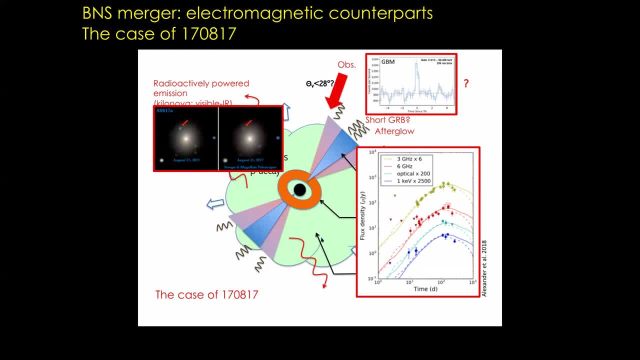 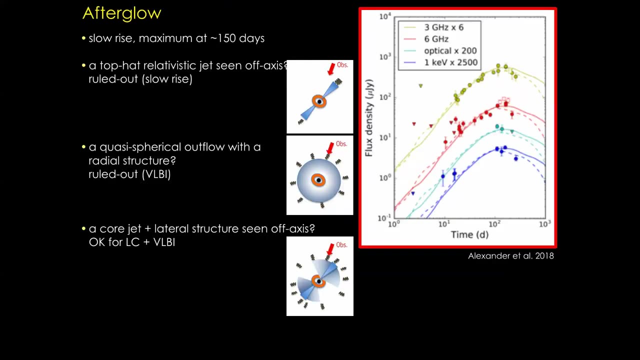 the kilonova, the gamma ray burst and afterglow. what I would like to discuss is the fact that the afterglow is unusual, but it can be understood why, and the short gamma ray burst is also unusual. so let's focus on the afterglow. 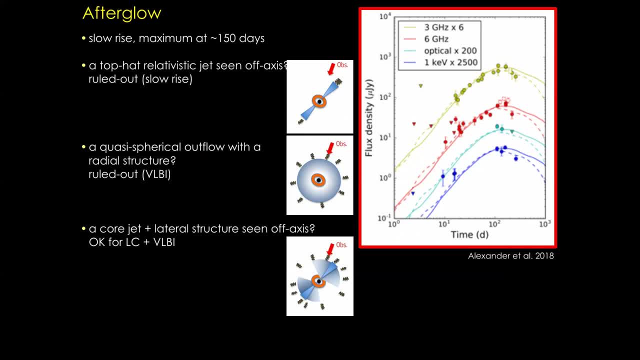 the main difference between the afterglow of 170817 and standard gamma ray burst afterglow is the fact that it has a very, very slow rise and the peak is reached only at about 150 days. it is illustrated with this figure, so in blue you have. 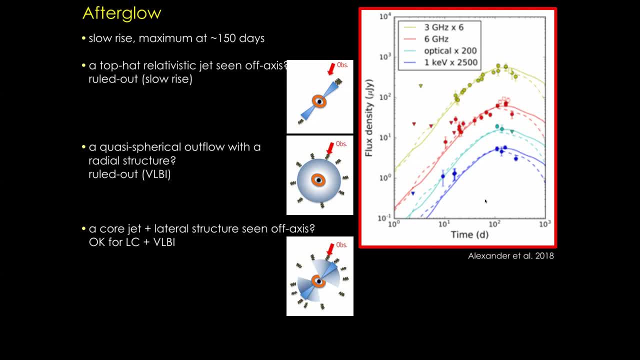 X-rays in red and yellow radio and in cyan. it's optical, and optical observation starts later because initially you are dominated by the kilonova emission. so you see a clear peak, which happens very late, from gravitational waves. we know that this event is not seen off axis. 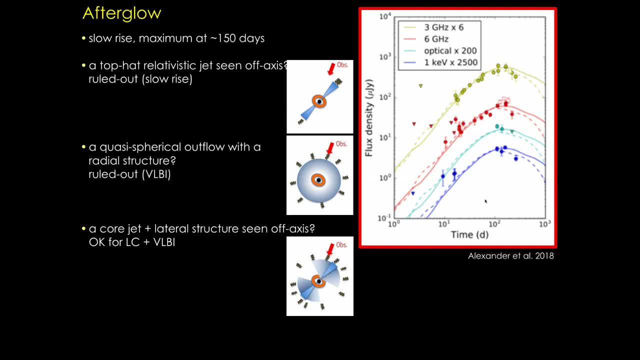 we are off axis. so the most natural explanation is to say: okay, it's a relativistic jet, like in standard gamma ray burst theory. so this is the first explanation. the problem with that is that it does not predict such a slow rise. the rise would be much steeper. 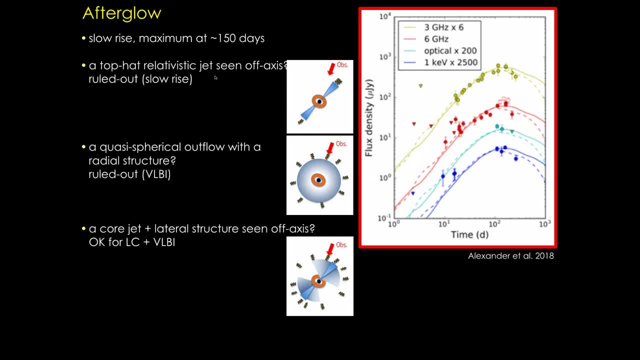 so then another idea would be okay. maybe the jet did not succeed to escape from the surrounding material, for instance the material associated to the blue kilonova. it's a shocked jet scenario. in this case, the gamma ray burst was associated with the interaction of the jet. 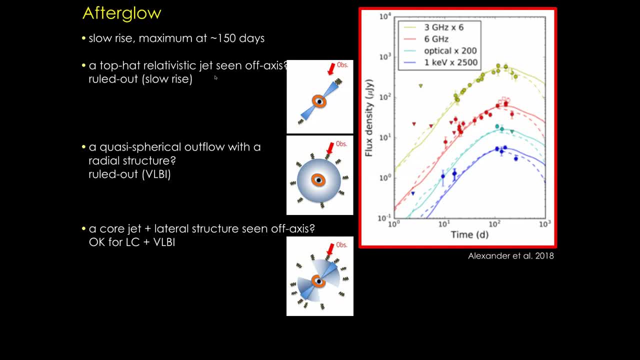 with this kilonova ejecta, a shocked breakout emission process, but the jet did not emerge and what we see is it's just a mighty relativistic ejecta which is quasi-spherical and which has a strong radial structure due to the interaction with the kilonova ejecta. 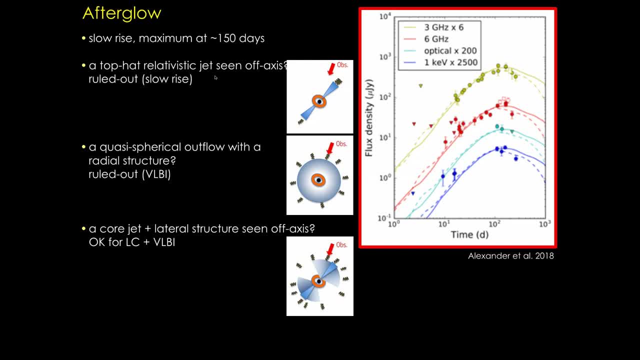 such a model can fit very well, but is now ruled out by VLBI, observations that I will show just after. and the last possibility is to come back to the previous idea but to say that the central core jet, which is ultra-relativistic, ultra-energetic, 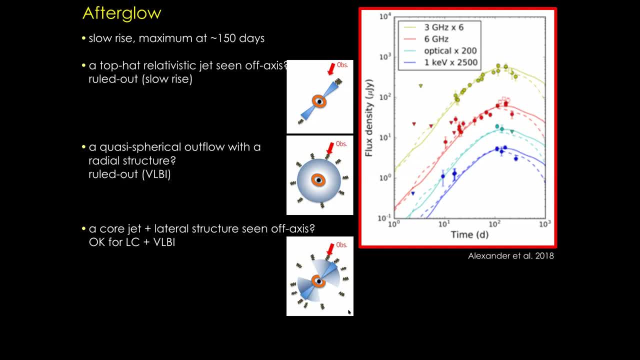 is surrounded by some material. it's a lateral structure. and one possibility to produce this lateral structure is, again, the interaction between the jet with the kilonova ejecta, in a case where it is successful, where the jet can escape. so in this case, the lateral structure. 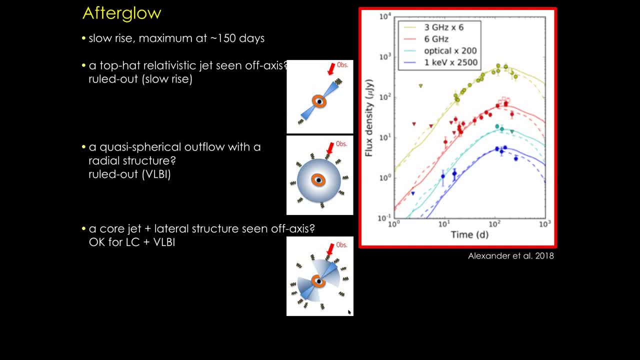 is often called a cocoon, but there are some other possibilities related to the mechanism of relativistic ejection itself to produce such a lateral structure. so I won't use the name cocoon, I will say lateral structure, because it's more general. so the idea is that 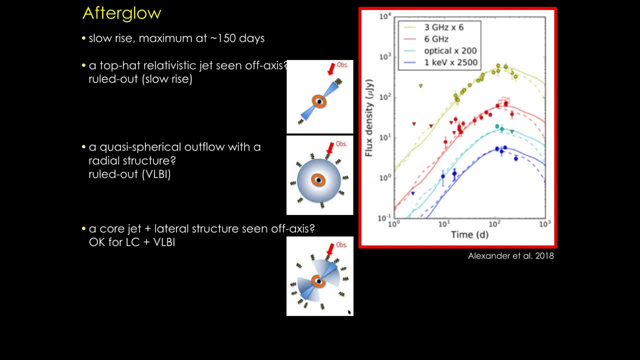 if something is highly relativistic, you see only the material which is pointing towards you because of the relativistic beaming. and this material is only mildly relativistic, mildly energetic. so you see a faint emission and then, due to the deceleration, the Lorentz factor. 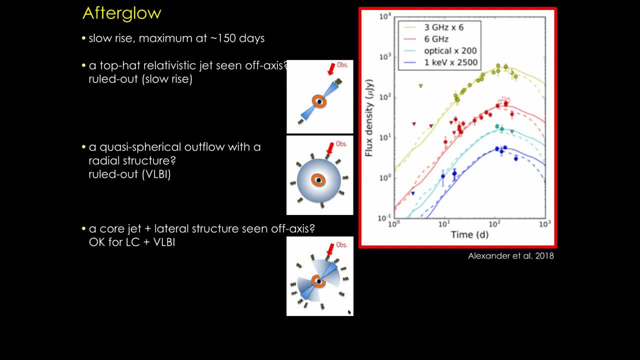 is decreasing and then the opening angle of the relativistic beaming 1 over gamma is increasing. so you see a region, an emitting region, which is larger and larger, and you start to explore regions which are closer to the central axis, so you see regions which are more relativistic. 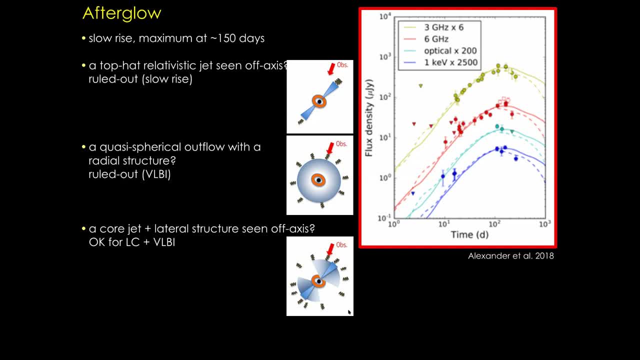 more energetic and you see a higher flux and the peak is reached when, for the first time, you see the entire ejecta, including the core jet. so it's very nice because it would mean that for the first time we see such a jet of axis and for the first time 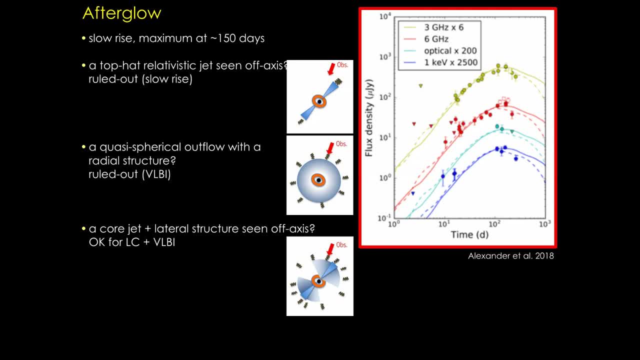 we can reconstruct the full geometry of the ejecta, and this scenario seems to be confirmed by VFBI Resmi. could you just confirm that you are still hearing me, because I have maybe an internet connection problem. do you hear me? ah, is the connection lost? yes, I can hear you. 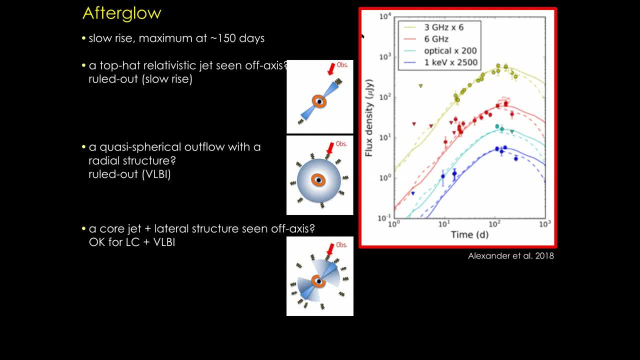 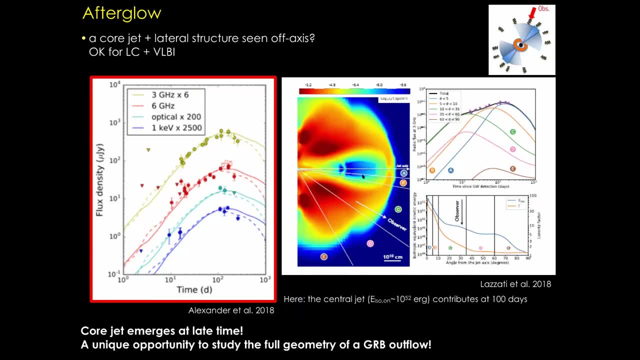 ok, sorry, thank you, because I have maybe an internet problem. no, you are fine. ok, thank you. so I show now an example of a simulation of the propagation of a jet in an ejecta producing a cocoon, and here you see the construction of the light curve. 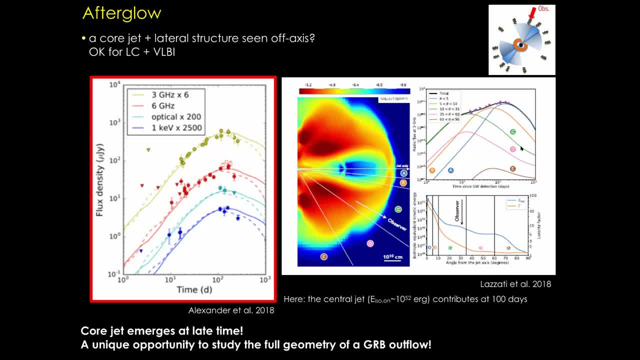 initially, at early time, you are dominated by the contribution of the sea region, which is an off axis region which is pointing towards the observer, and then, at later time, because the relativistic beaming is less efficient, you start to see the B region and, at the peak, the L region. 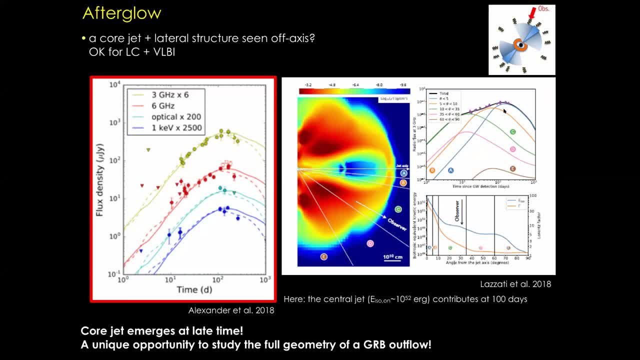 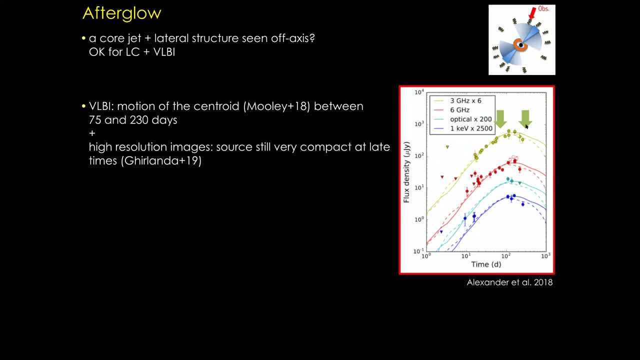 which is the core jet. so it's a very nice explanation. it works very well. and then it has been confirmed by VFBI observation, because at these two epochs indicated by the green arrow, there are VFBI observations and they show a proper motion. you see that there is a 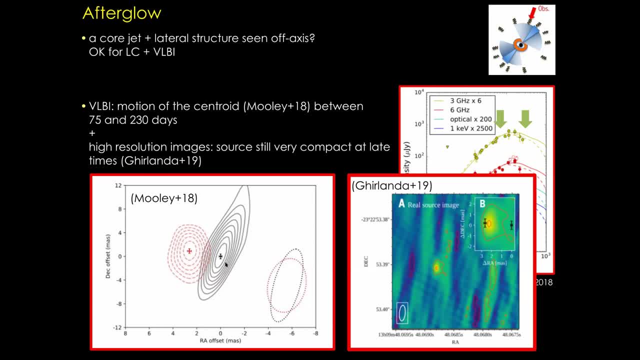 displacement of the centroid of the emission between the two dates. and when you compute the apparent velocity, it is superluminic. so it's a clear signature of an intrinsically ultra relativistic motion. so there is a jet and in addition other VFBI observations. 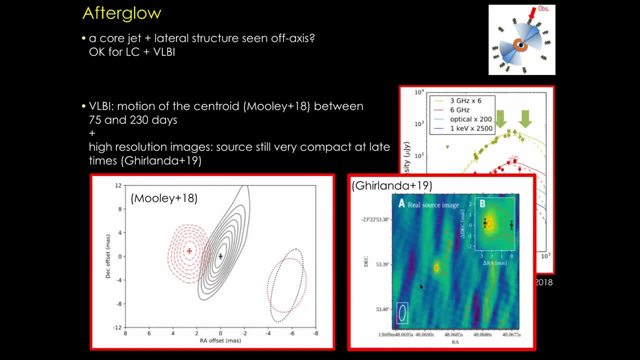 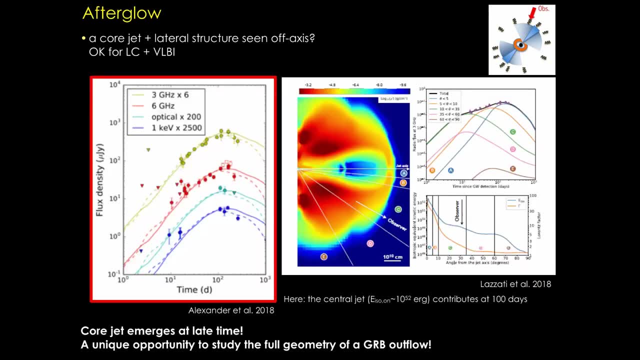 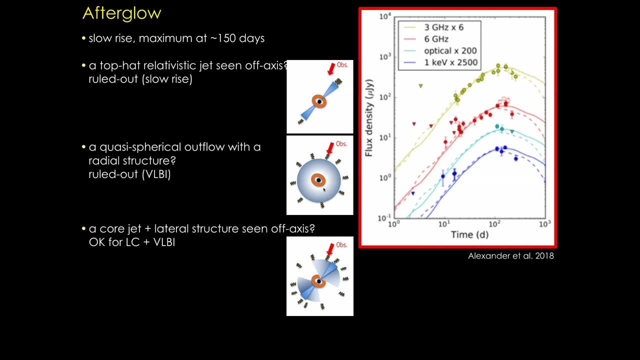 by a European group have shown that even at late time the source is still very compact. it cannot be resolved and it's not compatible with the scenario where it would be such a quasi-spherical ejecta expanding. it would be resolved at late time. so it's compatible with. 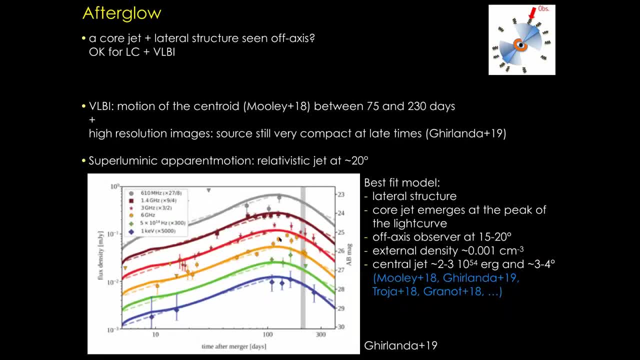 a more jet geometry scenario. so I show here an example of the best fit, including not only the light curve but also VFBI information, that we have to determine a lot of quantities. we know that we have an ultra relativistic, ultra energetic jet. we know that we see it of axis. 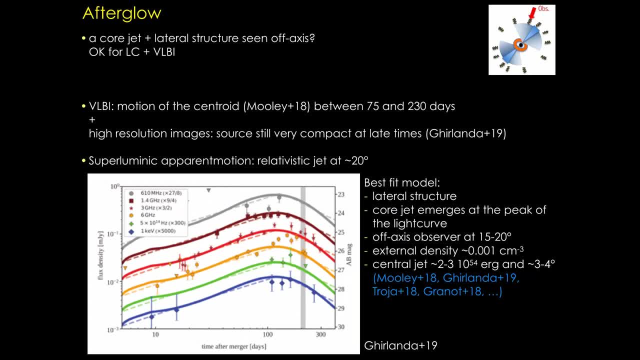 we know the opening angle of the core jet, we have an idea of the lateral structure and in this case the external medium is at a very low density. but it is expected for a neutron star merger. in this case, we know that the merger occurred in the periphery of the galaxy. 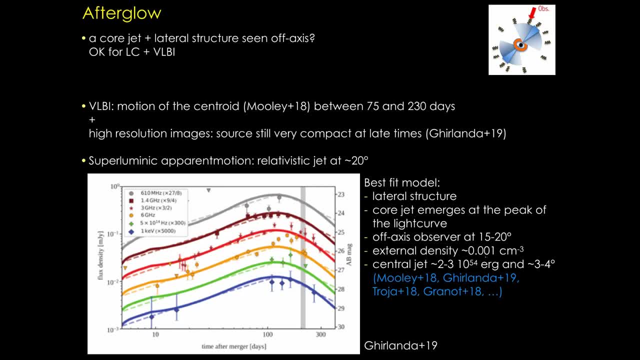 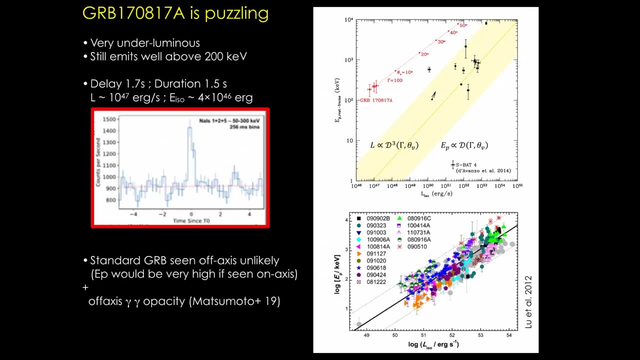 which is an lenticular galaxy, so it's very natural to have a low external density. so it's very nice because we explore this with the jet geometry for the first time, and I will skip that. and now I can say a few words about the gamma ray burst itself. 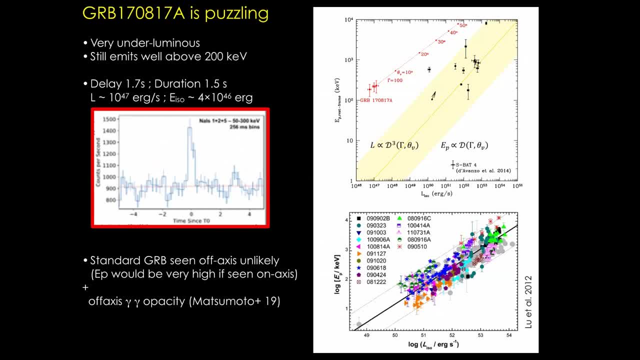 the gamma ray burst is very peculiar because it emits gamma rays above 200 kV, so it's a real gamma ray burst. but we know the distance- 40 MPa- and the gamma ray burst is extremely faint and we can see that it emits an isotropic equivalent energy. 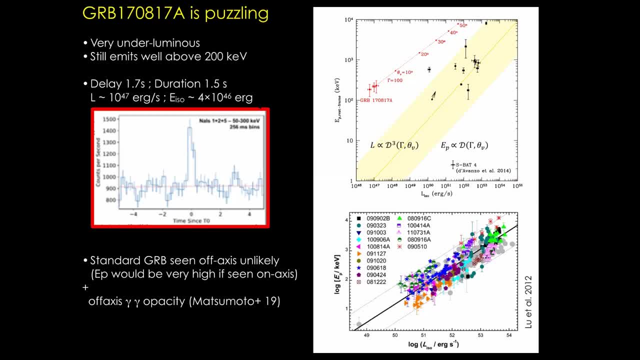 of a few tens to 46 Hz, so several orders of magnitude below normal gamma ray burst. here I show a plot with peak energy versus gamma ray luminosity, with a sample of short gamma ray burst and in yellow the typical region where they are observed. and here another such sample. 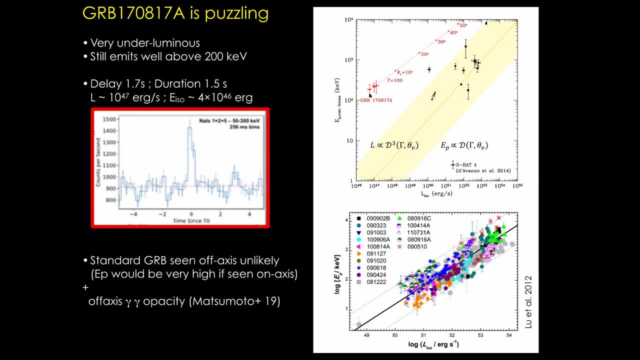 with a typical region, and here I show the location of the gamma ray burst. you could say it's much fainter and much weaker than normal gamma ray burst, just because it is produced by the core jet and the core jet is seen off axis. but there are several problems. 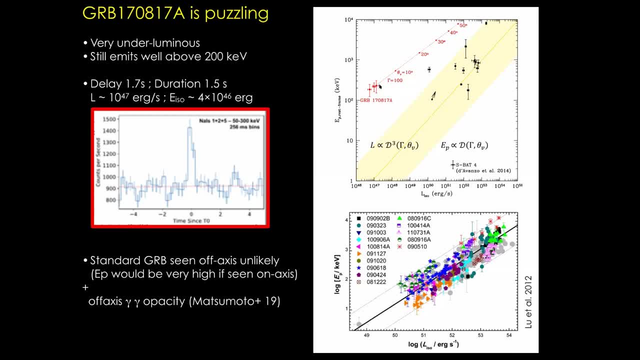 with this explanation. first, if you compute, where would be the same gamma ray burst in this off axis interpretation, assuming that you see it at another angle, you would move along this line and you would never enter this region where standard gamma ray bursts are, so it would remain a non-standard gamma ray burst. 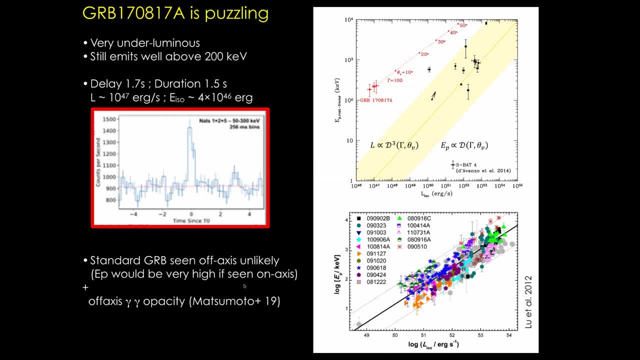 and, in addition, using the gamma gamma opacity criterion I discussed yesterday, Matsumoto and collaborators have shown that when computing accurately this opacity for an off axis observer, in fact gamma rays from the core jet cannot escape. so gamma rays cannot come from the core jet, they have to be produced. 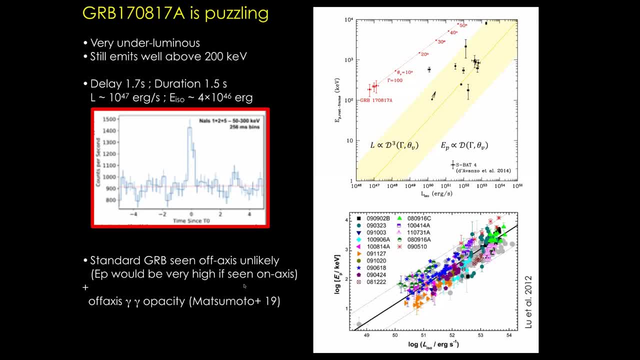 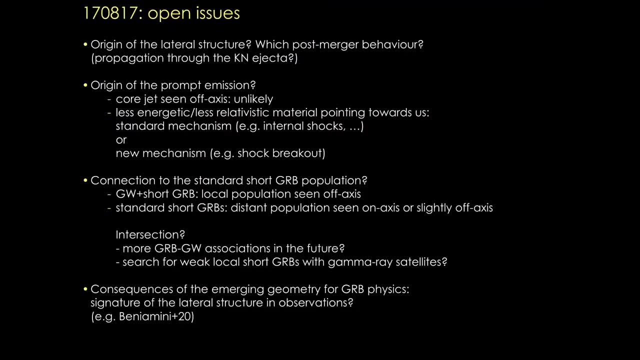 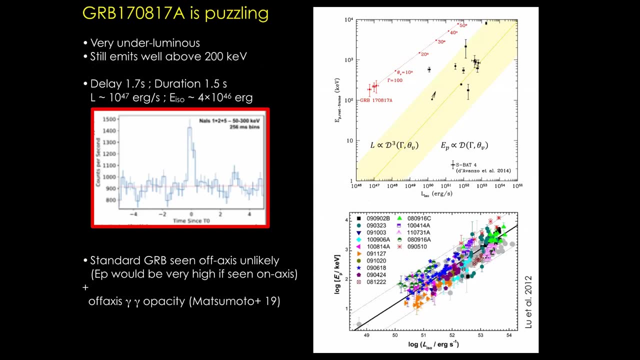 by the material coming towards us, so by the lateral structure, and then it leads to many questions about the processes in this structure. it asks the question to know if it's a new mechanism or if standard mechanisms like internal shocks can work in this lateral structure, which is less relativistic and less energetic. 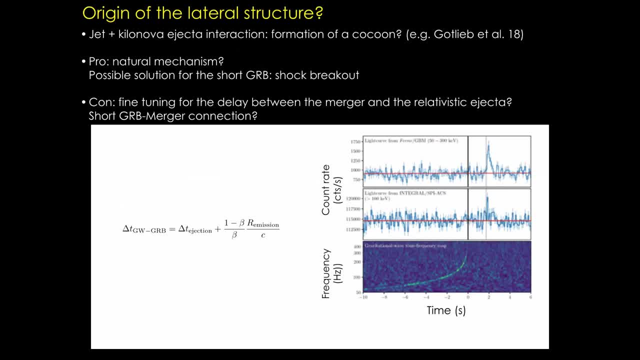 another question which is very important is the question of the delay which is observed between a gravitational wave here on the bottom and the short gamma ray burst on the top. you can expect two origins for this delay: a delay between the relativistic ejection and the merger. 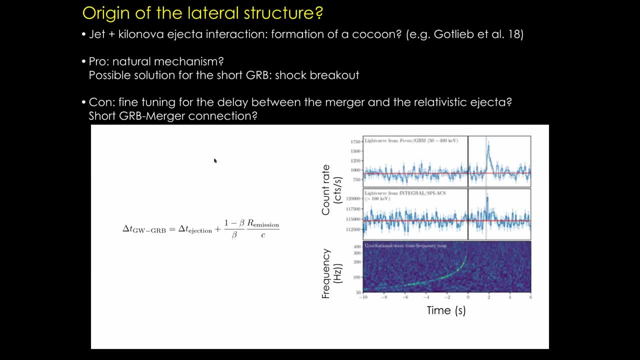 and then a delay due to the relativistic propagation of the jet of light like gravitational waves. in the scenario where the short gamma ray burst would be produced by something like internal shock, for instance, you can very naturally predict a delay which is of the same order as the duration of the burst. 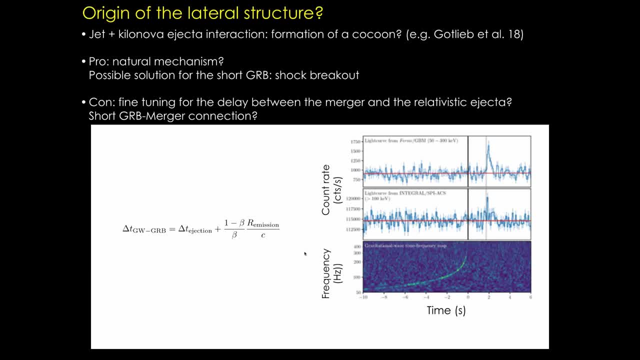 as observed in other scenarios where the mechanism is new, like, for instance, scenarios like the interaction of the relativistic jet with the kilonova ejecta, producing a shock breakout- the delay is less natural. you have to produce it by a delay between the relativistic ejecta. 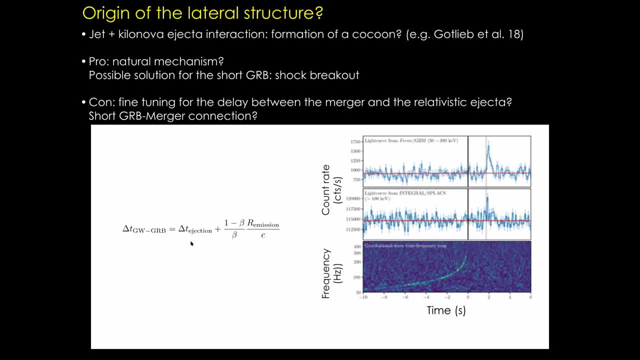 and the kilonova ejection, and so there is some fine tuning to distinguish between the two ideas. we need a larger sample and we need to study the distribution of delays, the distribution of delays and the evolution and about the mechanism responsible for the soft gamma ray burst emission. 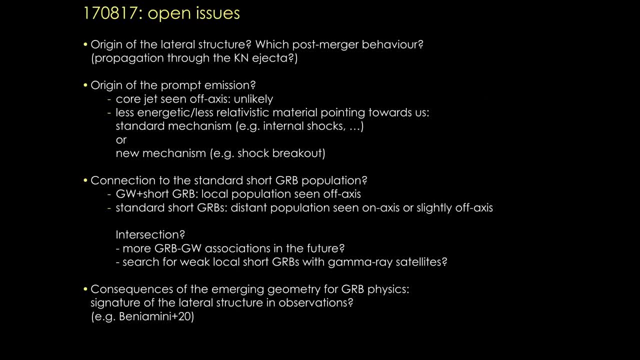 so I have listed here these questions, so questions about the origin of the prompt emission, and I will conclude by saying that with only this event we have already learnt a lot about the structure of the ejecta, and now it asks many questions about other gamma ray bursts. 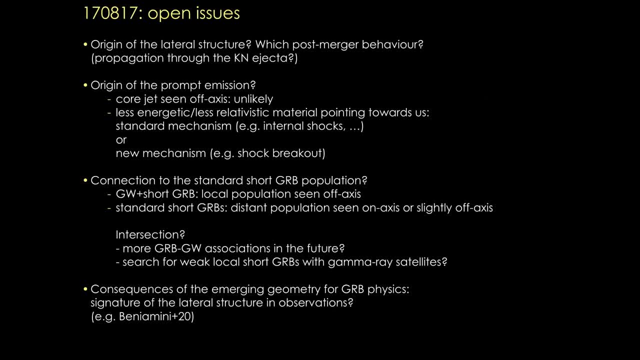 should we assume that the same lateral structure can be found in other gamma ray bursts, and then could we find a signature of this structure in other gamma ray bursts? what is very important for the future is to make the connection between the local distribution of gamma ray bursts. 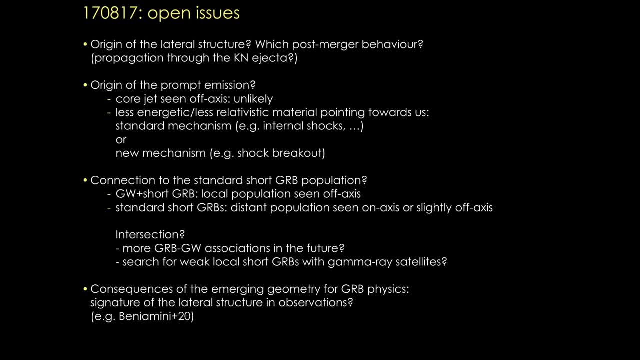 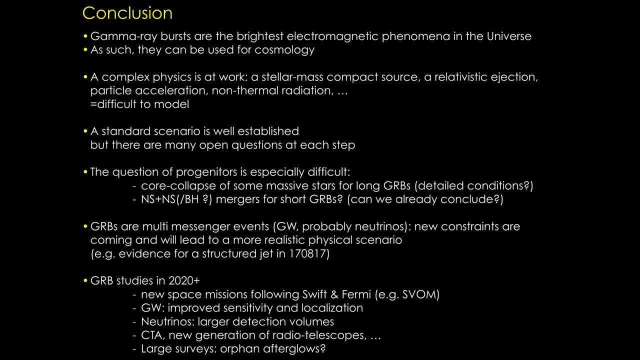 associated to gravitational waves with such weak off-axis bursts and the standard population. but for that probably we will have to wait for the next generation, because I have tried to introduce the basic concept of the physical modelling of gamma ray bursts, but I have also listed a lot of open questions. 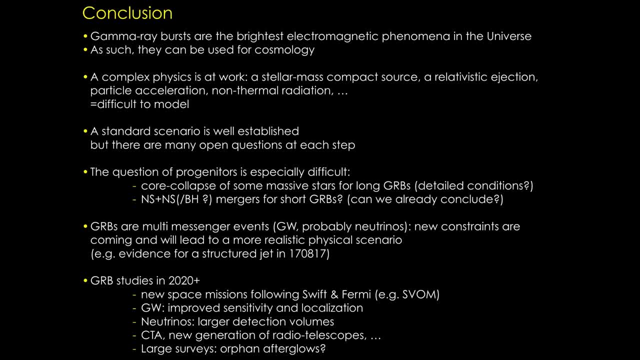 open issues. I am sure that among you and among the younger ones, there will be an interesting and important contribution to try to solve some of these open issues, and I think that gamma ray burst studies are still a very promising future because of the emergence of this multi messenger astronomy. 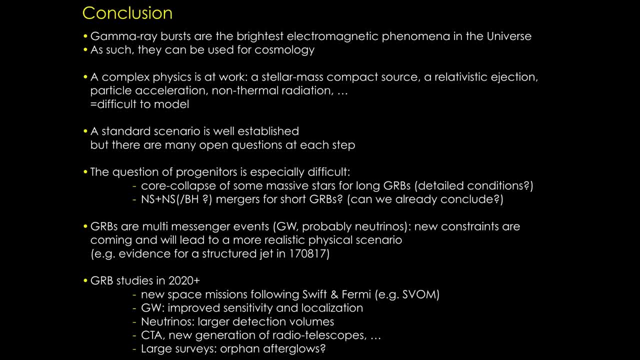 and the fact that in the future we will have even better means of looking for counterparts. we will have also a new generation of neutrino detectors which are more sensitive. we have the CTA, so I am pretty sure that the next decade will be very interesting for gamma ray bursts. 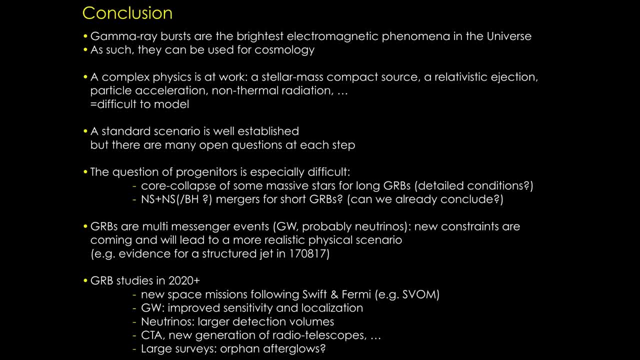 and I thank you for your attention and if you want, I can still, of course, take questions. Thank you, Frederick. Could you hear me? Yes, very well, Last time I was speaking, but I think you couldn't hear. so we will take a few questions. maybe people could raise their hands. 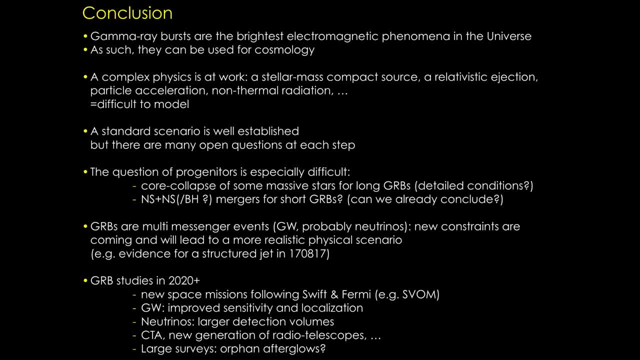 Are there no questions? I see that there is one question. There is one in the chat box. There is one in the chat box. If one or both of the components of a binary neutron star merger were a pulsar, we would have Good question. I am not an expert at all. 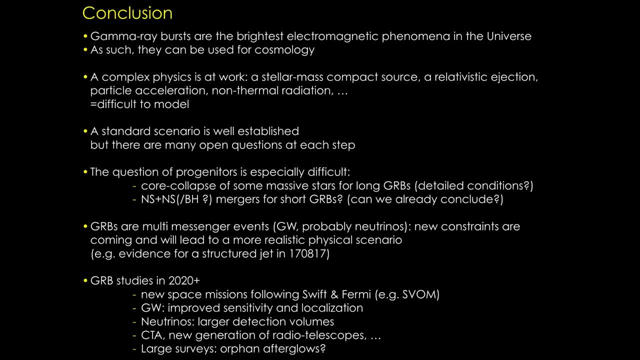 at this question. If the two are the same, then I think it is a good question. Can we expect an electromagnetic signature? and, very interestingly, could we expect an electromagnetic signature before the merger, which would be very interesting to have an electromagnetic precursor. So I am not an expert. 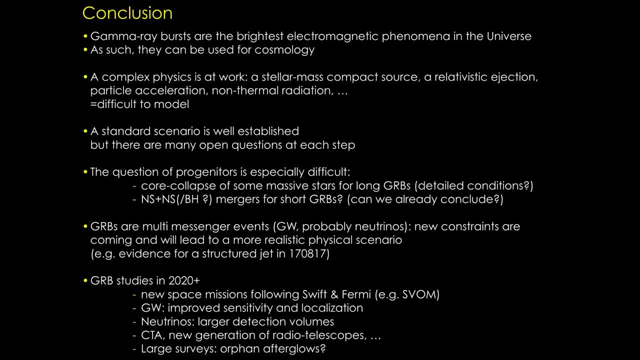 but I have in mind the fact that there is a group with Cerruti- Cerruti is someone working on a twin cell simulation coupled to a large scale simulation to study the magnetosphere of pulsars- and I have in mind the fact that they have produced. 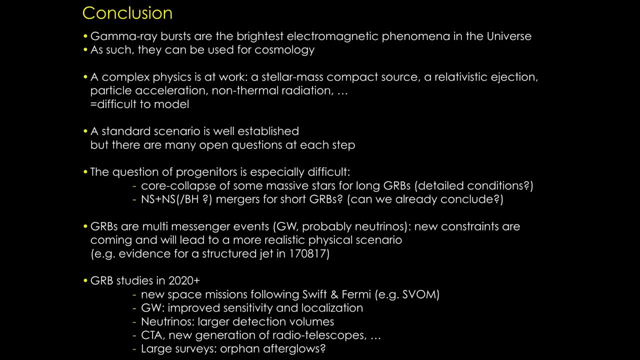 a simulation of two interacting pulsars during a merger and I think they have made some prediction for this possible electromagnetic precursor, but I don't remember very well the result. It was difficult to detect except at very small distance, but I am not completely sure it should be tested. 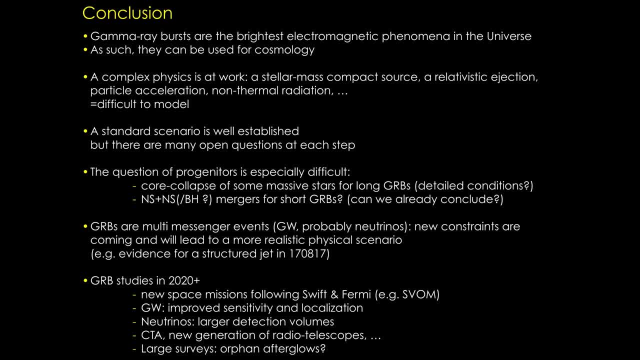 It is a very interesting question. There is some question. Is Mr Raj Patel asking a question? I see one question about 170817, about the fact that initially the optical afterglow was center than the kilonova. and it's not the case and usually the optical afterglow 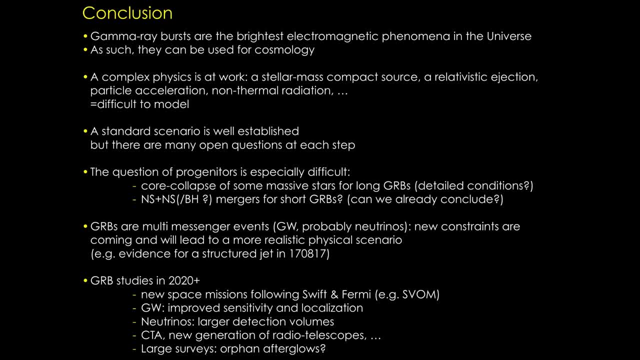 is very bright initially. Yes, it's a good question. It is a. probably I went a little too fast. This is the major difference between 170817. In standard afterglow, the flux is just decaying. Here we see a very slow rise and then a decay. 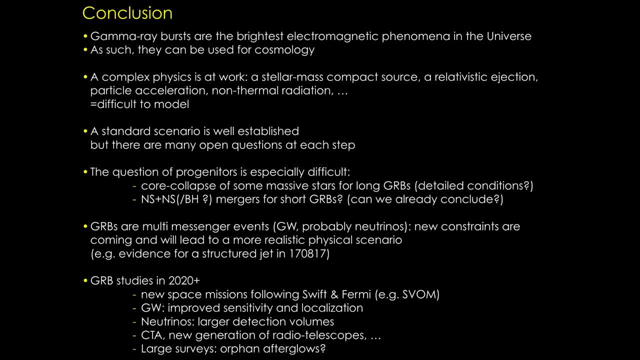 and I have tried to explain that this is due to the fact that they are really of axis. This is the main difference. So the sun burst, seen on axis, probably the optical afterglow. I should make the calculation to be completely sure. but would that be much brighter initially? 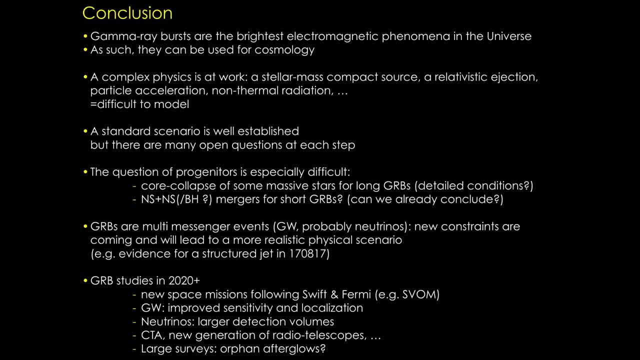 and maybe with the brightness comparable or even above, and then it would have been more difficult to distinguish both. So it's a good point is that the probability to observe in the near future a local burst on axis is very low. We see a lot of on axis burst at large distance. because the universe is very large, but at the scale of one galaxy it's very, very dense and when we are limited to the local universe we do not see as many galaxies. We have time for one or two more questions, Questions. Okay, There is one question about elaborating. 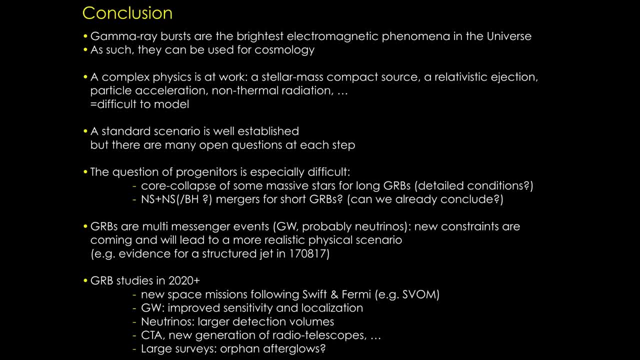 about the effect of spin down, in short GRBs. I must say I am not an expert on this topic so I will have difficulties to be very detailed. The idea- I would say that very generally- the idea is that if there is a long-lived neutron star in the 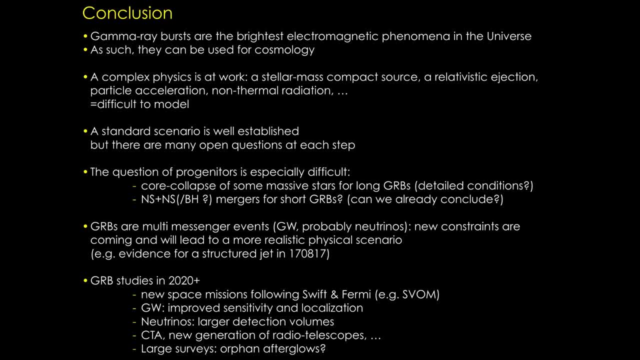 central source. I would say that a very general question that is not clearly answered yet is: what are the mechanisms for the relativistic ejection and how can you produce all the usual phenomena? It's not so simple to produce such a collimated, highly relativistic outflow. 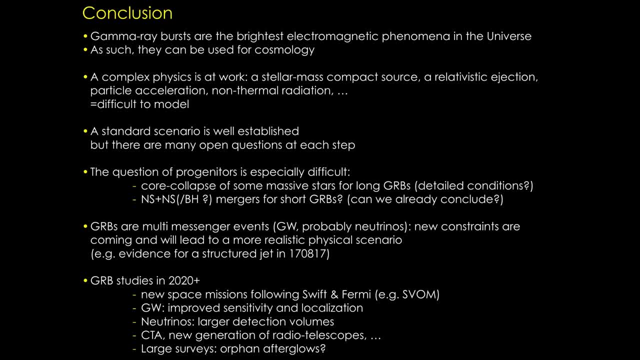 in a neutron star. If it's more a situation where you have an intermediate phase with a neutron star and then it collapses to a black hole, then it's interesting to know if we should look for a signature of the neutron star somewhere, and the idea is that 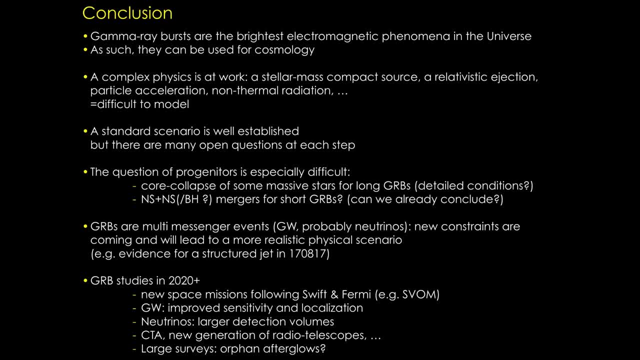 a neutron star has a well-known spin down luminosity- the standard pulsar theory, and. but in a standard pulsar it's producing a pulsed emission which is picking maybe somewhere in X-rays or gamma rays, but also with a strong component in radio, etc. this is a standard. 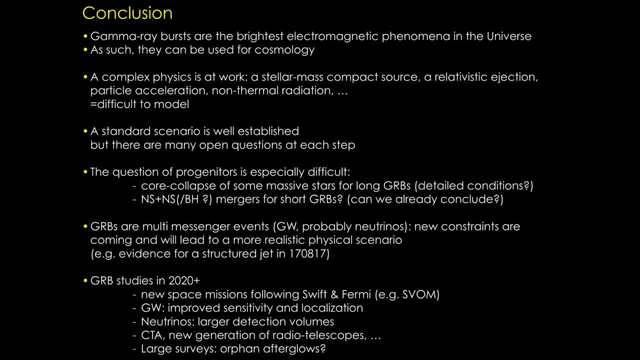 The idea is that to apply that to gamma-ray burst theory and to, for instance, to try to explain some features observed in some gamma-ray bursts, like plateaus or things like that, you really need to explain how a certain fraction of the spin down luminosity of the pulsar is converted. 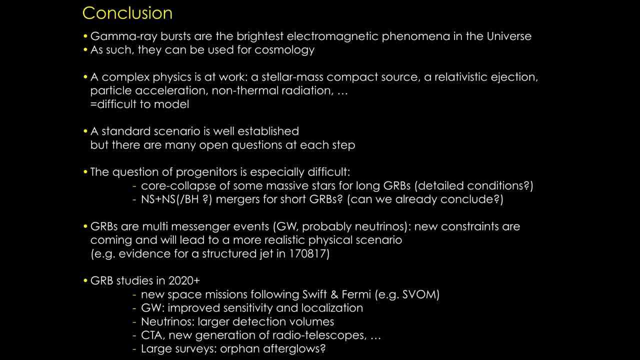 into radiation and what is the spectrum of this radiation? and, for instance, most signatures which are discussed in the literature are in X-rays. so how does it pick in X-rays? for instance, plateaus usually are not observed, so it's a very big component. so these are 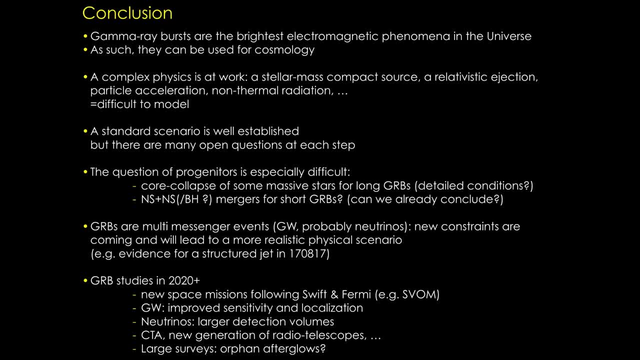 the kind of questions that should be answered. maybe one last question. ok, so I assume there is no more questions. that is it, then. let's thank Frederic for this wonderful set of lectures. I must particularly extend a special thanks, because many of the young members from my Pan-Indian GRB group 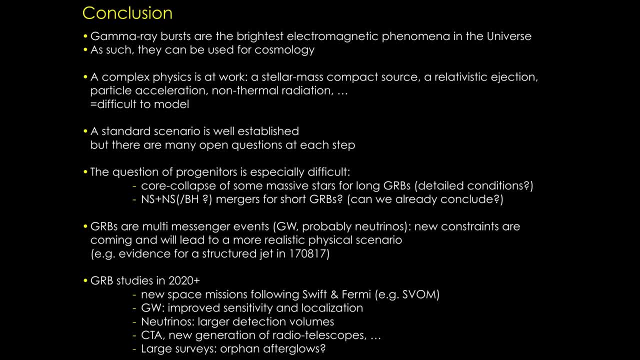 has greatly benefited from this also. thank you on behalf of the organizers and the remaining participants. let's give a big thanks in the zoom way. maybe, I guess, we could give it a clap reaction, all of us, or?